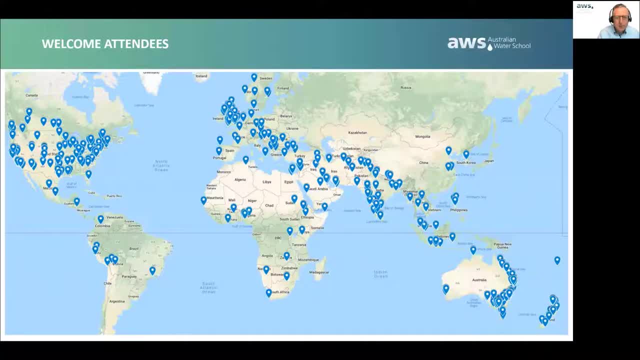 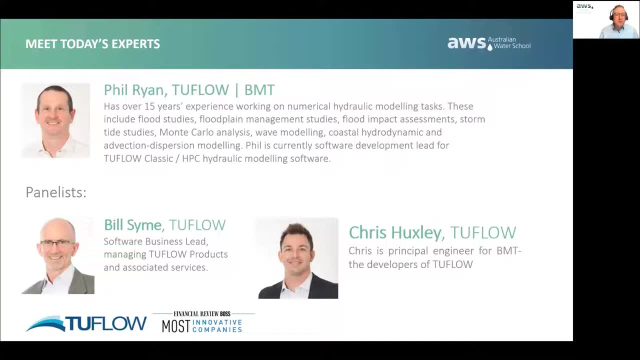 Look at that. spread across the globe: over 1,000 registrants spread right across from Australia through to the US, everywhere in between Europe, Africa, Southern America as well. Let's get into this. Phil, Bill, Chris, come on screen. Let's see what you look like. 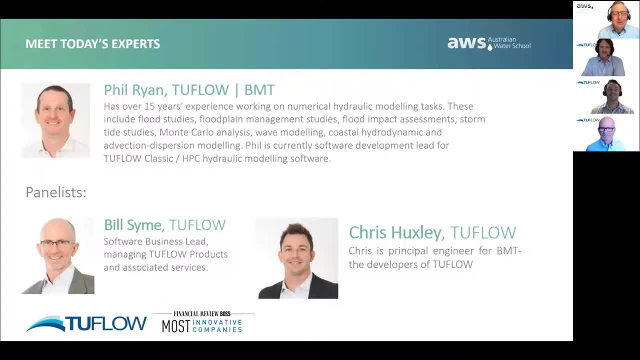 Phil Ryan. Phil Ryan, from TuFlo, has had over 15 years experience working on numerical hydraulic modelling tasks. These include floodplain management studies, flood impact assessments, storm tide studies, Monte Carlo analysis, wave modelling, coastal hydrodynamic advection dispersion modelling. 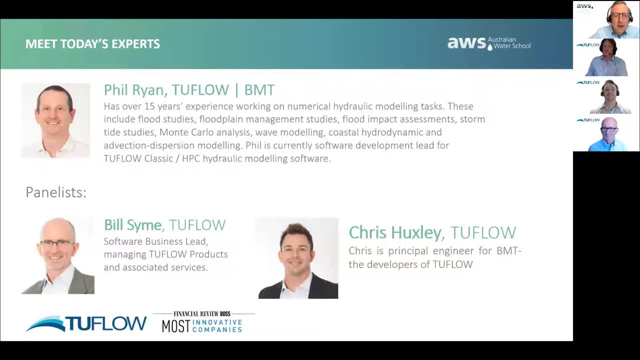 Phil is currently software development lead for TuFlo Classic, a HPC hydraulic modelling software. Bill Syme is also from TuFlo software business lead managing TuFlo products and associated services, And Chris Huxley from TuFlo is the principal engineer for BMT. 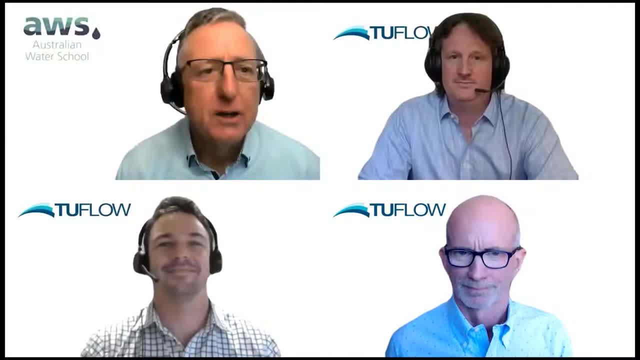 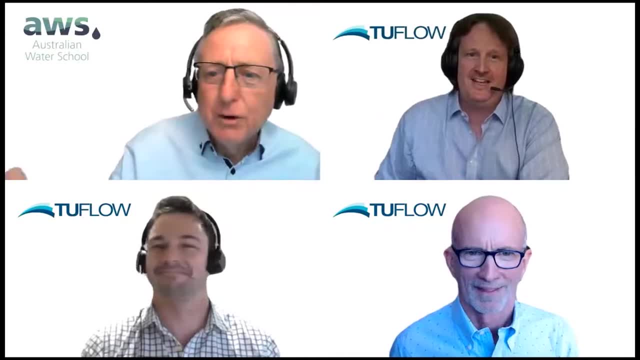 The business manager for BMT. The business manager for BMT. So we're so delighted to have you gentlemen with us, And I thought you were all Queenslanders in the wonderful Australian state of Queensland, but that is not the case today. Chris, you're from Queensland, in Queensland, in the capital of the city of Brisbane. 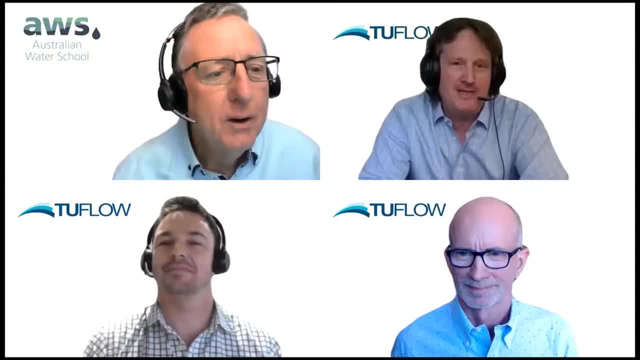 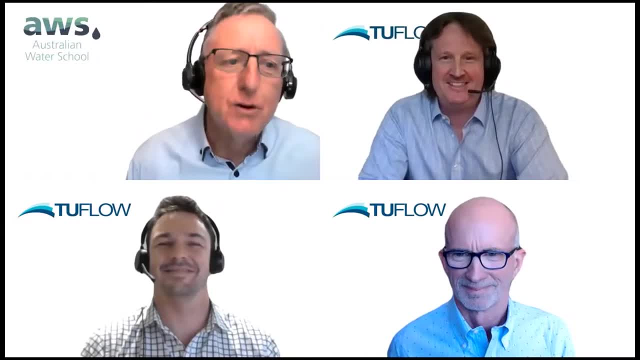 And Phil, you're not. I understand. No, I'm actually in northern New South Wales, in Bangalow, which is a town inland of Byron Bay. Make that distinction. You're not a Queenslander, I mean in Australia. this is very important. 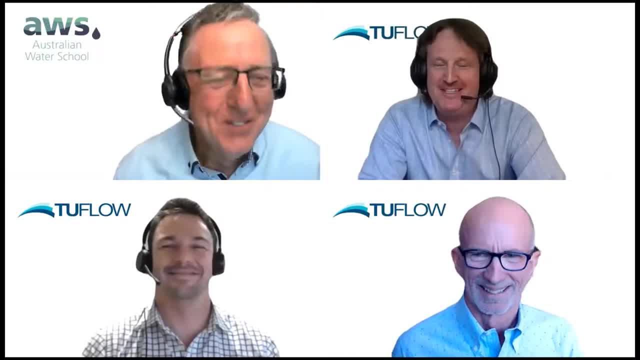 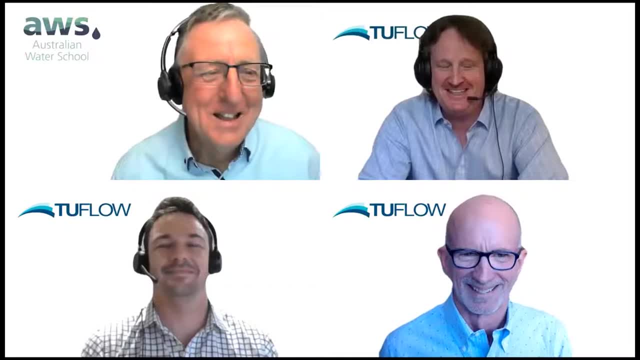 Well, I actually do follow Queensland in the state of origin. I did, But my career at BMT in Brisbane, So I don't know if that's what makes me a Queenslander or not. I think it might be. I think you'd be on that one. 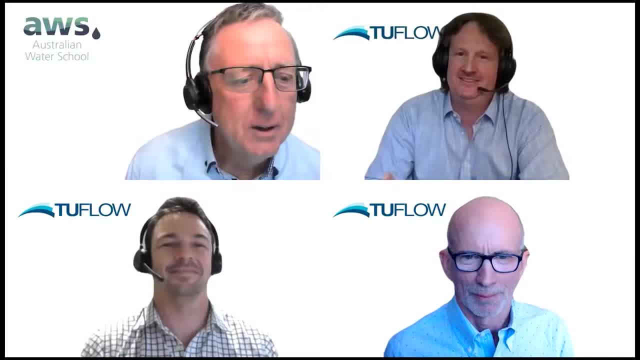 And Bill, you are a Queenslander but not up there today. Oh, I'm down in Hobart, Hobart, down in the wonderful Tasmania, In Tasmania, yeah, So great to have you. We're right up to you, Phil, in your hands now. 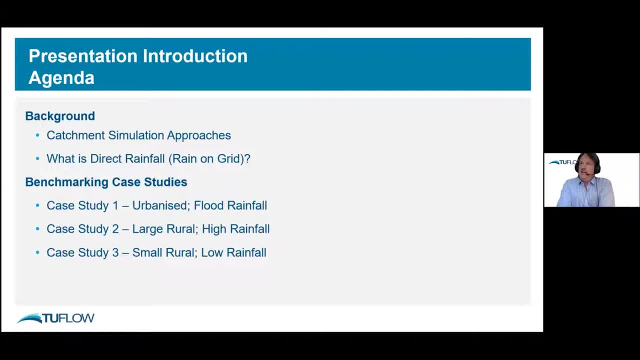 Thank you. Well, we'll take it away then. So yeah, in terms of today, what we wanted to go through is a little bit of background on different catchment simulation approaches and what is direct rainfall, And I guess, at this very early stage, I think there's. 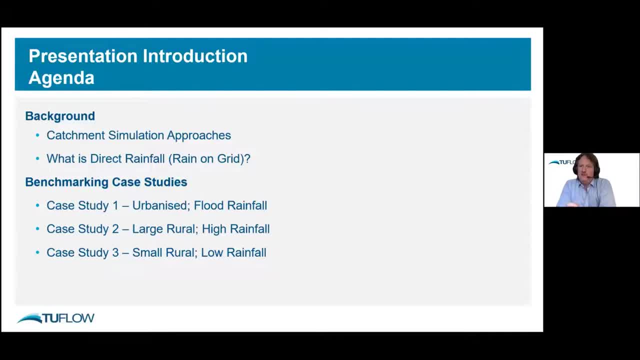 Direct rainfall and rain on grid- conflicting terminologies for the same thing really what we're talking about today. I had a look in AR&R, which largely the Australian rainfall and runoff guideline, which is our Bible here in Australia, which really adopts the terminology direct rainfall rather than rain on grid. 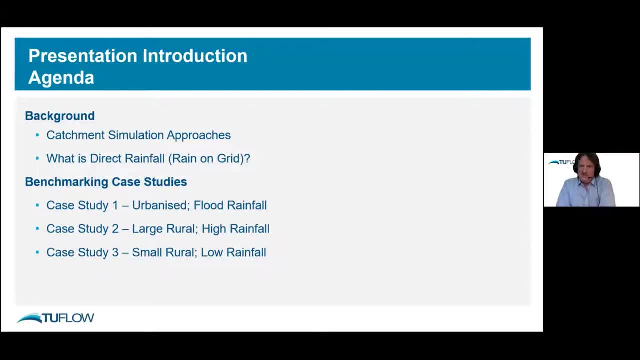 So I'm going to stick with direct rainfall throughout this presentation. But you know, I do understand that in other parts of the world, probably particularly the US, that rain on grid is more widely used. Just to be clear, we're referring to the same thing. 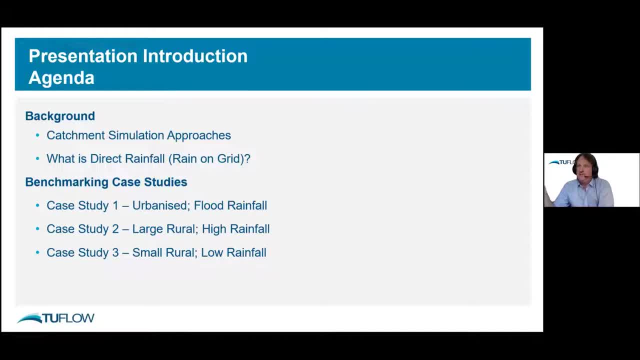 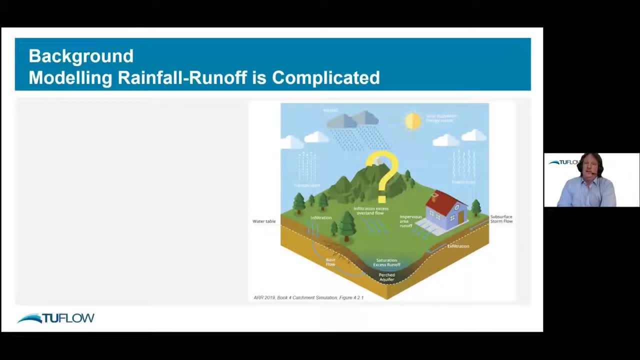 It's just a slightly different terminology, So we'll go into what it is And then we'll jump into A number of different case studies of quite different catchments and also rainfall events as well. So what we're really talking about here is the options for converting rainfall into runoff. 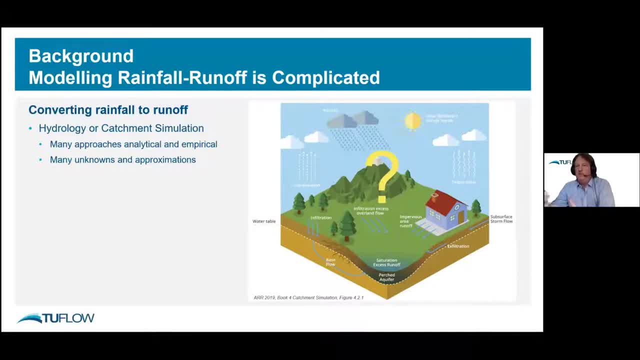 So traditionally probably a two stage process has been used. A rainfall runoff model has been used to generate flows which then go into a hydraulic model for routing those flows. So I guess typically the hydrology or catchment model uses an analytical or empirical approach. 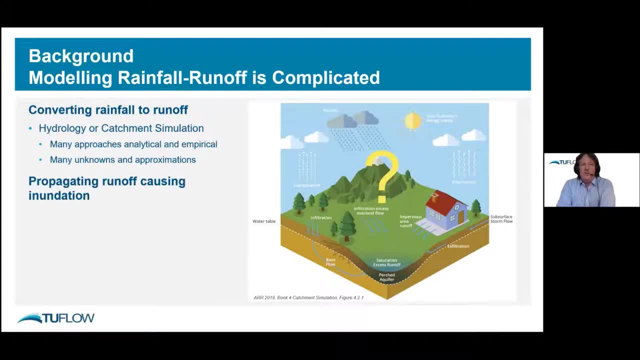 And there's there's some unknowns and approximations, As with all modeling. however, once we get into the hydraulic modeling, we're starting to talk about more a physics based solution of fluid flow, not saying that there's not uncertainties, but it's moving into that more hydraulic, physical equations. 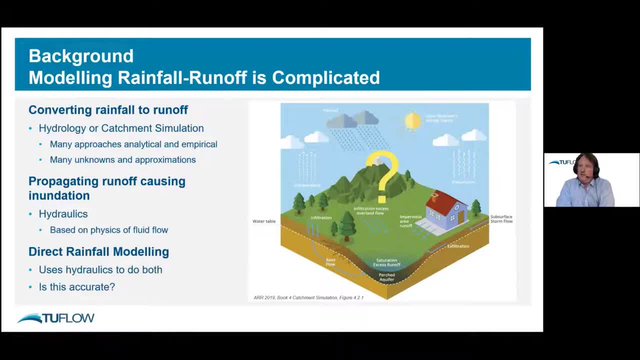 So direct rainfall modeling is is really using that hydraulic model to do both of those- the rainfall runoff generation and then also the routing of that flows. And I guess that the key question there is: is it accurate? And that's hopefully what we're looking to discuss a bit today. 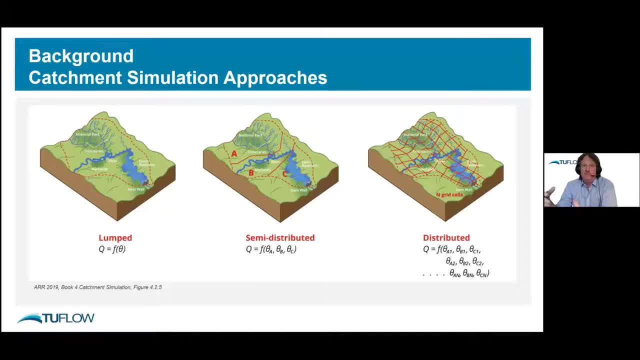 So, in terms of background, in terms of those catchments, Simulation approaches, there are a number of ways of doing that: A lumped approach, where you're basically lumping a catchment into the properties of that catchment, into a, into a single catchment and applying an equation there to generate flows coming out of that catchment. 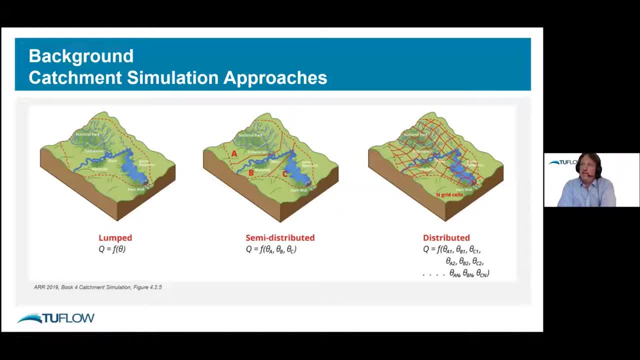 Going across to the right, we've got a semi distributed catchment. So we're breaking that catchment down into a number of sub catchments, generating those rainfall runoffs at that sub catchment level. And then, as we move further to the right, we're looking at a distributed model which is breaking it down into into a- not into subcatchments. 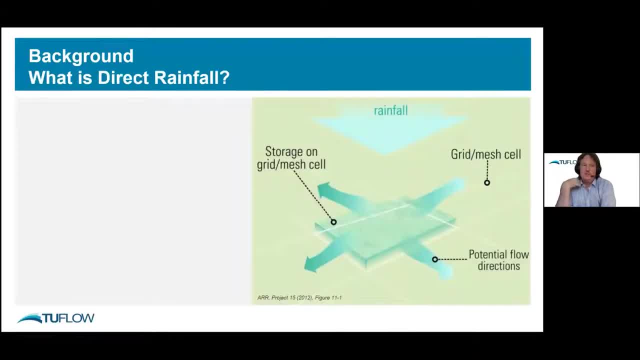 But into a range of smaller, smaller units, which is which is really the direct rainfall is moving across that way. So in direct rainfall, what we're doing is we're applying a rainfall depth to each of the 2D cell or mesh elements in the model, which one of the reasons I probably use rain- direct rainfall rather than rain on grid, because it doesn't just apply to the grid based models. 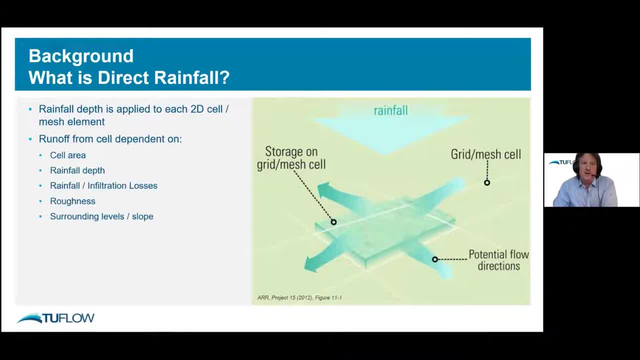 It also does apply to to mesh based models as well. So each of those cells or mesh elements gets the rainfall directly applied to it And the amount of rainfall Runoff from that cell is therefore dependent on the cell area and the rainfall depth, obviously, but then also the hydraulic parameters, you know, any rainfall infiltration losses that are being applied, hydraulic roughness and also the surrounding levels and slope in the surrounding cells. 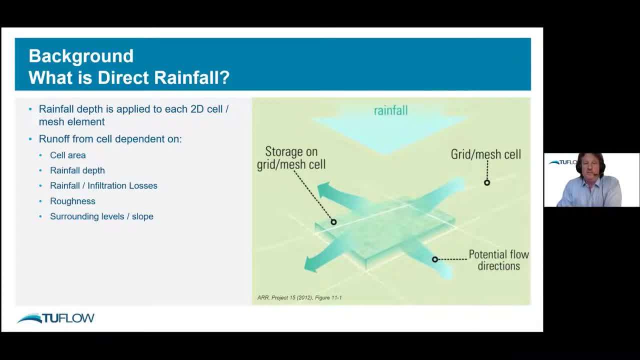 So there's a potential for for water to move in more directions, as opposed to a traditional hydrology model where you're generally routing that flow in a in a single, predefined, defined direction with a direct rainfall modeling. you're letting the 2D cells 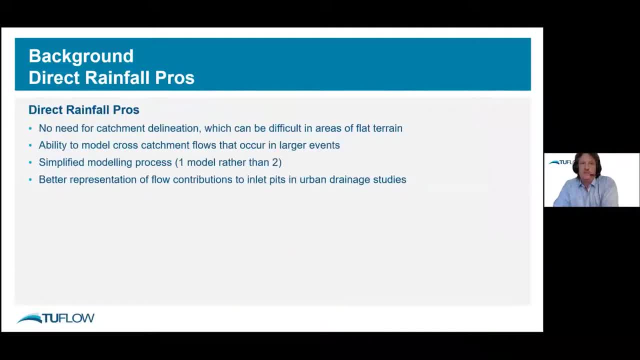 Decide where that water should be going at the current time step, which does have some some advantages. There's no need for a catchment delineation, which can be a little bit difficult in areas of a flat train, So you don't have to pre process that elevation model into a series of sub catchments. You actually just feed the elevation model into the software. 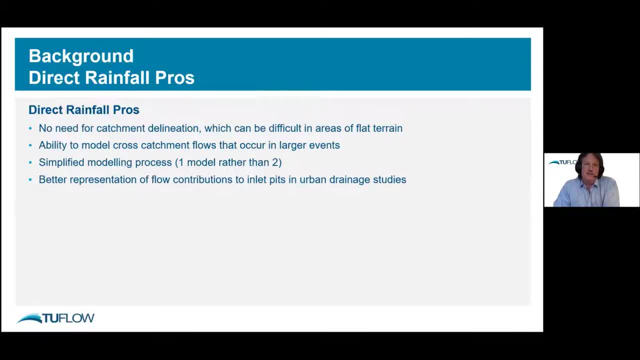 And it also gives us the ability to model cross catchment flows that can occur in in larger events. So the flow paths in smaller events may not be the same as the flow paths in larger events and a hydraulic model- And nearly everywhere, in the end it will just definitely capture that. 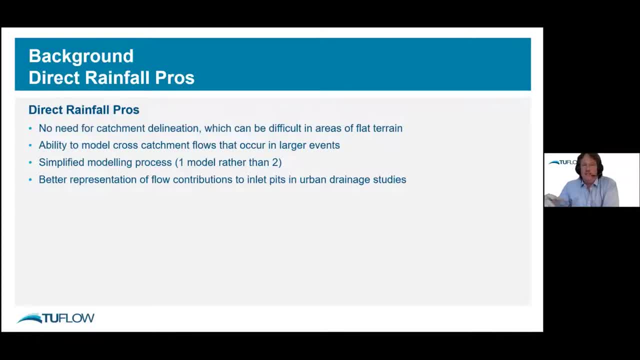 And it does give us a simpler modeling process. So we've got one model rather than d models there and particularly as we're getting into urban drainage, high resolution of an drainage- it's probably giving us a better representation of of flow contributions to individual. you know, pitets or in that, gullies, in that the water's going onto this 3D cells and making its way, you're not having to pre define the catchment area upstream of each. 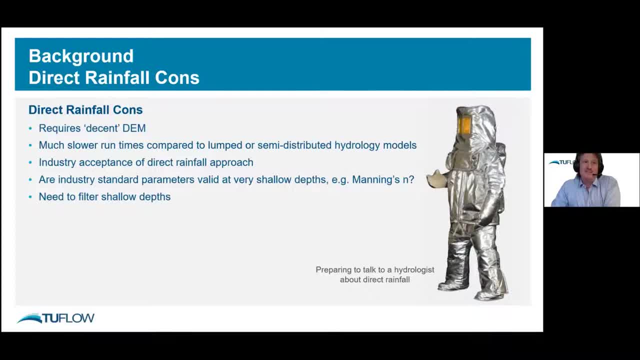 Each individual pit in order to get that right amount of water coming into there. Naturally, there there are cons. cons to everything, The direct rainfall probably are. you do require to have a decent DEM that covers the entire area that you're looking to apply the direct rainfall to. Typically, that would probably be done for a 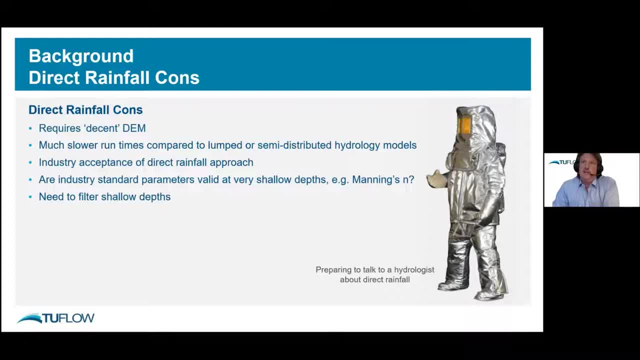 whole catchment, So you'd use direct rainfall over your entire catchment area. It is possible, obviously, to mix and match, So you've got a hydrology inflow in certain tributaries and then apply direct rainfall just to a portion of the 2D model. Obviously, we're solving more, and that. 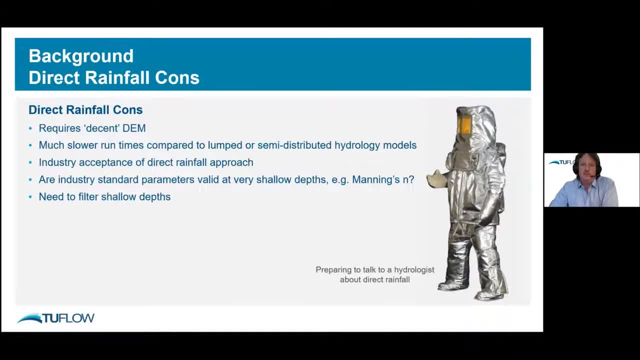 gives us slower run times compared to a lumped or a semi-distributed hydrology model. Industry acceptance of direct rainfall. There is, in different parts, a bit of resistance to direct rainfall modelling, So there's a picture of me, all geared up in my flameproof suit, talking to a 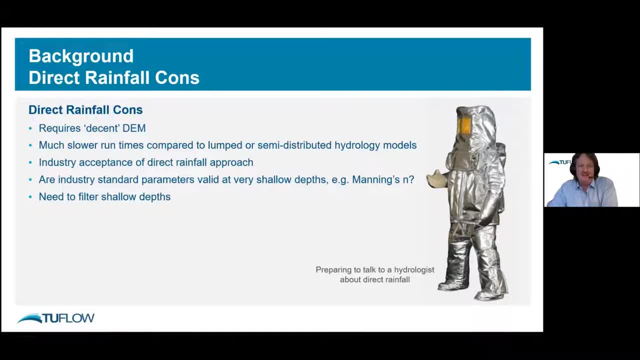 hydrologist about direct rainfall. Yeah, I think there was a fair chunk of no's in that poll question on is it accurate? So, yeah, there is a little bit of resistance to it in the industry And I guess a part of that is: you know, are those industry standard parameters that we use? 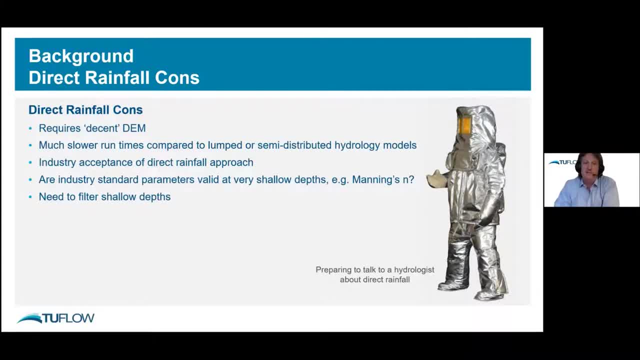 for calibrating hydraulic models, Manning's ends and things like that. are they applicable at the very shallow depths that are encountered in direct rainfall modelling? And the last one: there is a need to filter those shallow depths out, Because you're applying rainfall directly to every cell. 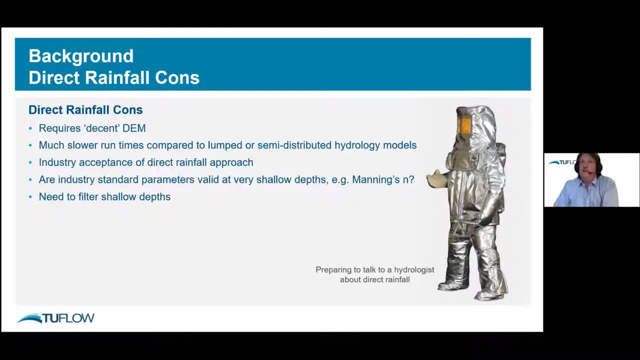 in your model, all of the cells are therefore wet and flowing, So it's up to you, as a modeller, to work out what type of cutoff you should be using in terms of where you're mapping what's wet and what's not, what's flooded. 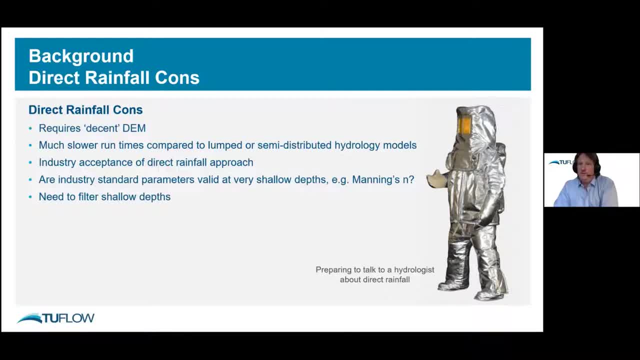 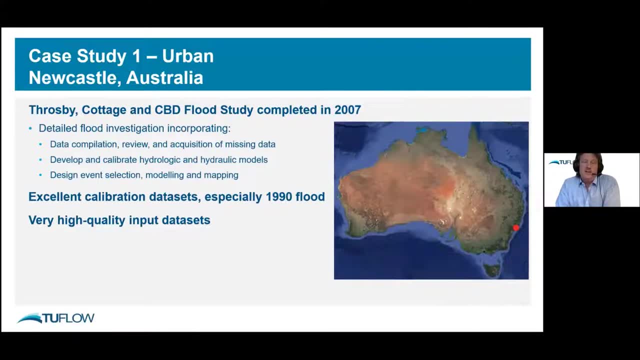 Or what's just that really shallow direct rainfall being applied. I guess that's an introduction of what direct rainfall is and how it compares to the more traditional approaches. So I'll jump straight into a number of case studies, The first one of which is the Frosby Cottage Creek in 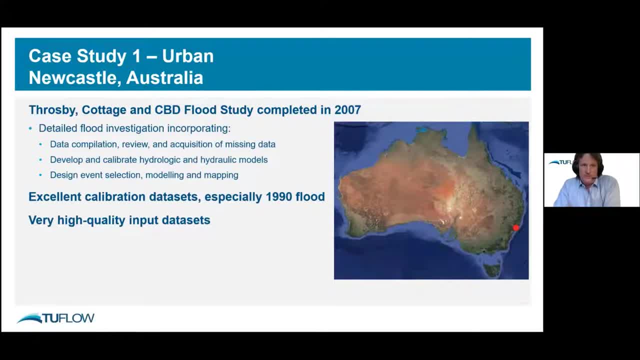 Newcastle in Australia, And this is actually a study that we at BMT did the flood study for in 2007.. We sort of wound it up- And Bill is here with me And I actually worked on that as consulting engineers- And it was a detailed flood investigation using the standard- the New South Wales Flood Management Guidelines. So data 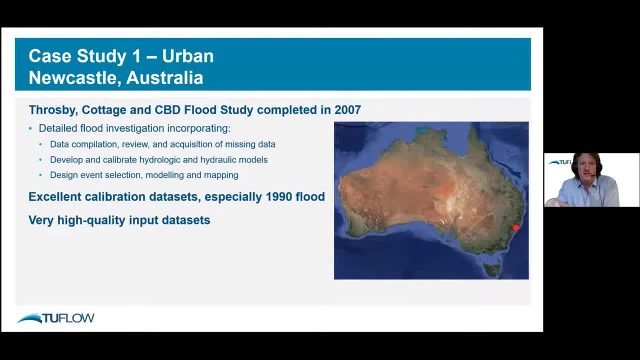 compilation and review And we basically developed and calibrated both hydrologic and hydrologic models And then running the range of design events and mapping and things like that. What was notable about that is is it had a really good calibration dataset, especially for the 1990 flood, And it also had really good input datasets. So when we started looking at models to benchmark the site and the 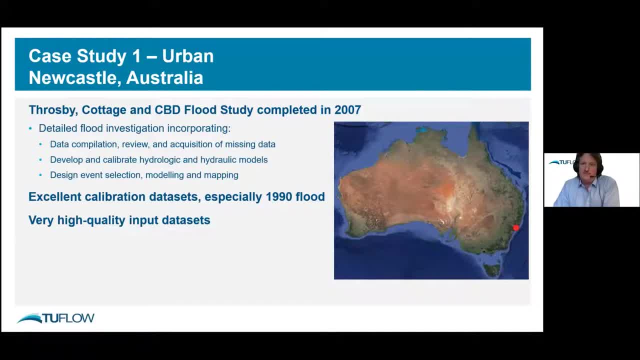 what was notable about that is is it had a really good calibration dataset, especially for the 1990 flood, And it also had really good input datasets. So when we started models to benchmark, that one sort of jumped back to us, you know, as having a good data set to look. 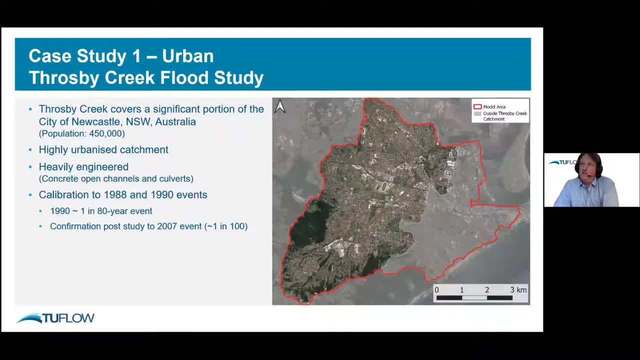 at. So a little bit about the catchment. The Throsby Creek covers a significant portion of the city of Newcastle in Australia, as opposed to the Newcastle in the UK, which has a population of about 450,000. And you can see from the aerial imagery in the right there it's a highly urbanised. 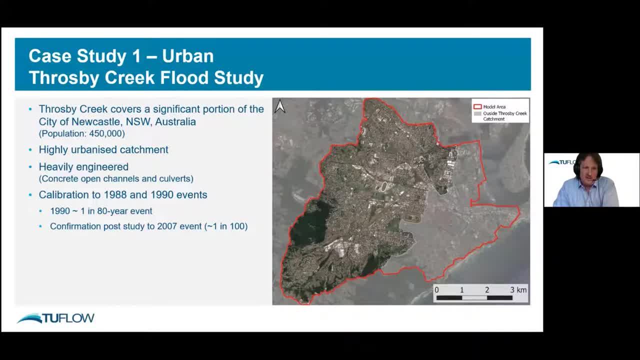 catchment and it's quite heavily engineered as well. So most of the main channels are concrete, trapezoidal, or, you know, rectangular channels with large numbers of coals in it. And so, as part of that flood study, we calibrated to two events, 1988 and 1990,. 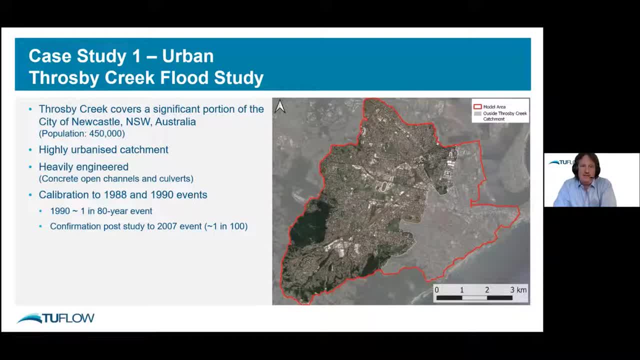 of which the 1990 was the larger event which came out at about a one in 80 year event And actually, following our study, there was another event in 2007, which was also a bit larger as well. Looking at the data that we had available for there, it's a really nice. 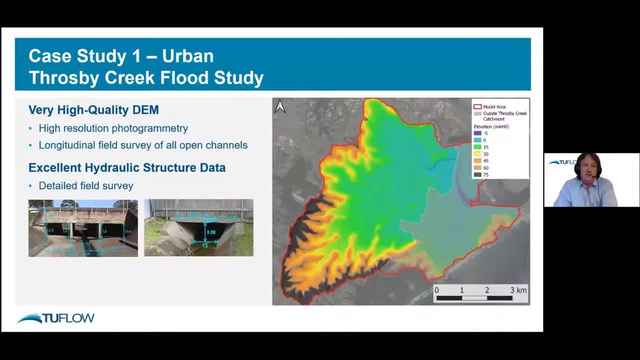 DEM for that. So I'm going to go ahead and show you that. So I'm going to go ahead and show you that. So it was a high resolution photogrammetry and stamped into that. the field surveyors went and took longitudinal survey along all those open channels, so centre lines and the 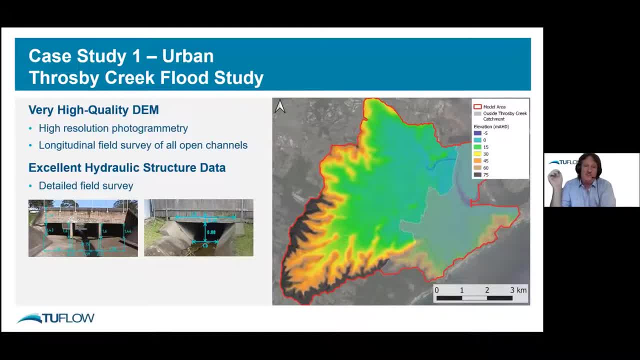 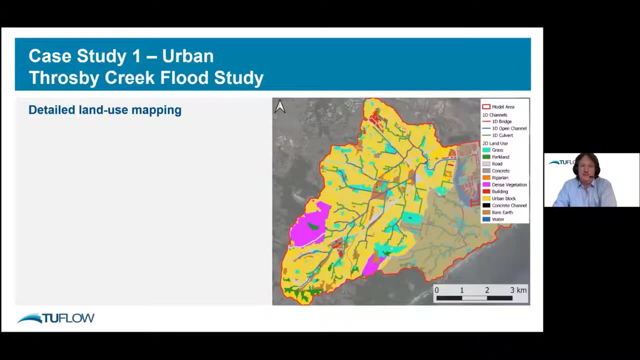 toe of the trapezoidal channels and things like that. So we had really high resolution data in the channels as well as for the structures as well, And that's an example of what the DEM looks like in those concrete channels And detailed land use mapping as well. 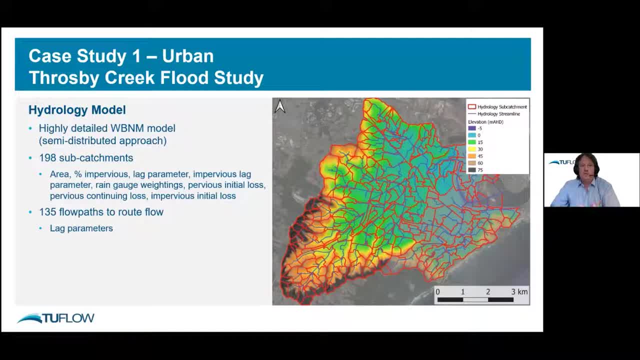 So, as part of that study, what we did was create a hydrology model. So this is work that was done back in pre-2007.. And it was a detailed WBNM model, which is one of the hydrology model packages used here. 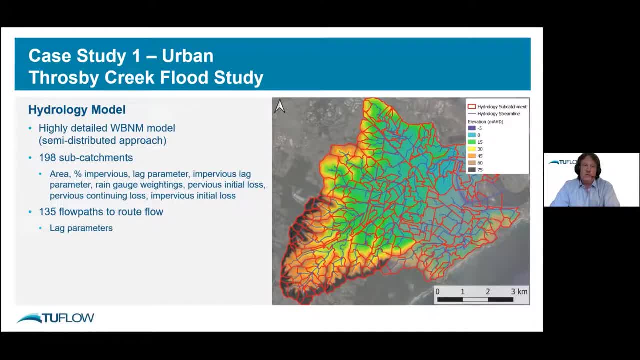 in Australia, which is a semi-distributed approach, where we broke that catchment down into 198, so almost 200 sub-catchments, for which each of those were applying the typical hydrology parameters: catchment area, percentage: impervious. some lag parameters and things. 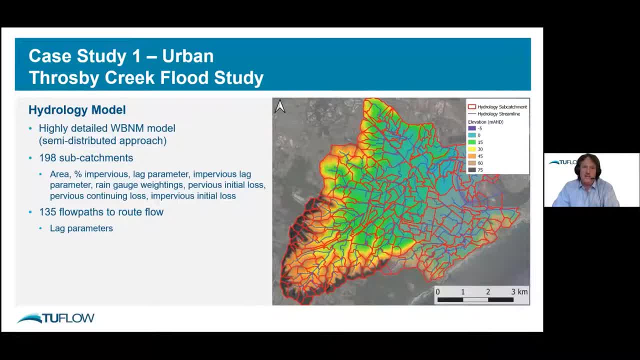 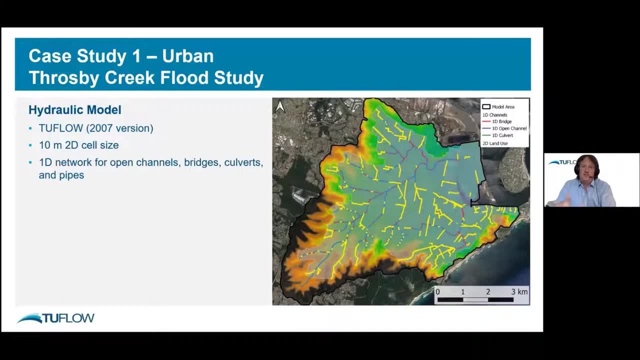 like that And there's a lot of work going on there, So I'm going to go ahead and show you a little bit more of that. And there's 135 different flow paths in there to route that through the hydrologic model. So jumping back to the hydraulic model, So two-stage modeling process originally. So we're using 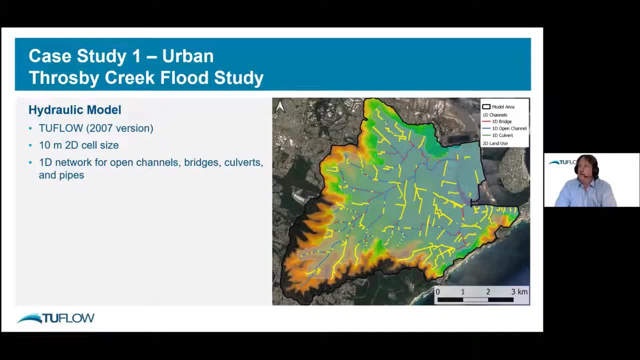 two-flow for the hydraulic modeling with a 10-meter cell size, And so the grayed area on the map there is our 2D area. The various line work is our open channels for bridges and culverts and pipes. So this was done with a 1D- 2D coupled model. 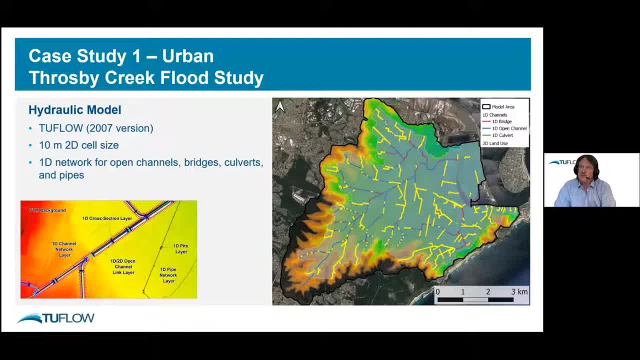 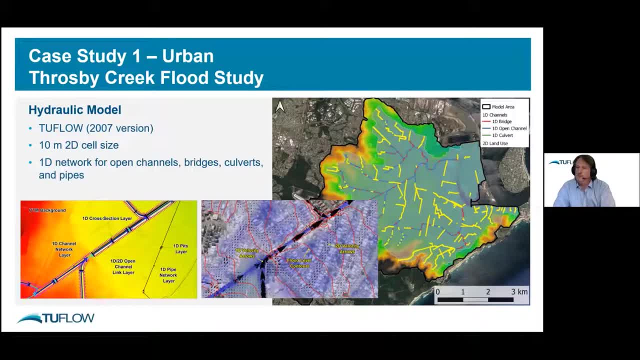 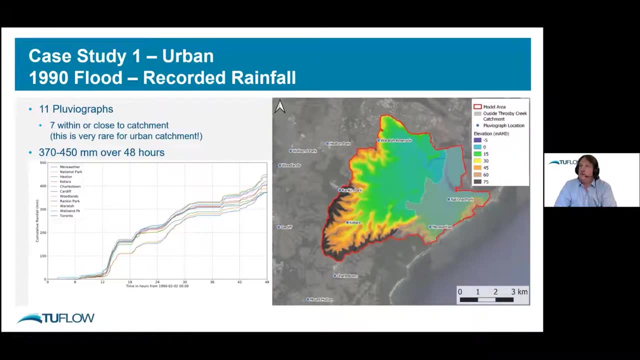 So 1D- open channels- and, as shown there on the bottom of the screen, linking to the 2D for the overbank areas, And that's an example of some of our mapping output for that study. In terms of the data available, there's actually 11 pluvia graphs recorded that recorded the 1990 flood. 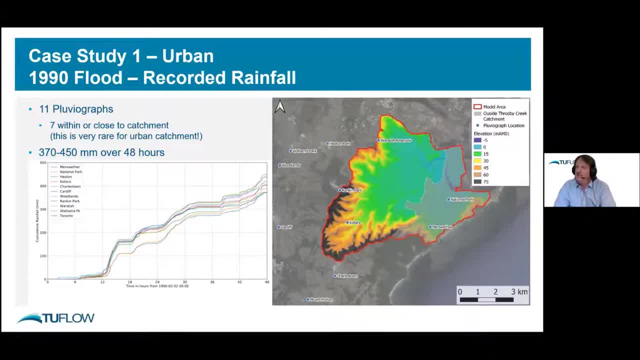 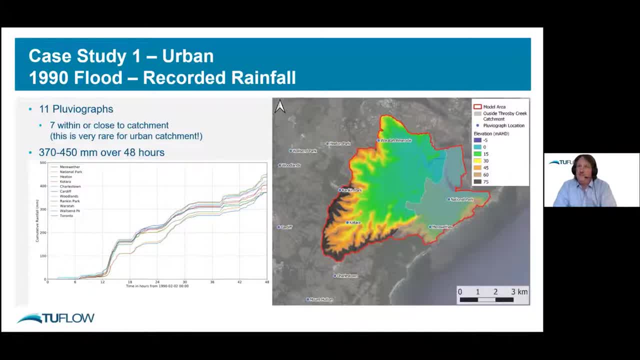 Which is sometimes the case with gauges, Which is sometimes the case with gauges. They give out when you need the most. But it's still a good coverage of pluvia graphs And we can see there that the rainfall for the event. 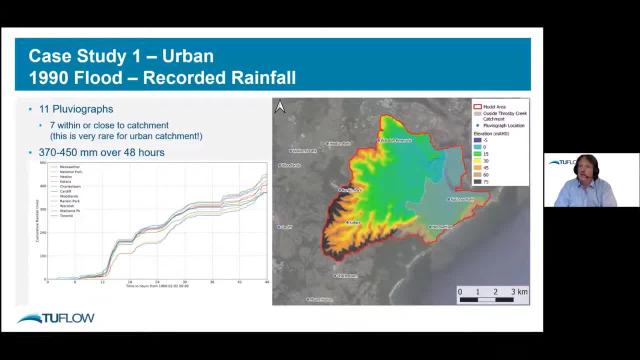 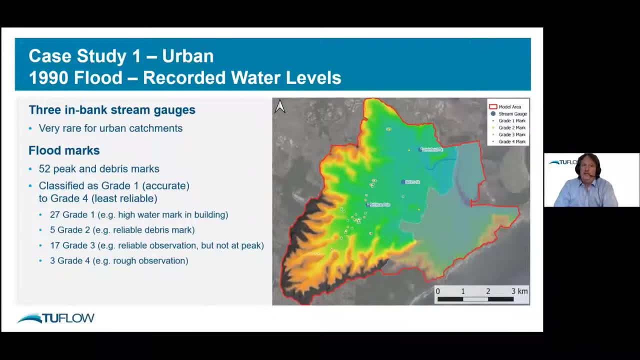 We're talking about 370 to 450 millimeters over a couple of days, And most of that actually falling in the later 36 hours, So it's quite a significant rainfall event And three inbank stream gauges as shown there on the map as blue dots. 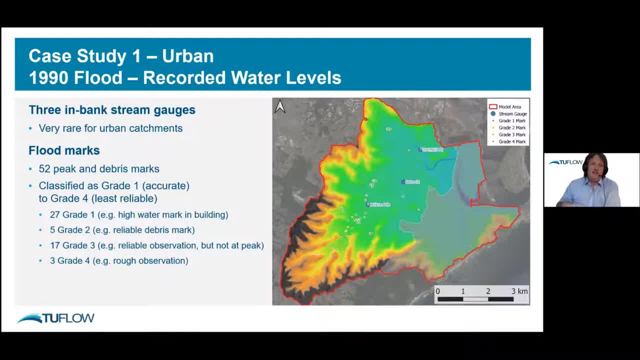 which is pretty rare for urban catchments, at least here in Australia, which is pretty rare for urban catchments, at least here in Australia- and a range of flood marks as well, throughout the floodplain, And they were actually split into four different classifications. 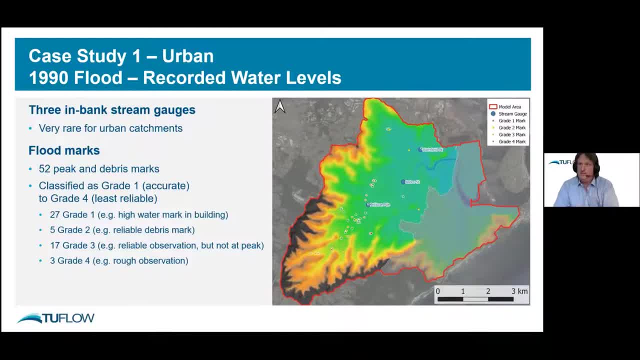 based on how accurate they were believed to be. So in that first category, Grade 1 marks, we had 27 of those. So an example of that would be a high-water marker recording in a building. Grade 2, less of those thought to be reliable debris marks. 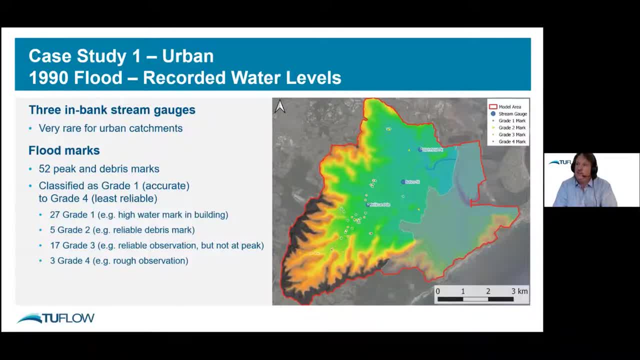 And then once we get into Grade 3 and 4, they might be reliable observations, but either not at the peak or the Grade 4 ones were more observations that we had less confidence in. So throughout this presentation I'll mainly focus on the 27 Grade 1 marks. 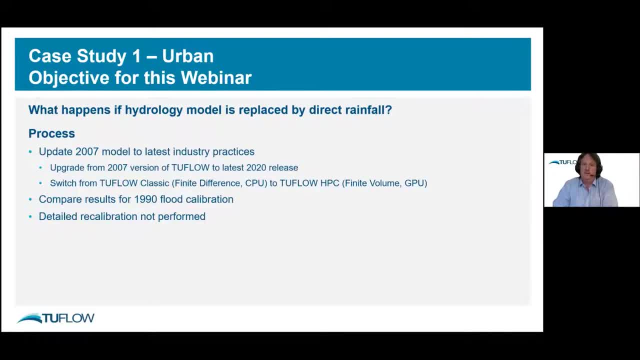 because they were thought to be really high-quality flood marks. The aim of today is really to compare: is direct rainfall accurate compared to a traditional hydrology approach? So what happens if we replace that hydrology model with a direct rainfall? So the process we went through is to: 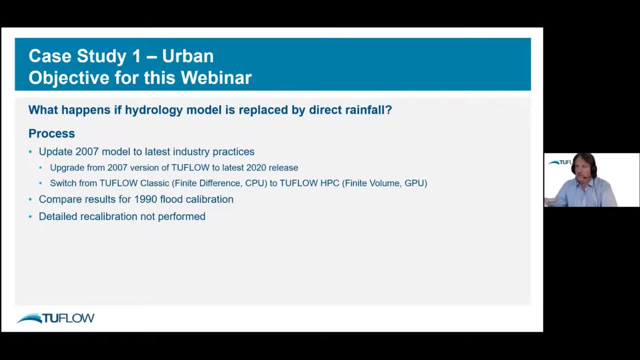 update the 2007 model to the latest, greatest version of TuFLO. We also switched from the TuFLO Classic, with a finite difference CPU-based solver, to TuFLO HPC, which is a finite volume GPU-based solver, And what we did was compare the results back to that 1990 flood calibration. 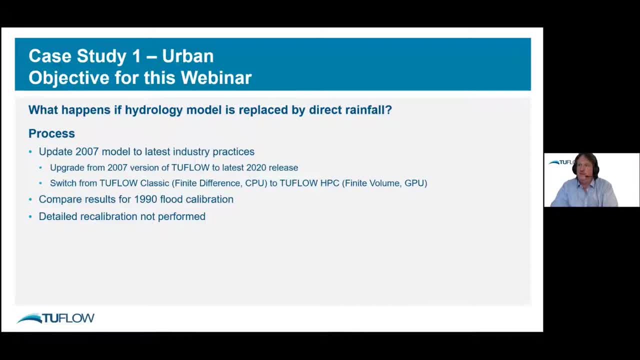 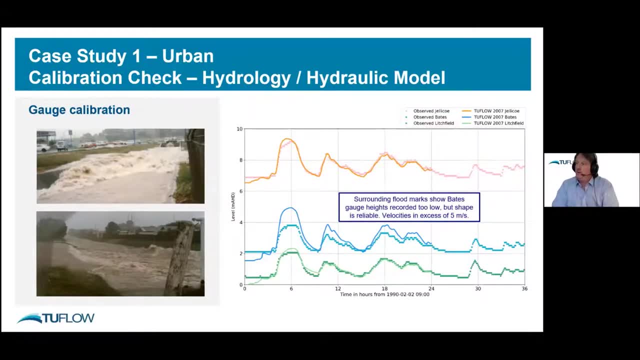 So we didn't actually go through a detailed recalibration process. What we did was make sure that we were getting a similar level of accuracy in our calibration. So for the three gauges there, this is with the original model results. So this is with the 2007 model results. 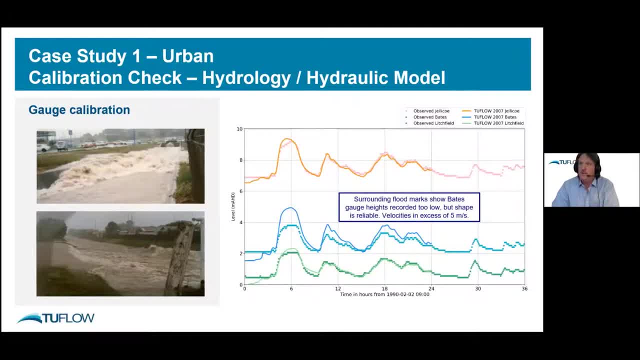 the calibration time series over there And a couple of photos of that event. So I've made a note there in blue that the Bates gauge, which is the blue gauge, it's thought that the recorded levels were too low, but the shape is reliable. 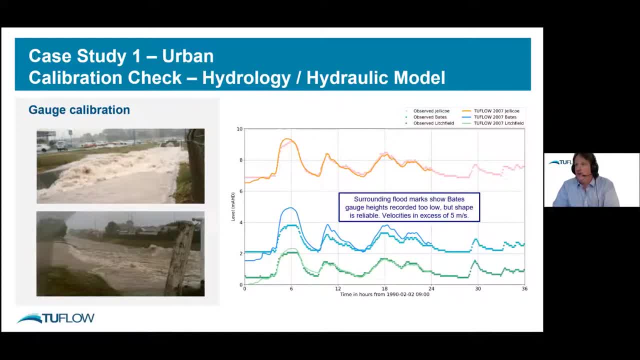 The recorded levels actually don't match with the surrounding high-quality marks. So we think that the timing is correct. but there's question over the actual level that that gauge was reporting. But there's also good evidence that the very high velocities in those channels 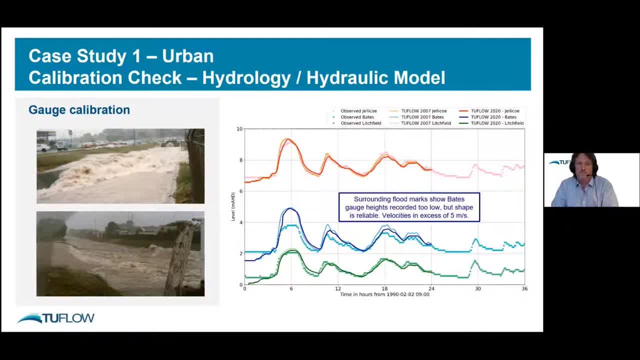 as you can see from the photos and some of the damage that was done, Adding on a next line. So that's the same model with a hydrology inflow, just running with the latest version of TuFLO and the update from the TuFLO Classic to the TuFLO HPC. 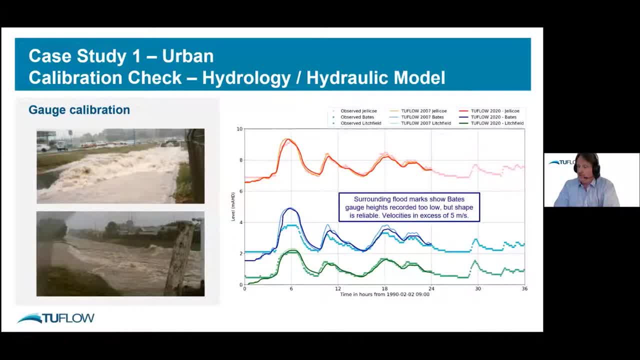 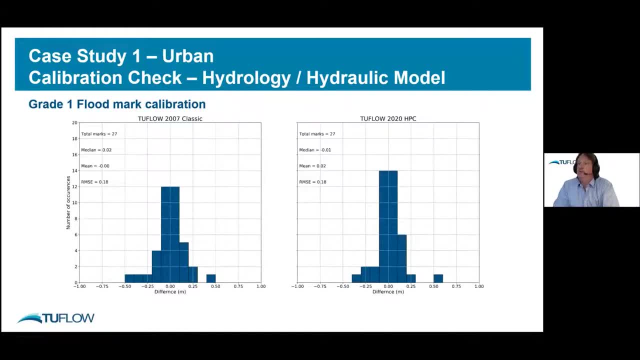 So not a huge change in the results there. A little bit of change in the time series. If we go to looking at a histogram of those flood levels, the 27 grade one flood levels, that's the spread that we've got. So on the left hand side was the original 2007 data set. 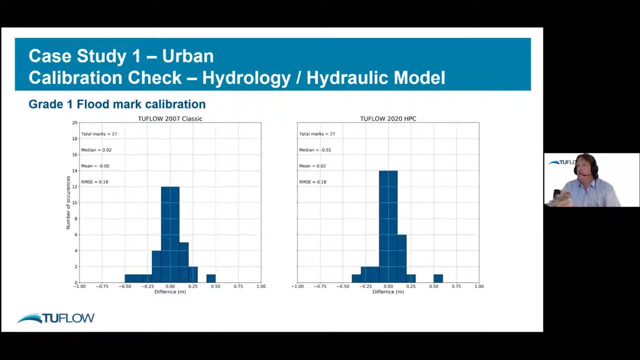 On the right hand side is the revised one. So a very similar actual level of calibration in terms of those peak water levels, similar in terms of mean median and also a root mean squared error. So we were pretty happy that we hadn't by changing. 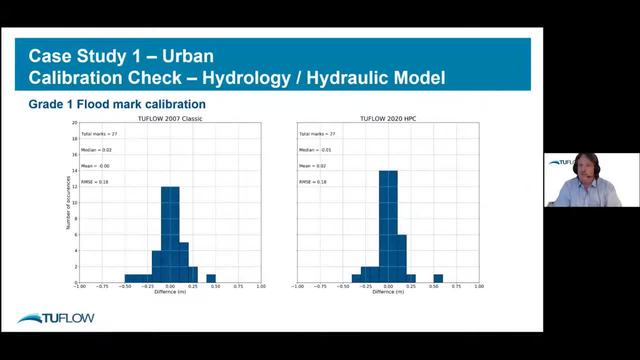 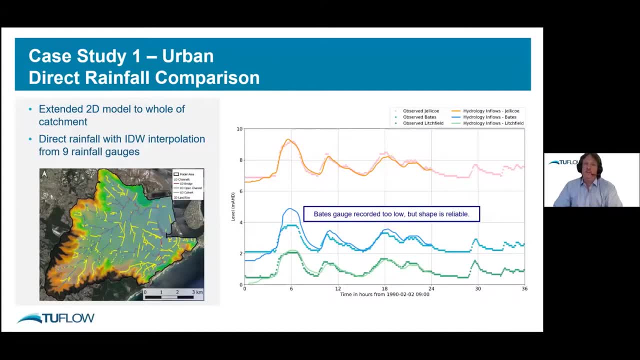 the software. we hadn't adversely affected the calibration, So we basically went ahead with no changes to the model apart from a software update, And so we took that as our base case with the hydrology model, the latest version of TuFLO. 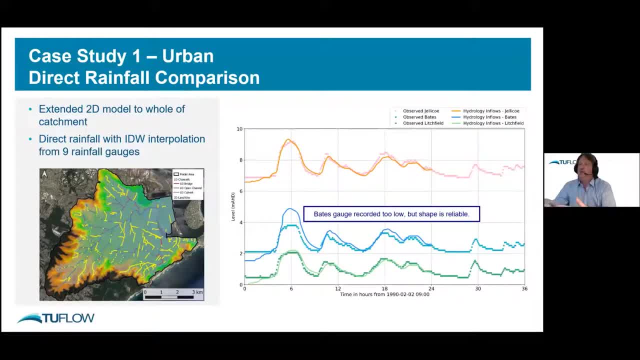 And then what we did was extend that 2D model to cover the whole of the catchment, to remove those hydrology inflows and to replace those with a direct rainfall. So in this case, in the bottom of screen, we're actually going from the 2D model area. 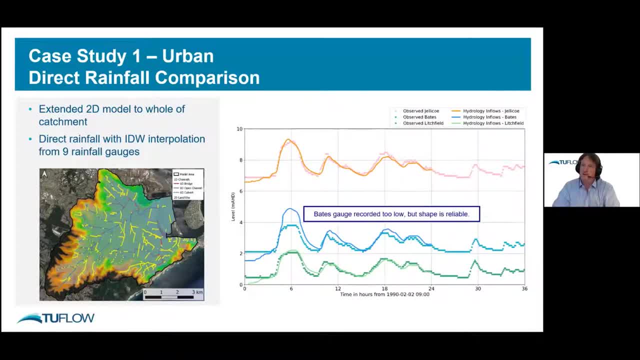 covering just the lower parts and admitting the steep parts of the catchment to covering that whole catchment, And we applied a direct rainfall based on an inverse distance weighting interpolation from those nine rainfall gauges that I specified. So on screen now is the hydrology. 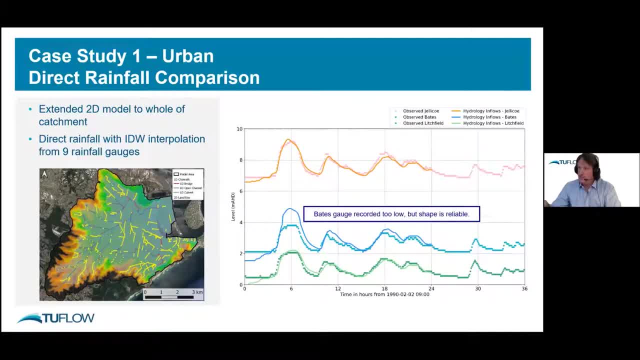 the calibration of the model to the time series for the hydrology approach, And in the dark colouring is actually the direct rainfall. So if I jump between those actually probably caught me by surprise. this one is that even with no changes to the model, 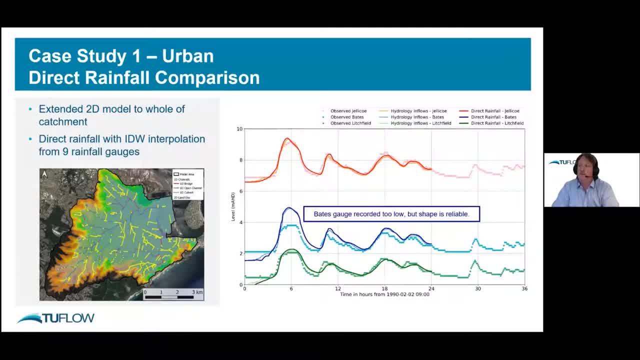 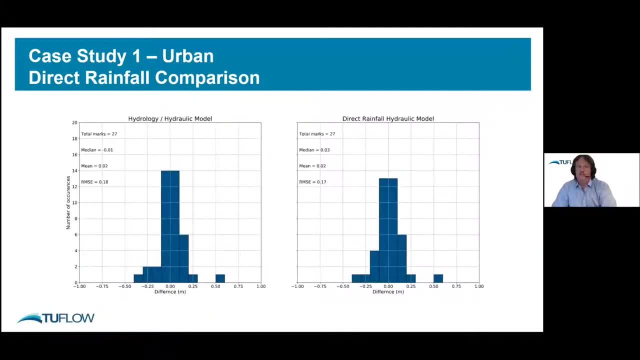 apart from replacing the hydrology with a direct rainfall, we're actually getting a pretty consistent calibration And once again, if we go to looking at the histogram of the differences in those level, one marks pretty similar level of calibration. our root mean squared error has actually very slightly decreased. 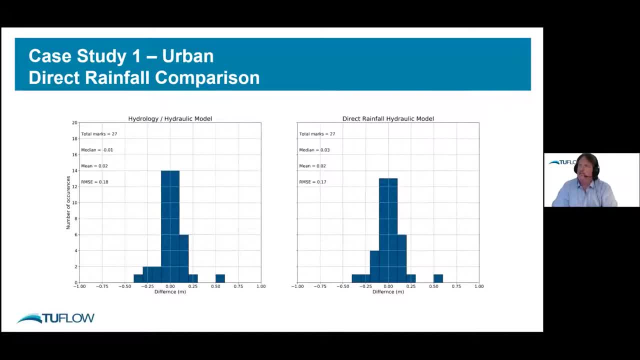 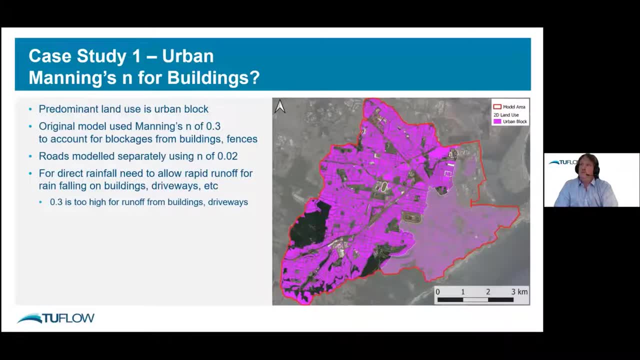 Looking at the time series, I probably think that the time series were a little bit nicer in the original approach, But in terms of peak water levels, it's actually doing a really good job, with no other changes Moving on one of the things that. 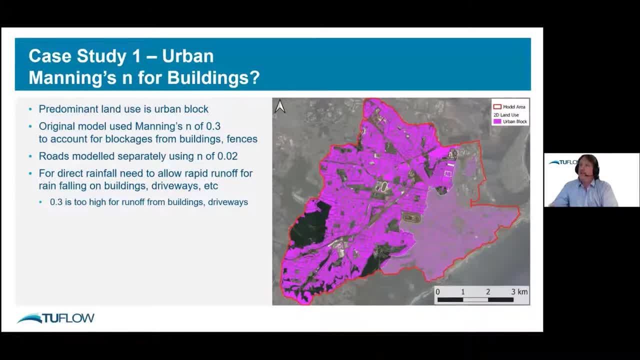 one of the main land uses in that catchment area was urban block, So urban blocks were classified in together. We didn't have that level of land use definition where we had individual houses and driveways digitised separately. It was digitised at a block scale. so urban blocks. 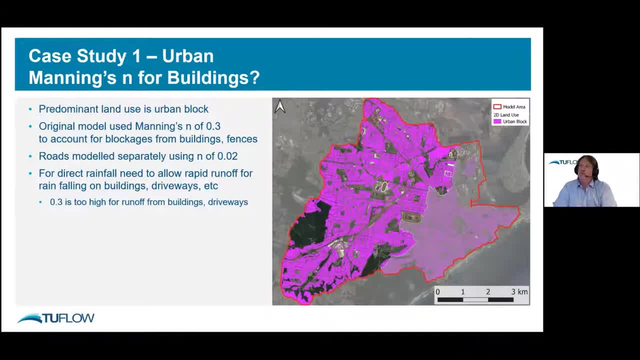 And the original model was calibrated with a Manning's value of 0.3 to account for the blockages from buildings and fences. So, of note, the roads were modelled separately with a typical low Manning's N, but for those urban areas quite a high Manning's was used. 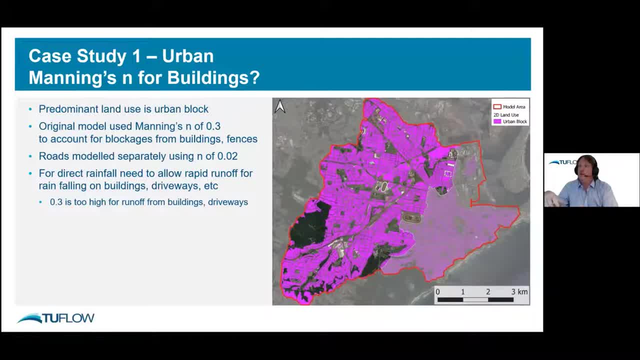 But for direct rainfall we probably want a more rapid runoff from those urban areas, particularly with counts, for you know where rain is falling- on buildings and driveways- we would expect to see a rapid response. So you know, 0.3 is probably too high for that. 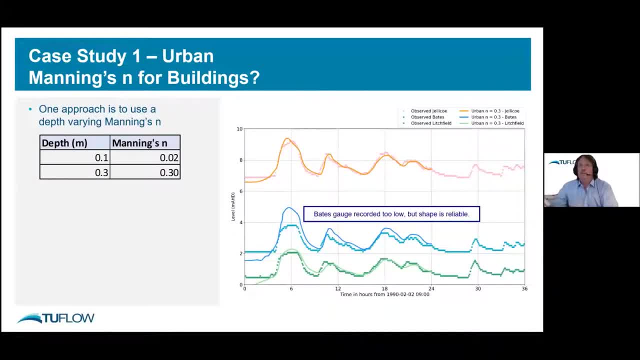 We also looked at depth varying Manning's. The reason that the high Manning's value was used initially was to stop having high flow paths through those urban blocks because of the fences in the buildings. So what we did was adopt a depth varying Manning's. 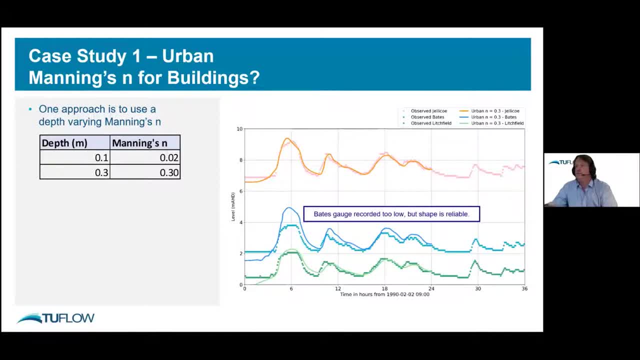 So a very shallow depth. it's actually very slippery, So water will run off those areas quickly. But once we get to higher depths and if those urban blocks become flow paths, the Manning's actually ramps back up to give it a quite resistant to flow. 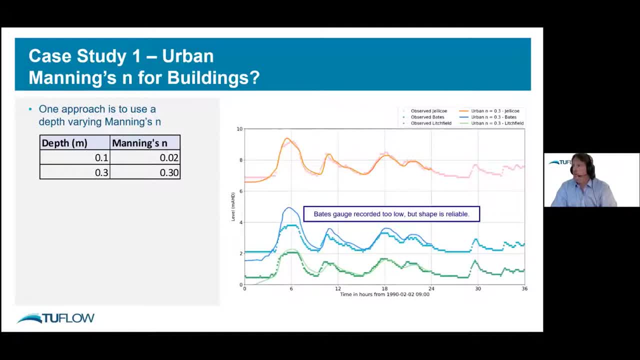 So in that case there's the original case with a Manning's N of 0.3.. And if I jump to the next slide, we've got that depth varying. So by putting in a depth varying Manning's we are getting a nicer shape. 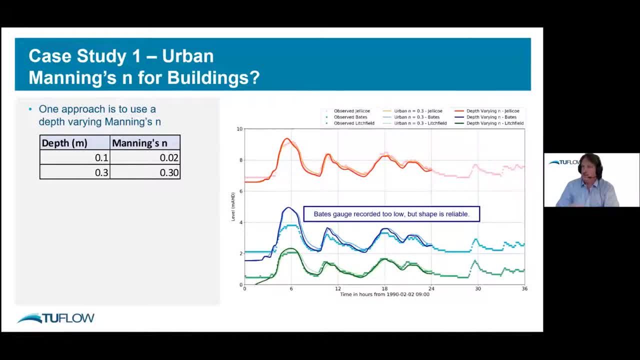 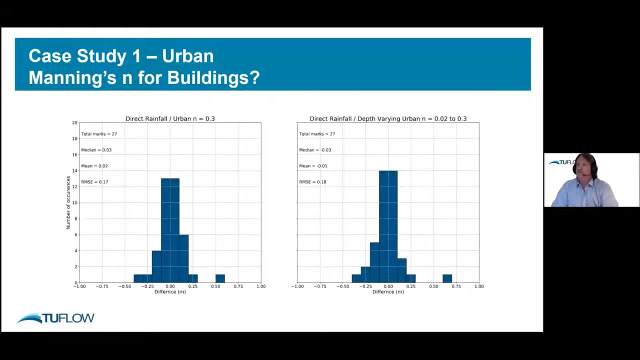 to match to the shape of the recordings, particularly on these rising and tailing limbs, but not a lot of difference in terms of the peak water levels in this case. So yeah, very similar in terms of the peak water levels between the two. 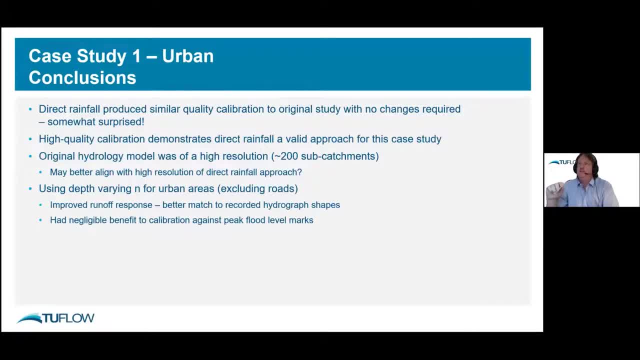 So that's probably where we'll leave that highly urbanized catchment. So you know, we think that with direct rainfall produced a really similar quality calibration to the original study, which used a hydrology hydraulic model with no other changes apart from the rainfall. 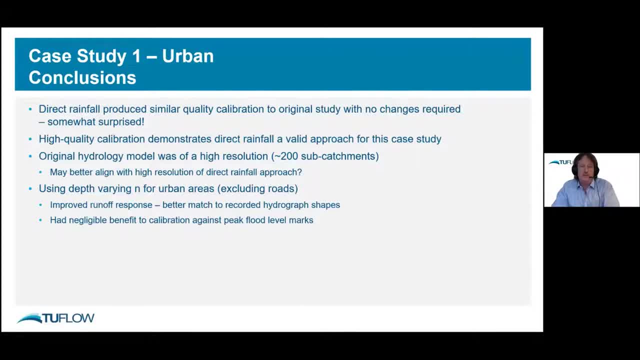 which caught me by surprise. I thought we would probably need to do a bit more tweaking of Manning's and things like that to get a similar level of calibration. I think that demonstrates that for a direct rainfall for this particular cage is certainly a valid approach. 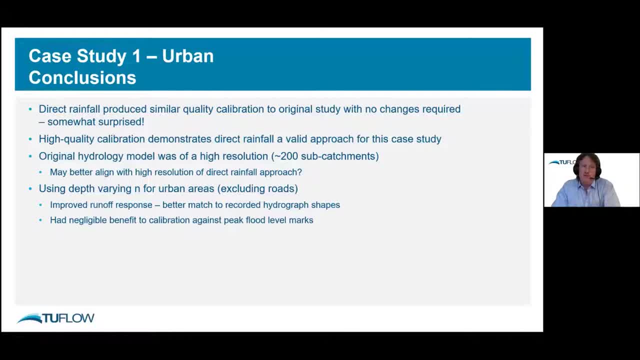 And I think part of the reason that we're getting similar results might've been because of the original hydrology model was quite a high resolution one, you know, broken down into a lot of little sub catchments, which was then applied to the 2D model. 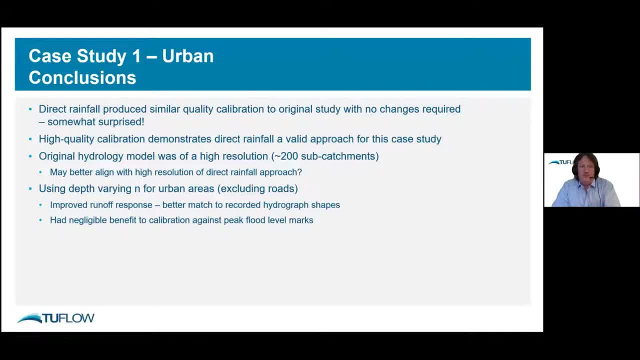 And certainly the use of depth varying for those urban blocks improved the runoff response better matched to the timing of those recorded hydrographs, but actually had not much benefit in terms of the peak calibration. So it would appear that a higher Manning's was required. 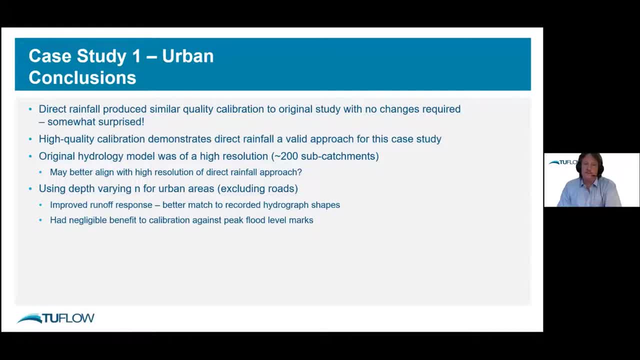 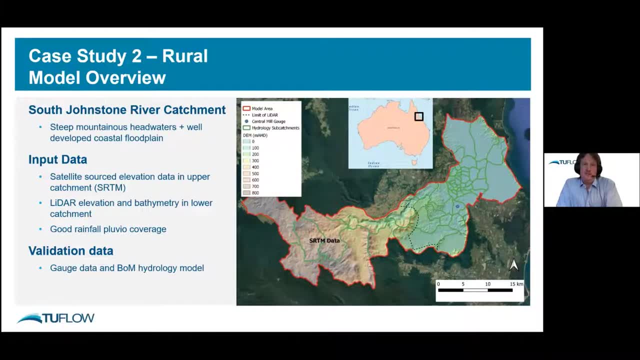 to actually to resolve those flow paths through urban blocks. So I'll jump onto a second case study which is a South Johnson River catchment in Queensland which I've got a DEM over there. on the right It's a steep mountainous headwaters. 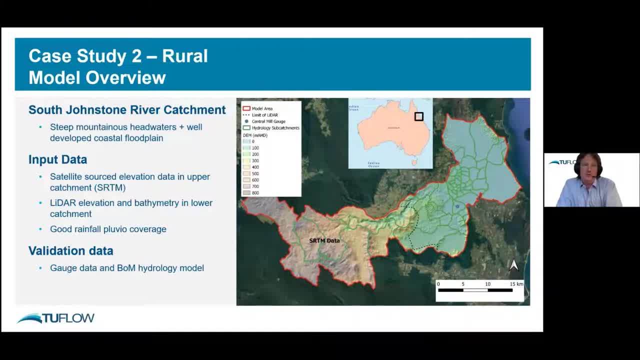 and a well-developed coastal floodplain spilling out into a very broad floodplain, And there's a line on that, a dotted line on that map, which is a distinction between the elevation data we had for the upper catchment, which was SRTM. 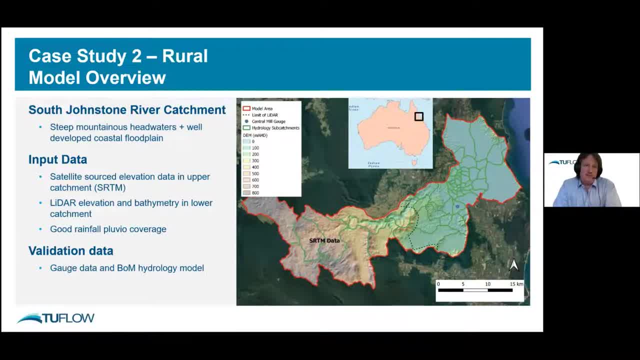 the shuttle radar topography data and also LIDAR and high quality bathymetry in the rivers in the lower area And once again we had a pretty good rainfall, pluvial coverage And, in terms of validation data, we had gauge data. 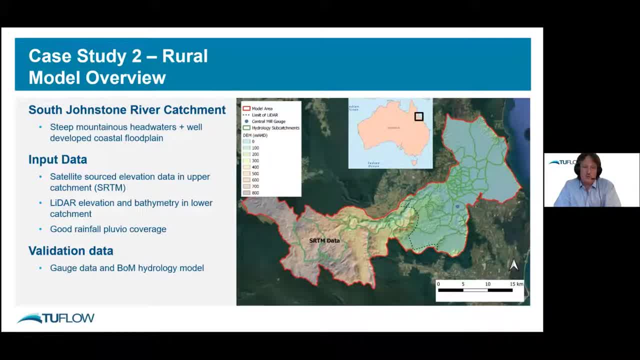 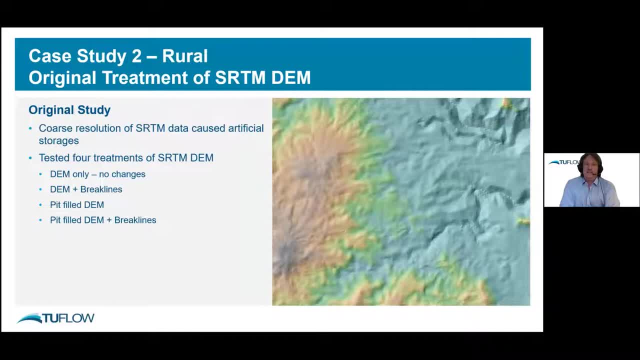 and then we also had a calibrated hydrology model, which was that one from the Bureau of Meteorology here in Australia In terms of the upper catchment and that SRTM data. what we found when we started running the model was that that course resolution of that SRTM data. 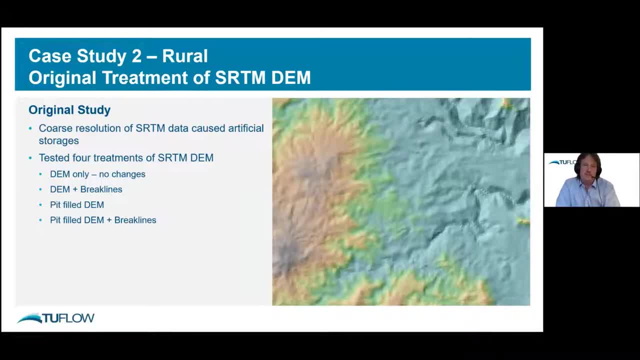 was causing artificial storages. We weren't seeing as much rainfall running off that upper catchment, So we actually tested four different treatments of that SRTM elevation data. So the first case: we just read the DEM, the elevation model, directly into TuFlo. 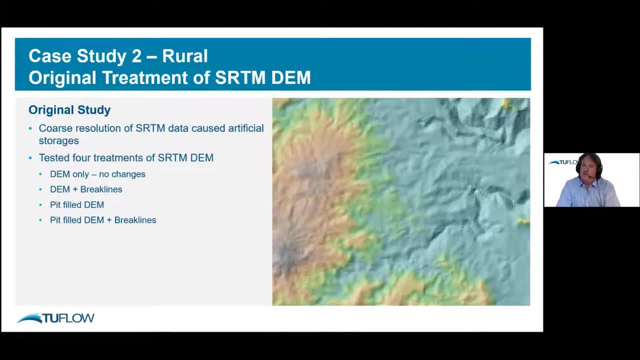 and we had no other changes. The second case: we put brake lines. in TuFlo terminology we probably refer to these ones as gully lines, so they're enforcing flow paths to make sure we've got a continual connection. The third case is a pit filling. 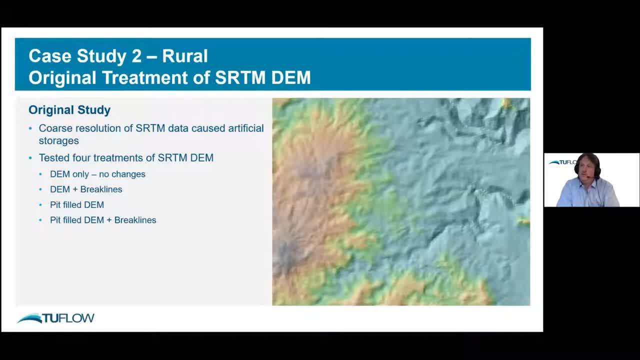 So we actually ran that DEM through a pit filling process in a GIS package and used that in the model And the final case is a pit filling as well as those brake lines to ensure the flow paths. I'll jump to some results for the time series there. 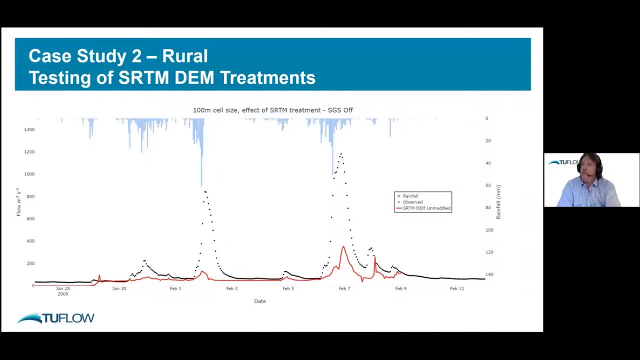 So that's what we're seeing. So in this case we've got 100 metre TuFlo cell size and we've got sub-grid sampling- which I'll talk more about later on- turned off at this stage. So with untreated DEM we're really not getting. 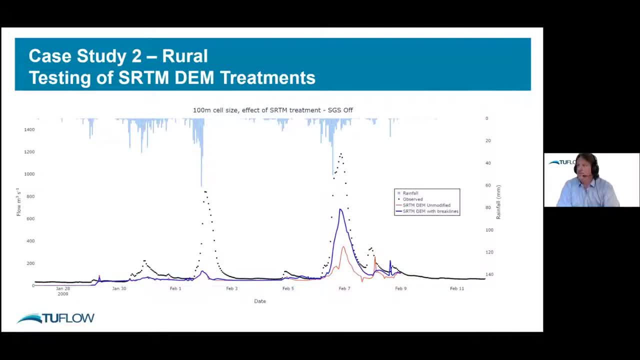 a great rainfall runoff response at all. Now, adding in the blue line and we've added in the brake lines, it's getting more water down the catchment but still not really ideal. Thirdly, we're bringing in, you know, 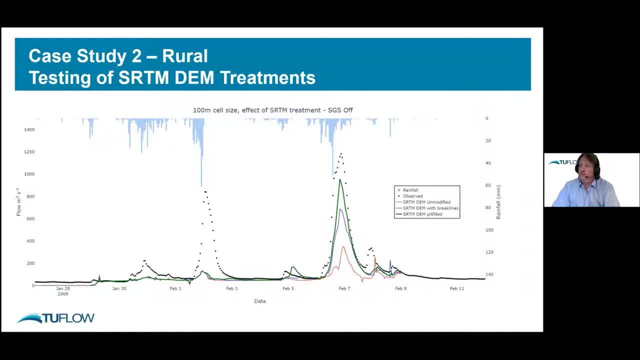 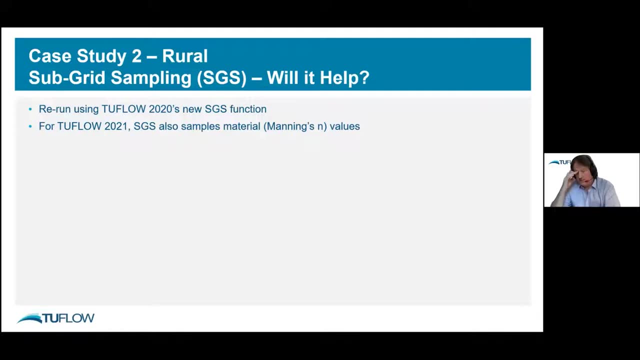 the pit filling in pit filling, which makes more of a difference. And finally we've got both the pit filling and the brake lines, none of which I would call a good calibration to that data set at all. We ran that with the sub-grid sampling functionality. 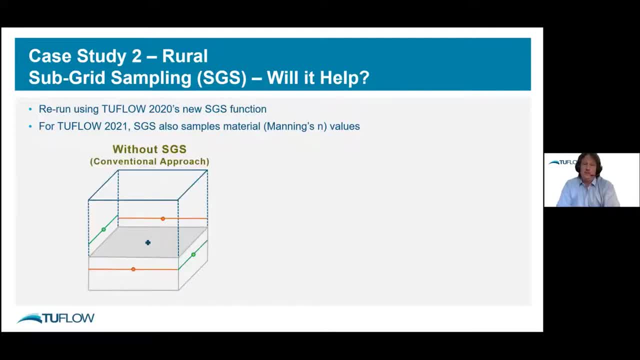 which has been released in the TuFlo 2020 version, which so the traditional approach within TuFlo is a single elevation per cell and an elevation per cell phase, whereas with the sub-grid sampling turned on, multiple elevations through the cell and the cell phase as well. 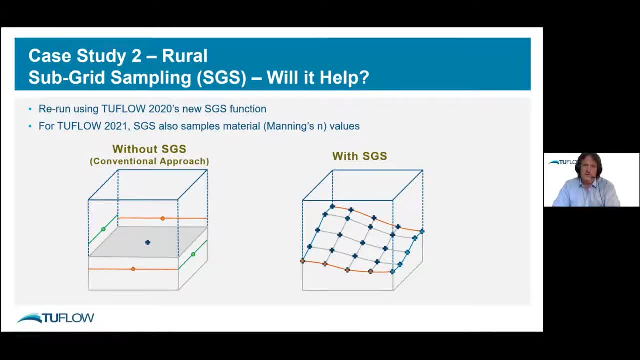 For the 2021 release of TuFlo. we've actually allowed a sampling of material or land use across those cell phases as well, as well as depth varying mannings as well. So depth varying mannings across. that has been for a while. 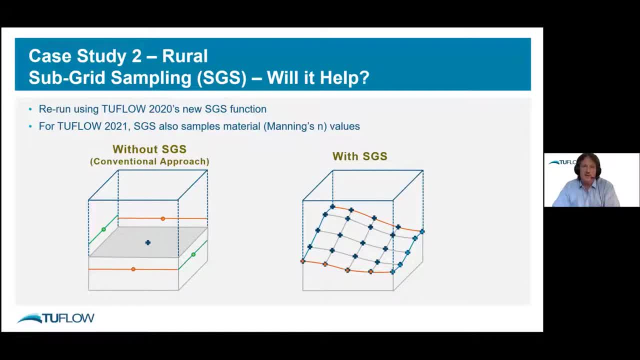 but the 2020 brings a spatial sampling of mannings across there as well. Still only get a single velocity calculation per cell phase, but a better representation of both the elevations and also the underlying land use across there. So jumping to the sub-grid sampling. 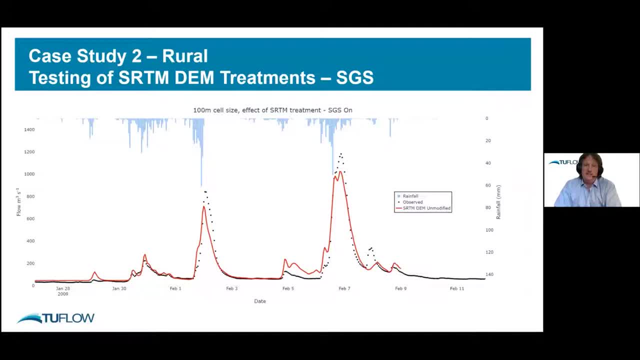 we've got the same results. The red line there is the same as previously. That's the SRTM data unmodified, but this case we've got the sub-grid sampling turned on, So quite a big difference from the original data sets. 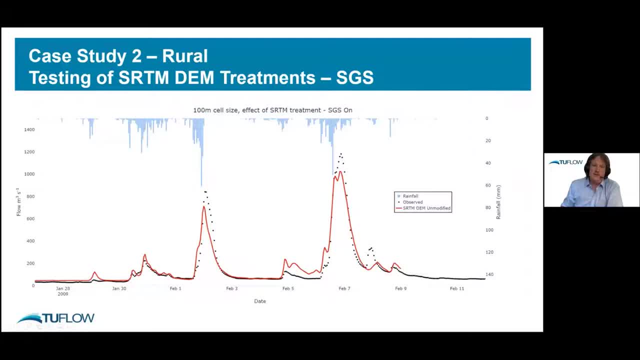 which really didn't. or the original sub-grid sampling off, which really did not pick up any of those big, those first flow events, well at all, Adding in the break lines, the pit filling. So these are making less difference now with the SGS. 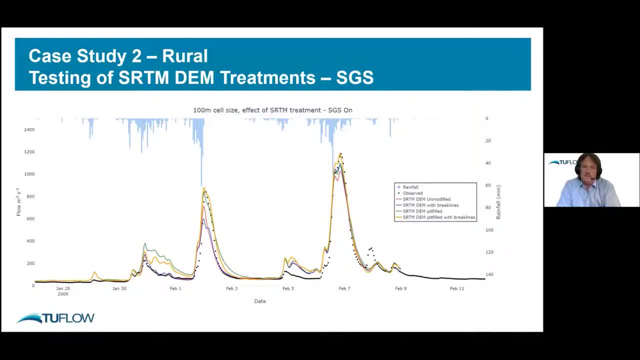 but they are still actually making a difference there. So there certainly is a need, particularly where you've got very coarse elevation data, to maybe do some pre-treating of that if you're going to be using it for direct rainfall. But the sub-grid sampling feature in 2Flow 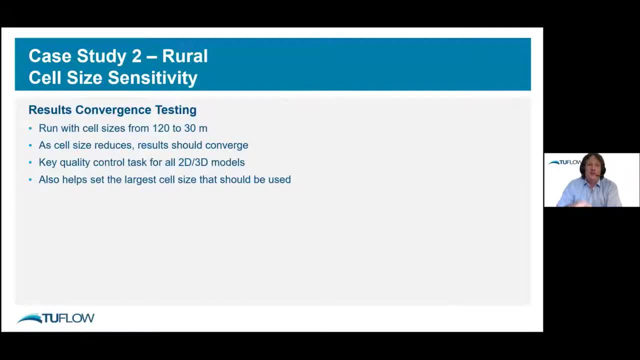 does help that quite a lot, but it's not a magic cure. So we ran a test on cell size convergence. So we ran that with cell sizes from 120 metres down to 30 metres. So as that cell size reduces, what we would expect to see is those results converge. 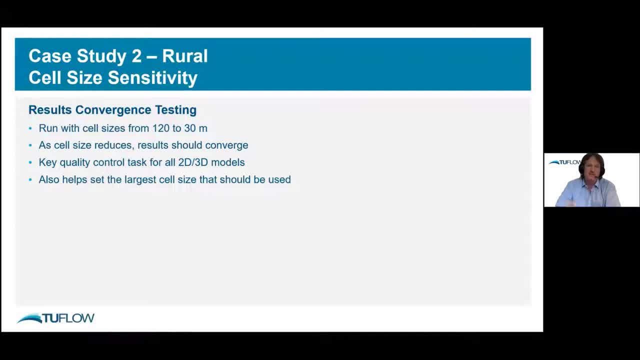 to a consistent answer- And it's a really good quality control task for all 3D models- is to look at mesh or cell size convergence, And it also helps us to work out what the largest cell size we can get away with. Obviously, there's a trade-off between runtime and cell size. 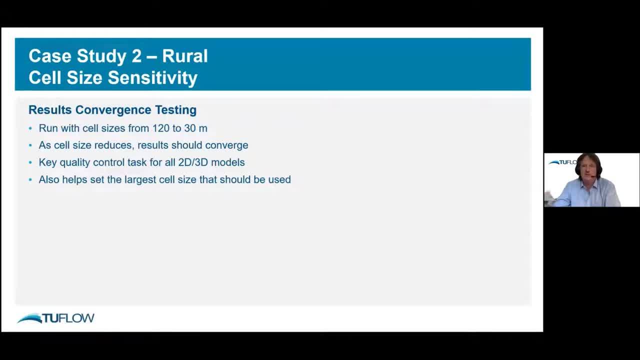 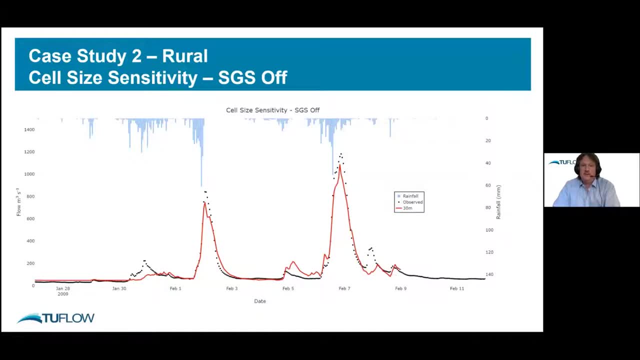 So if we know we can get consistent results at a larger cell size, we can certainly do a lot of our calibration at that coarser cell size with faster runtimes. So in this case, looking at the 30 metre cell size and the 60 metre cell size, 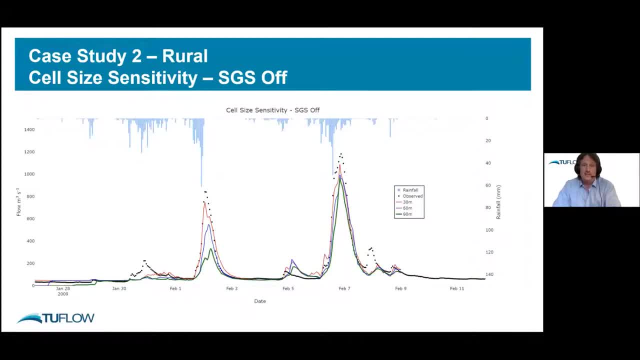 we're not seeing the big differences that we were seeing in the SGS- Sorry, this is the SGS off, So we are seeing big differences there in terms of those results between those cell sizes As we get down to 90 metres and down to 120 metres. 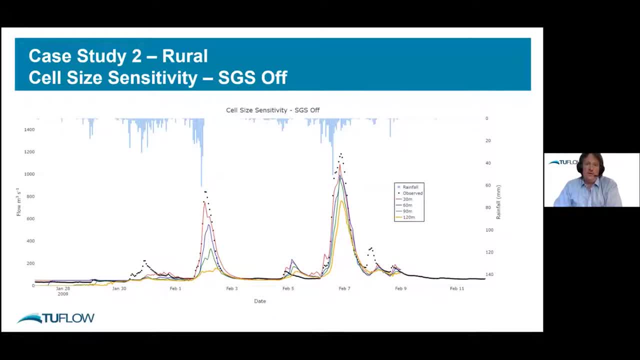 we're really not capturing those flow peaks as well with a coarser cell size. If we jump across to sub-grid sampling on, we've got the 30 metre cell size there, adding in the 60 metre, And now we're seeing a little difference. 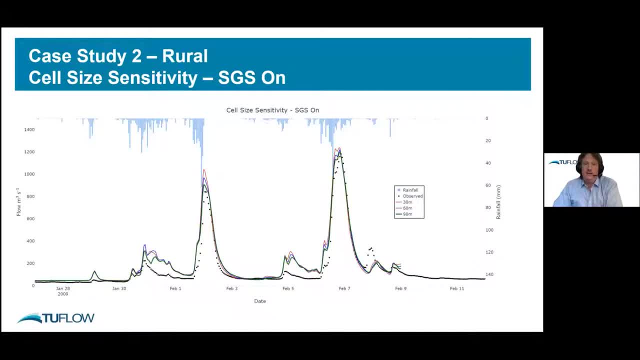 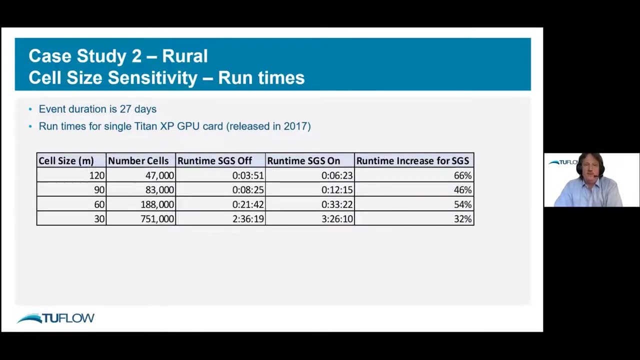 much less difference in those results. Adding in the 90, and we're still getting a similar flow peak there at the main peak of that flood event Does drop down a little bit with that 120 metres cell size. So that model was running for 27 days of simulation time. 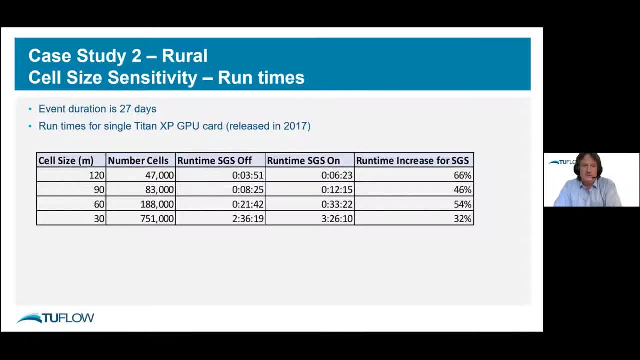 So a very big catchment with long duration rainfall events and long runoff times. Comparing the runtimes of those and numbers of cells, you know 120 metres, we had 47,000 cells in that And the runtimes are in the order of minutes. 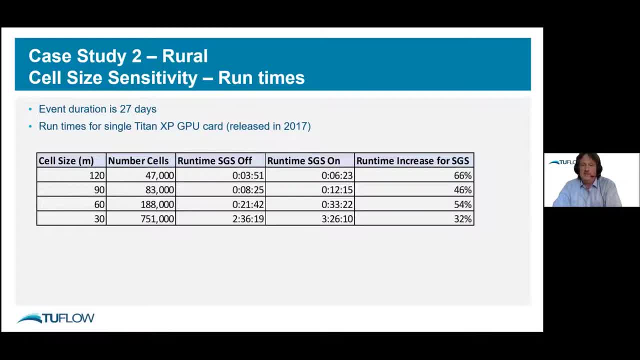 you know, four minutes for the SGS off case and six minutes for the SGS on case, And they're runtimes for a single Titan graphics card, which is originally released in 2017.. So it's a decent card, but it's not latest and greatest. 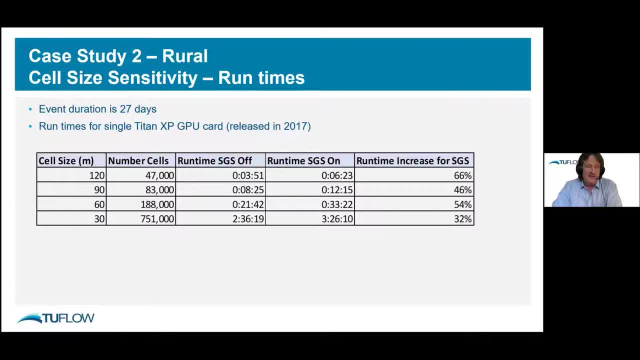 We probably see those runtimes, hopefully hard, if we could get our hands on a 3090, which seemed to be very, very rare at the moment, And of those you know for the SGS off. we really needed to be down at that 30 metre cell size. 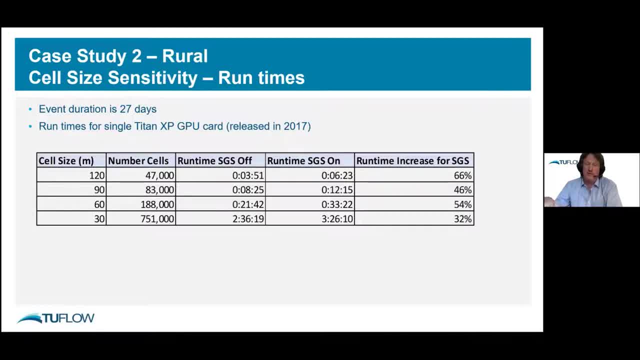 to be able to get that rainfall runoff response looking reasonable, Whereas with the SGS on probably I would have been happy with 90 metres or less. you know, I think the 30, 60 and 90 all gave pretty consistent results there. 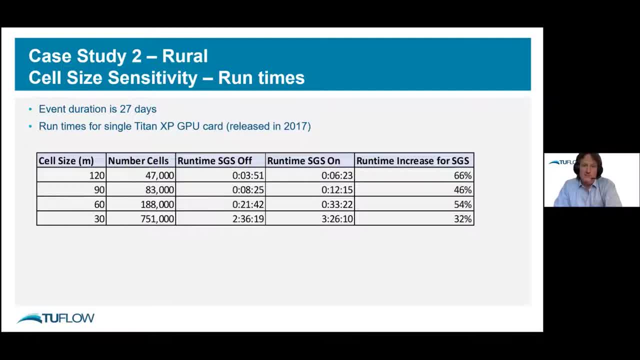 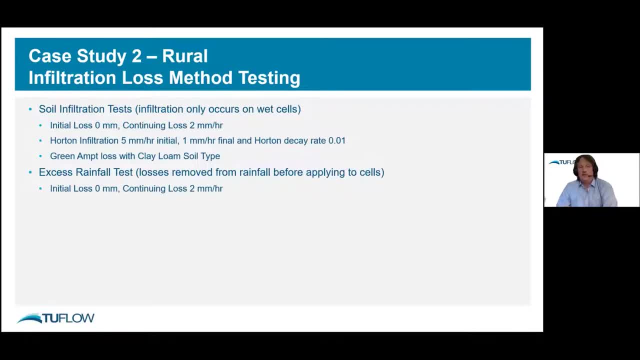 So we can get away with that. and you know runtimes of 10, 12 minutes to run a- you know, almost a month worth of data through is not too bad. So once we had a model that we were happy with, the cell size. 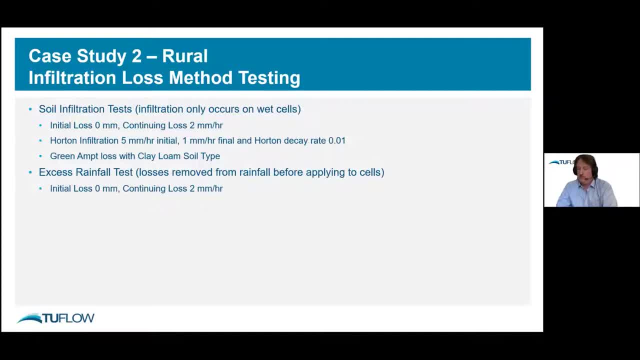 we looked at infiltration and how we can, you know, get those losses into the system. So there's a number of different ways we can apply those. So we looked at soil infiltration. So that's applying that infiltration on any wet cells, So once a cell becomes wet, 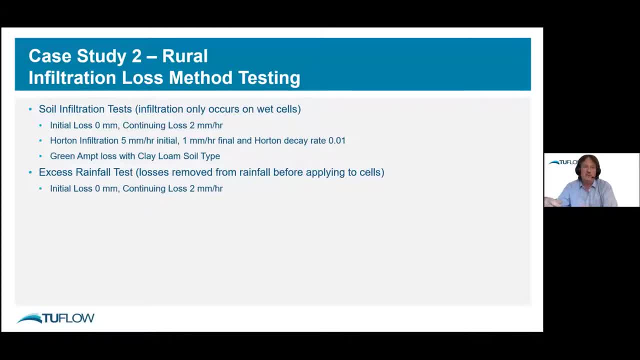 it can start to infiltrate water in. And we've done three different approaches for that: An initial continuing loss method And in this case, because we're running such a long- you know, almost a month's worth- we've actually set that initial loss to zero. 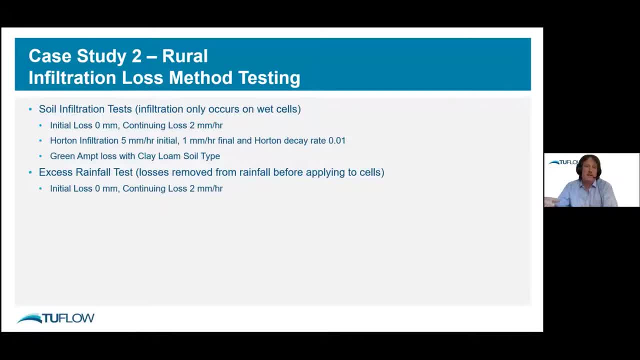 It only affects 10.. So that's the very start of that hydrograph: A Horton infiltration where we have an initial, a final and a decay rate and also a green amp type loss where we've applied a clay loam soil, And the last one in there is actually a rainfall excess test. 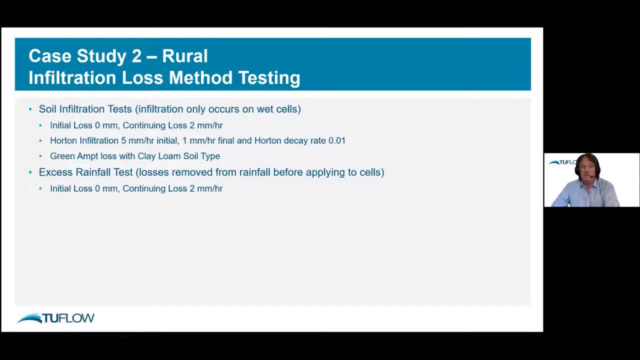 So in that case the rainfall is actually removed, The losses are removed from the rainfall before that rainfall is applied to the 2D cell size, the 2D cells, And we've adopted the same losses as for the soil infiltration. We've used 100 metre cell size. 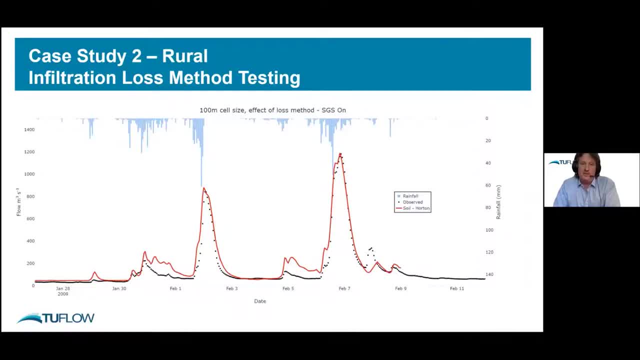 I didn't actually show that in my cell size conversions but it gives quite similar answers to that to the 90 metre So we're happy with that. Gives us nice quick run times. So having a look at the effect of that rainfall loss method. 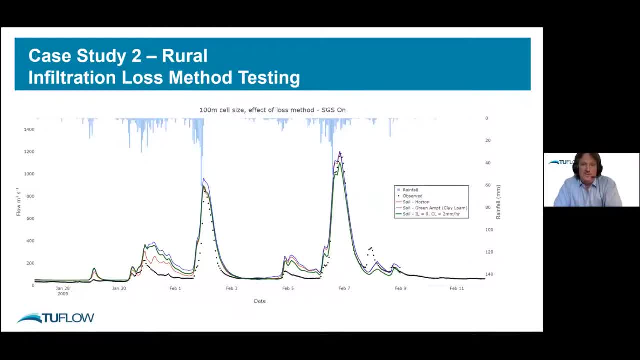 green amps- initial and continuing loss on the soil type and a rainfall loss being applied. So we can actually see that applying that rainfall loss to the rainfall- it's essentially a rainfall excess- gives a higher flow rate. that does the same infiltration rate applied to the soil, because the soil will keep infiltrating. 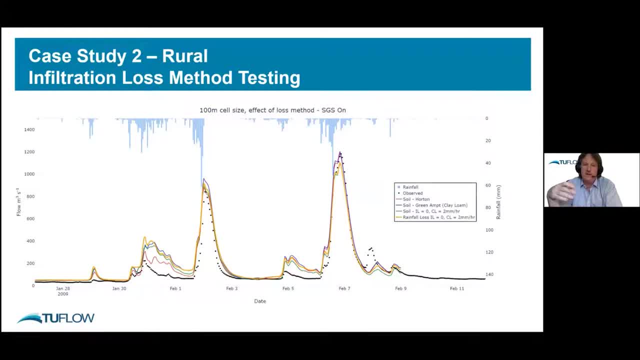 that water out even when there's no rainfall. As long as those cells stay wet it will continue to infiltrate. So that's why we see a slightly higher flow hydrograph for that rainfall excess approach. Obviously we've sort of dialled those in to give roughly the same peak flow. 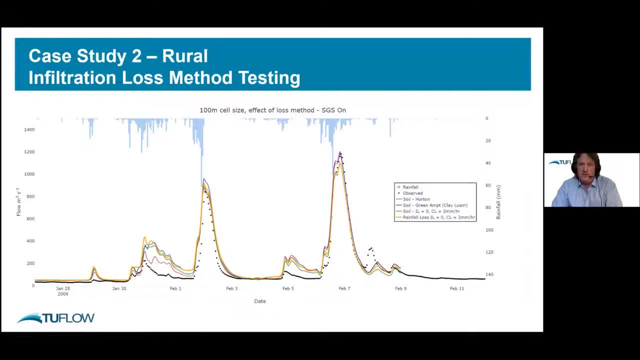 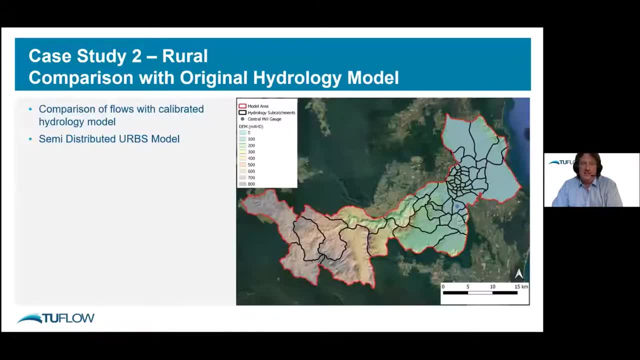 Obviously that you've got a lot of calibration knobs to turn. if you're changing your soil types and things like that in order to match those flow records, I guess the key question is probably: how does that compare with a calibrated hydrology? So in this case, comparing back to a semi-distributed ERBs model, 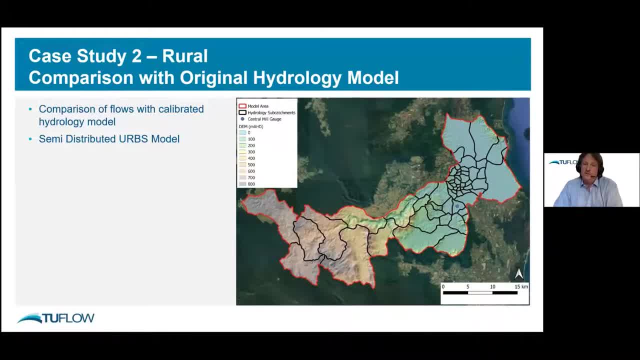 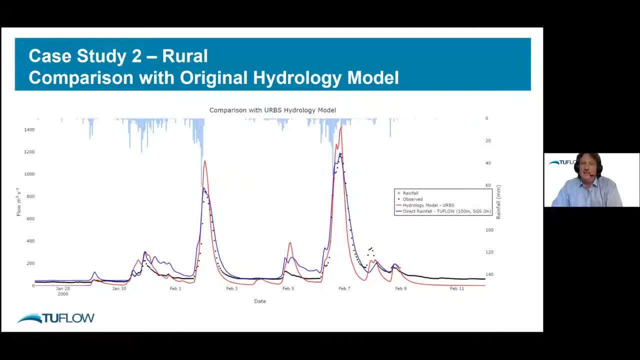 So in black there on the screen are the ERBs- hydrology sub-catchments. So there's about 20 or so sub-catchments upstream of that rain gauge And in this case in red we've got the flows from the hydrology model. 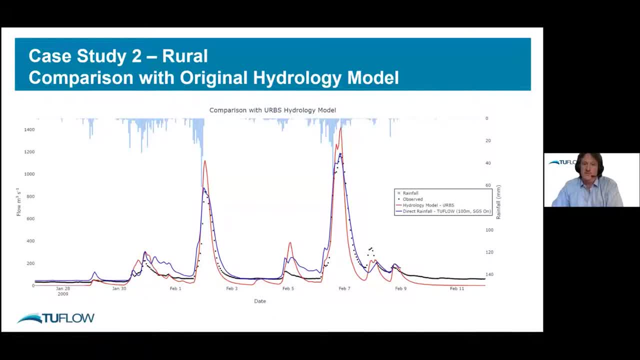 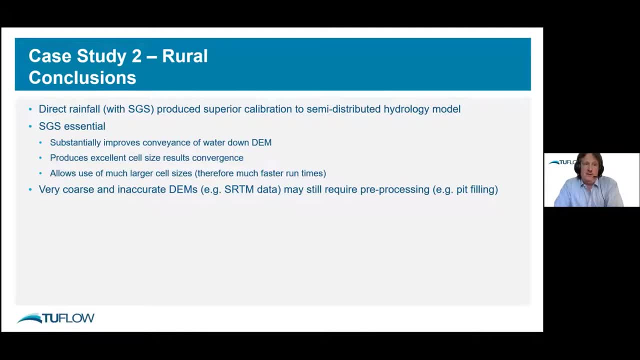 comparing that to the flows in blue for the direct rainfall model, That's at 100 metre cell size with the SGS turned on. I'd probably argue there that the direct rainfall access actually produces a superior calibration to that semi-distributed model. The run times for that: it's probably 10 minutes or so for the two-flow model. 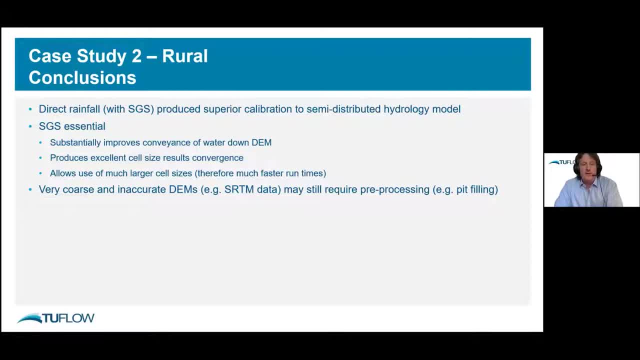 is probably seconds for that hydrology model. But of note is that that SGS sub-grid sampling really is essential to get that conveyance coming down the DEM right. And the SGS also gives us excellent cell size convergence and allows us to use larger cell sizes and therefore faster run times. 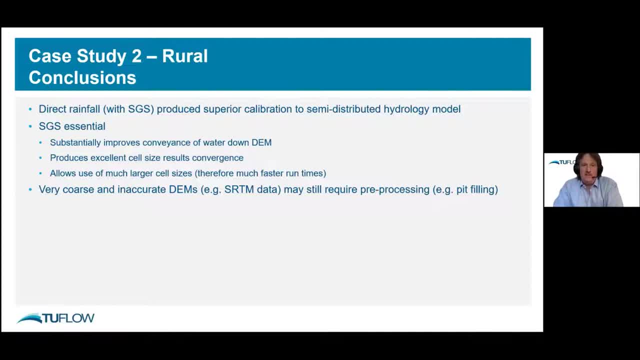 But it won't make up completely all of that. It won't make up completely for DEMs that are coarse or inaccurate. So you know we had to do some massaging of that pit filling and enforcing of brake lines in that SRTM data. 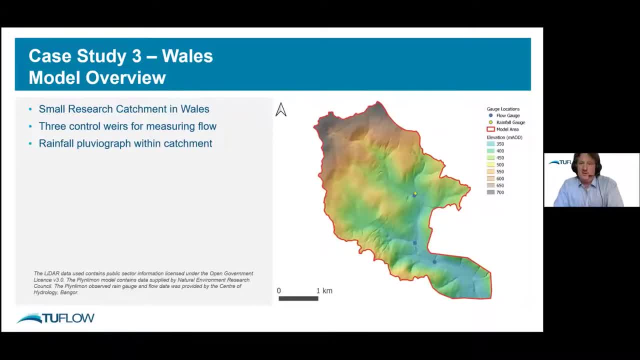 in order to be able to get that looking reasonable. So, moving on to the third and final catchment. So this is actually a small research catchment in Wales where there's actually control weirs in those locations shown in blue. So there's actually three weirs. 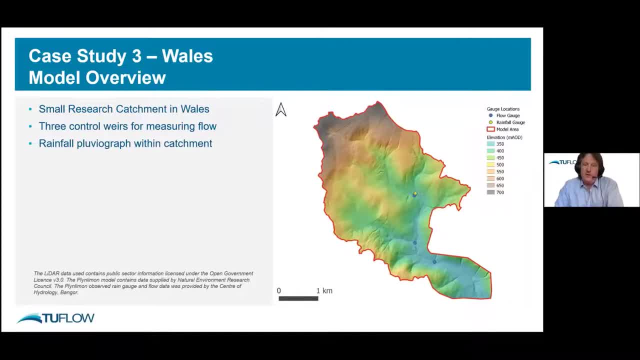 So to get a good recording of flow we're going to have to do a lot of work with a known sort of water level flow relationship. And there's a rainfall, pluvio in the middle of that catchment And it's quite a small catchment as you can see from the one kilometre scale bar. 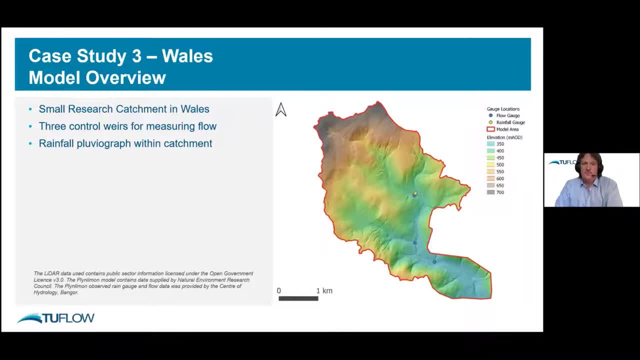 Orders of magnitude difference in terms of the last model that we just looked at, And the focus of the calibration that I'm going to present is actually really all that downstream gauge, which is Keffenbrun, So apologies for anyone who knows Welsh at all. 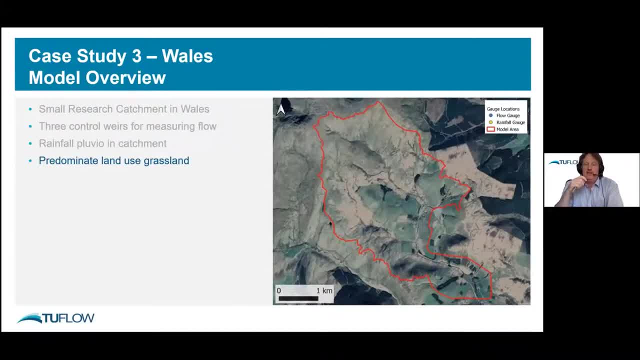 I probably murdered that pronunciation. So predominantly grassland land use in there. There's actually two different grasslands that have been defined in there, An improved grassland and an acid grassland, which I'll show a bit later on. So, as we did for the South Johnson catchment, 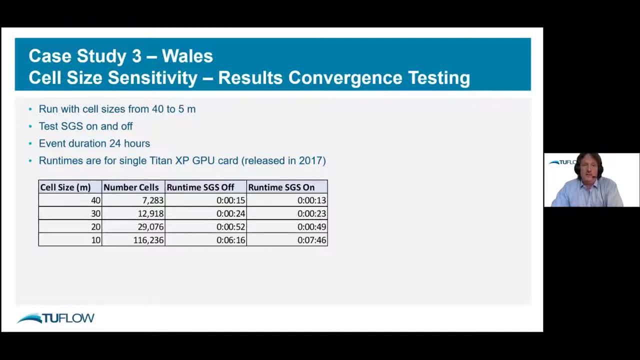 we looked at a cell size convergence. In this case, we ran the model with cell sizes from 40 metres down to five metres, Once again with and without subgrid sampling. In this case, we're looking at a smaller rainfall event. 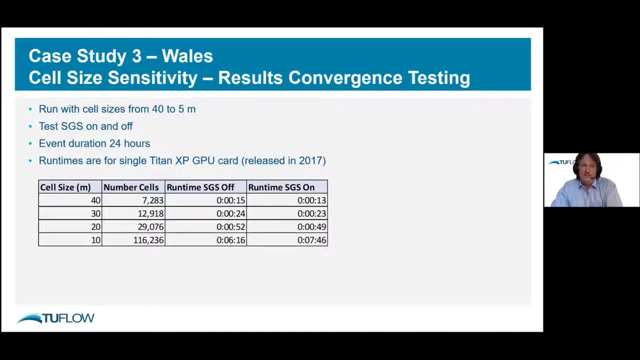 It's a 24 hour duration runtime And, once again, the runtimes are for the same Titan GPU card. Interestingly for the smaller cell sizes, the SGS runtimes are actually slightly lower, And that's due, I think, in part to it being able to run with a slightly larger time step. But in that order of magnitude of those runtimes it could just also be numerical noise in terms of what else is running on that computer when we ran those benchmark models. So as you start to get down to the high resolution cell size we do start to see that SGS takes a little longer to compute. 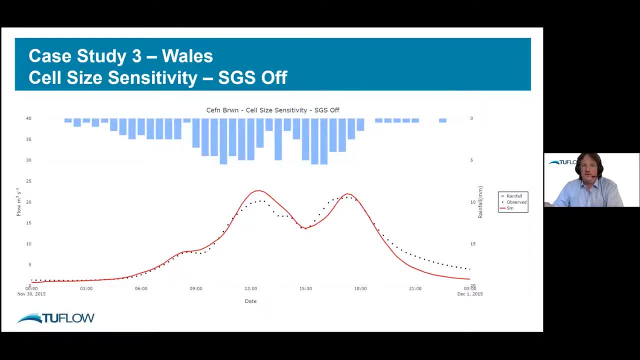 So, looking at cell size convergence, starting at the finest resolution here for the SGS off case at five metres, and that blue is there at 10 metres, Reasonably consistent there, As we start to increase the cell size further, though, we're really not getting that initial. 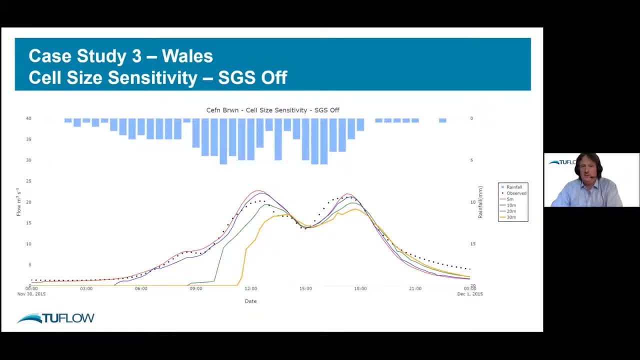 response: off that catchment And by the time we move to 30 metres we're going to be running at a higher resolution. So we're going to be running at a higher resolution. So we're going to be running at a higher resolution. 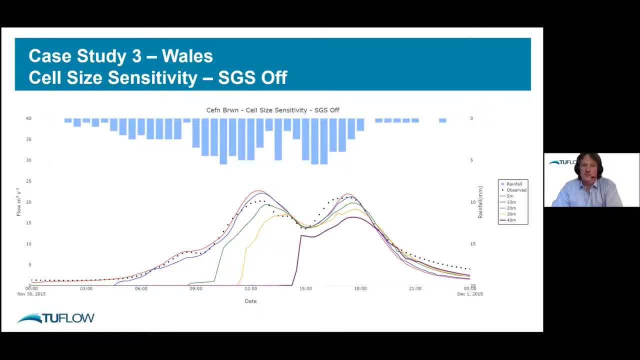 So we're going to be running at a higher resolution And 40 metres- yeah, we're really not doing a great job with direct rainfall approach If we compare that to the subgrid sampling on same cell sizes- five metres, 10 metres. 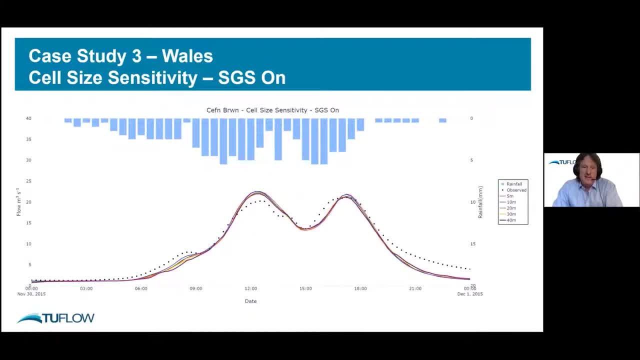 20 metres, 30 metres and 40 metres. So really good cell size convergence there. So I'd argue that we could probably run that model happily with a 40 metre cell size and get very similar answers to the five metres. You know, the runtime for that 40 metre cell size is 10 seconds or something. 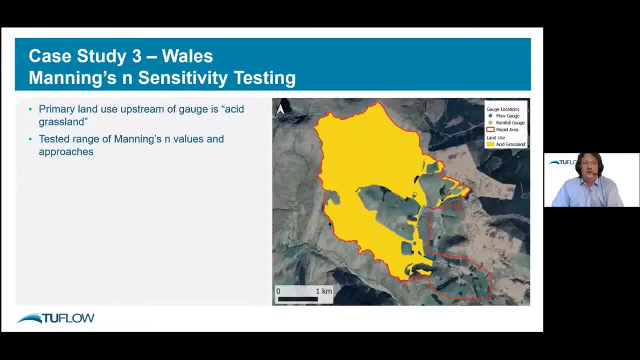 like that. so quite fast. So the primary land use in that catchment highlighted there is actually the acid grasslands which is highlighted there in yellow, And we did actually test a range of Manning's N values and also Manning's N approaches for getting that right. 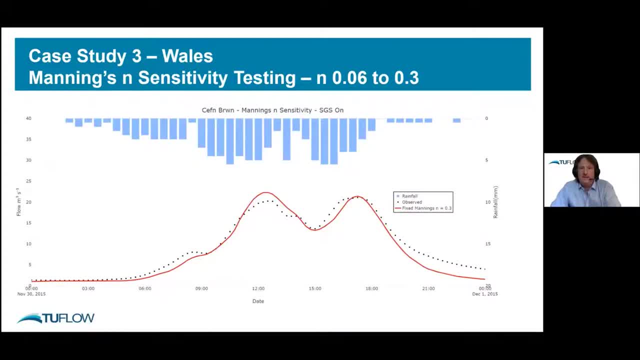 So the images that I've been presenting so far actually have had a fair amount of data, a fixed Manning's value of 0.3, which is probably higher than I would expect for that grassland type approach. you know, maybe in post-COVID world we'll be able to get out there and have a site visit to. 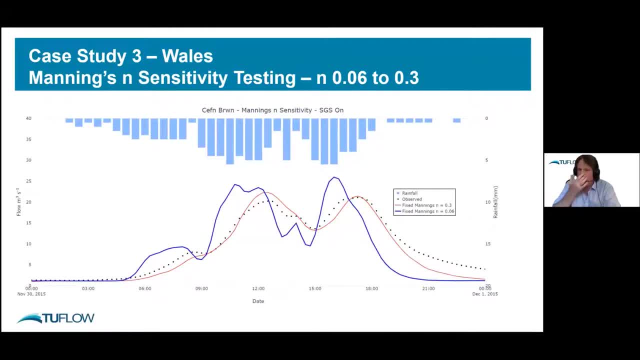 actually have a look at what it looks like out there, but I would expect that a Manning's value of, say, 0.06 would be more applicable to that grassland and that's shown there in blue. so that's, if we had a Manning's value of 0.06, which is probably more in the lines of what I'd expect. 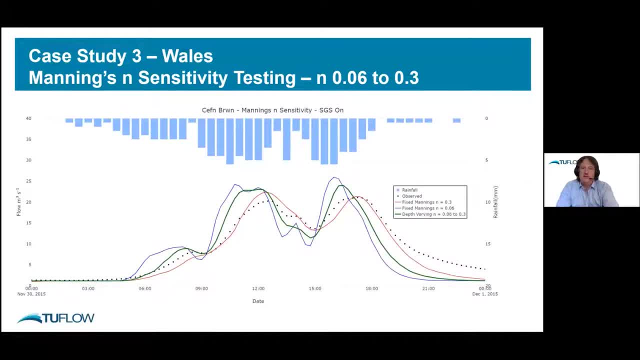 The third case that I've shown: there is actually a depth varying Manning's end, so varying that Manning's from 0.06 at higher depths and to 0.03 at lower depths, so having it more roughness, a higher roughness at those very shallow depths, transitioning up to a value of 0.03. 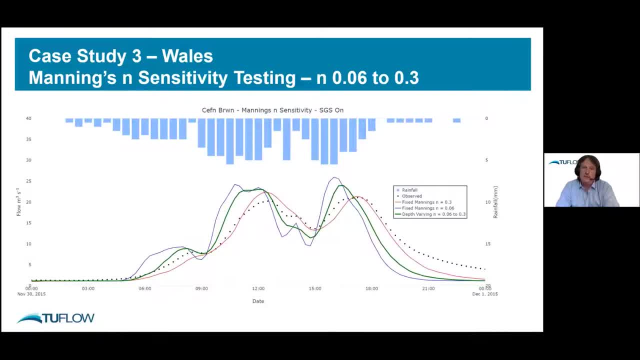 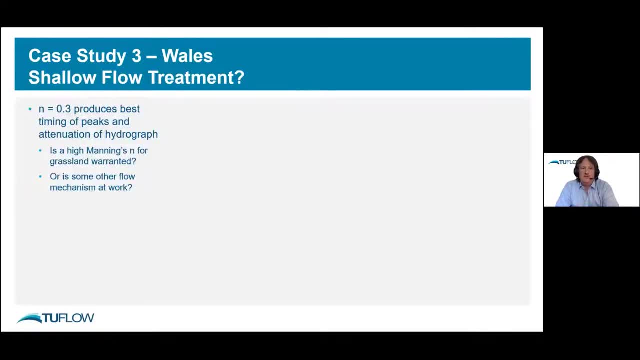 at a higher depth. So it's somewhere in between those. still we're not really getting the attenuation quite correct, so that Manning's value of 0.3 it produces the nicest looking timing and attenuation of that hydrographs. but can you really justify a Manning's end of 0.3 for a grassland? 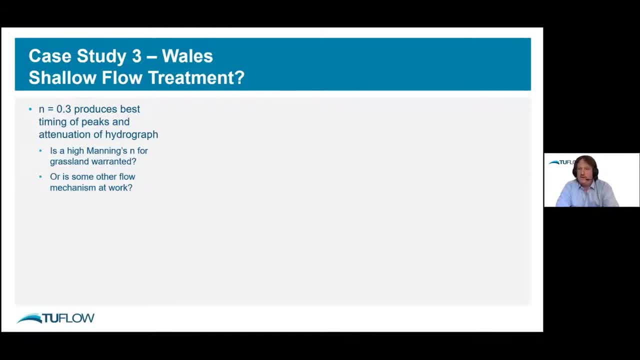 Yeah, I'm not convinced, or maybe there's some other flow mechanism at work. Going back to our hydrology diagrams, you know what we're doing is modelling everything essentially as a surface runoff at this stage, but for this particular catchment, maybe interflow and groundwater. 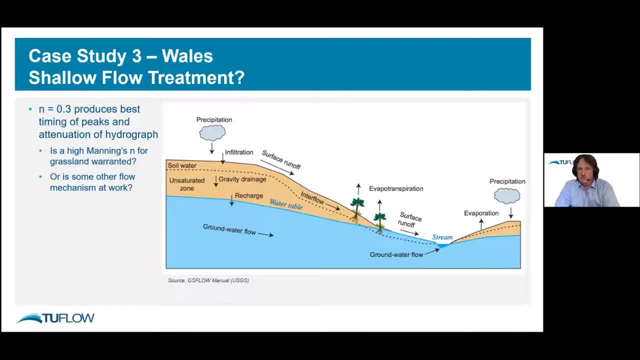 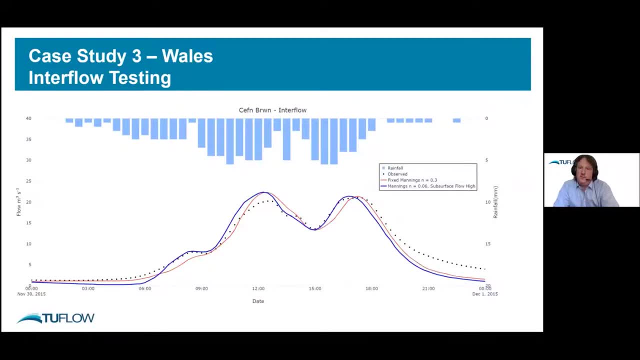 base flow are actually quite important in that hydrograph response. So we tried the same thing with some interflow. so for the 2021 release of 2Flow, we've put in some interflow features so we actually can can apply a depth of interflow and a transmissivity coefficient. 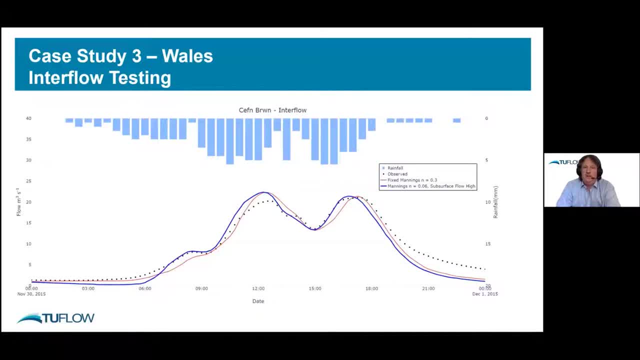 for interflow. So the blue line that's been added there. so red is fixed Manning's at 0.3. the blue there is a Manning's value of fixed Manning's not varying with depth of 0.06, but in this case we've got a 3.8.. 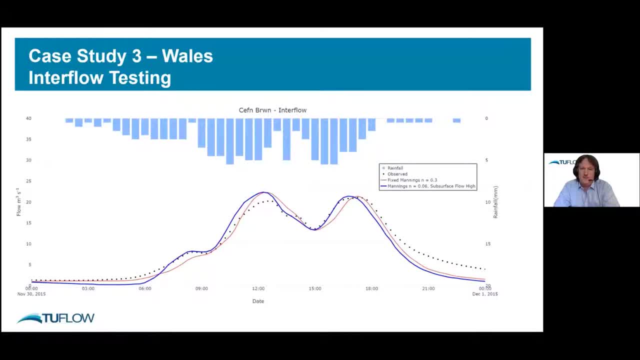 a subsurface or an interflow being applied, and in this case with quite a high transmissivity. so it is actually allowing quite a lot of water to move through that interflow zone. If we keep the mannings the same and look at changing those interflow parameters, we'll start to see that we 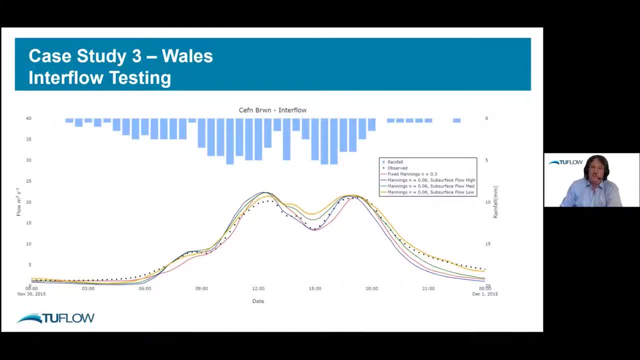 we're slowing that water down and with that last case, there with the lowest transmissivity, we're starting to lose that hydrograph shaping between those two rainfall peaks. but but doing a nicer job on the receding limb. Back to the Agile question: how does it compare? 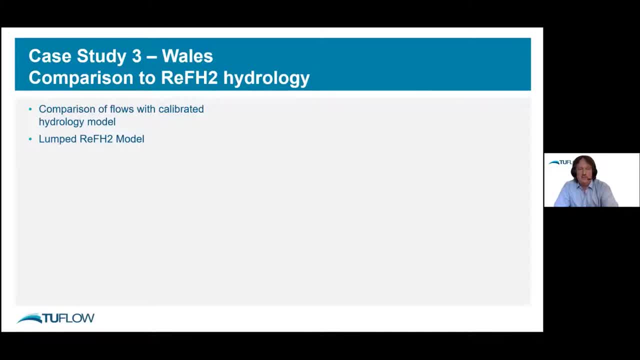 with a calibrated hydrology model- In this case we've compared back to a RefH2 model which has been prepared by my colleague in the UK- so thanks, Duncan- which is a lumped model, so it's a single essential catchment above that gauge and then it produces that flow hydrograph coming off that, In this case the orange. 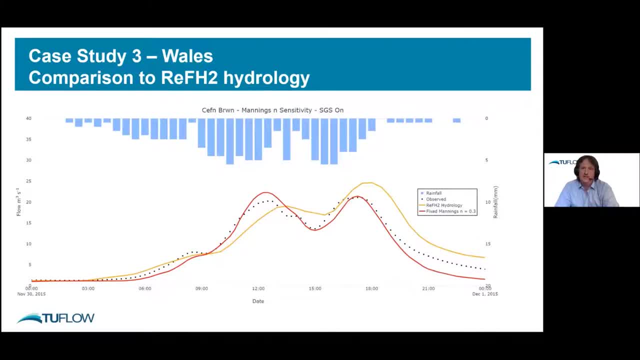 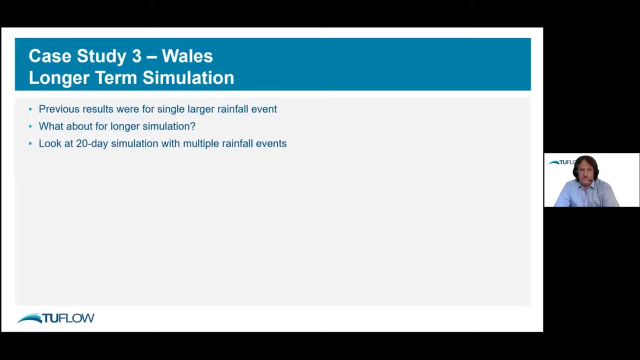 is the RefH2 model and red is the two flow model. In this case I've picked on the fixed mannings value. I think we probably give a nicer shape around the peaks of that, but that was for quite a large rainfall event, even though the rainfall intensities are probably a lot less than what we're. 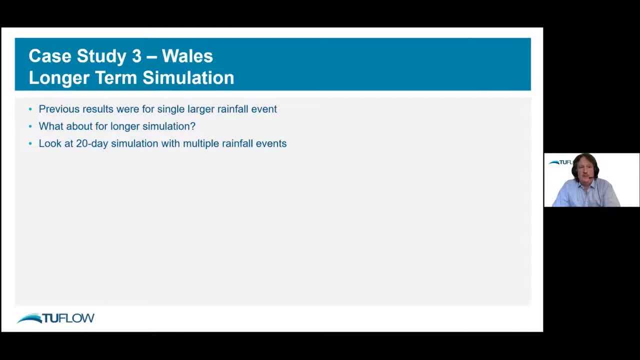 used to seeing here in the east coast of Australia. What about if we look at a longer term simulation? So we we've got quite a lot of data for this catchment. so we looked at a 20-day simulation over a period with multiple rainfall events in there. In this case we've now got the 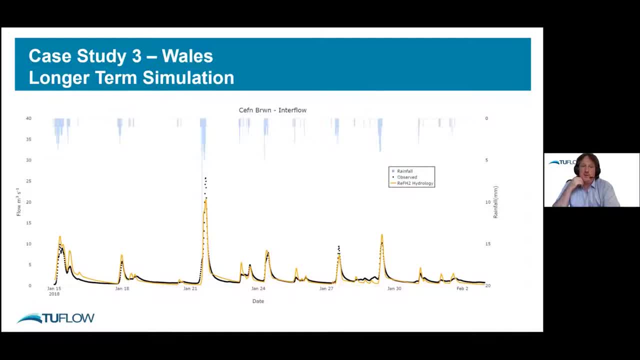 the black dots obviously being the observed data, and we've got the RefH2 hydrology model in there, so it's actually doing a pretty good- um, pretty good- job of capturing those. If we look at that fixed mannings, which I showed you in the same color on the previous 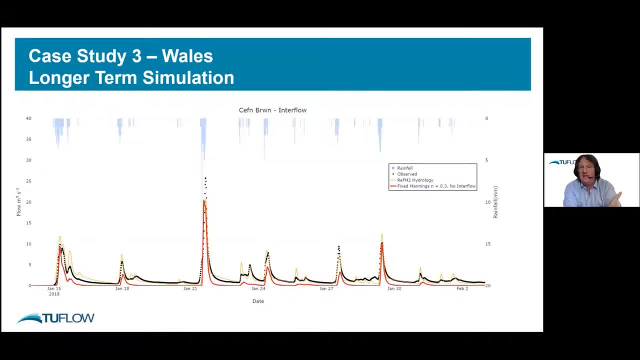 shorter duration of vent where we've got the Webbilianしかregulatory粘 where we were getting a nicer calibration. in this case, with no interflow turned on, we're really not getting a great calibration on those receding limbs, so we're doing a reasonable job of matching. 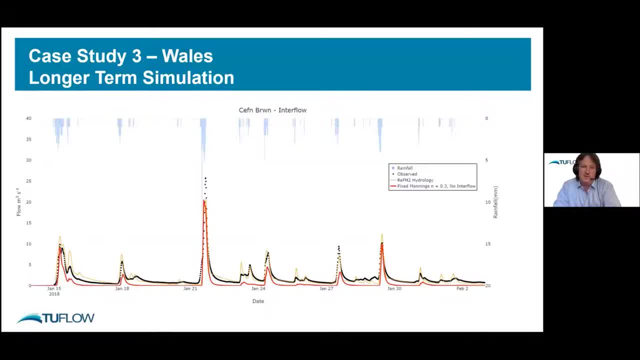 some of the larger peaks, but probably not on the on the smallest peaks and certainly not on the on the receding limbs. the blue class that's just been added now is: is that same manning's value, but with a, an interflow being applied, so a low transmissivity interflow, which is doing quite. 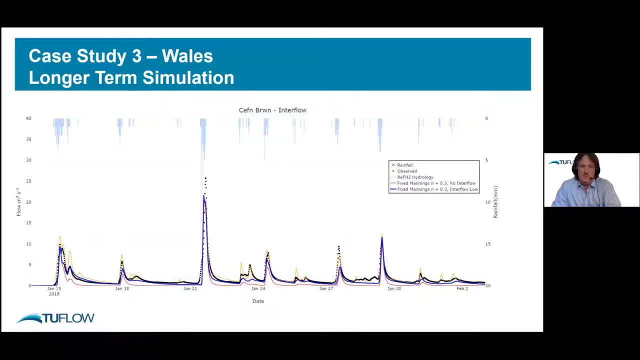 a nice job to matching the shape even throughout the receding limbs and as well as the peaks. and probably moving to something that we're we're a little bit more comfortable with is: is that manning's value of 0.06 and an interflow term turned on? uh, we're getting those smaller. 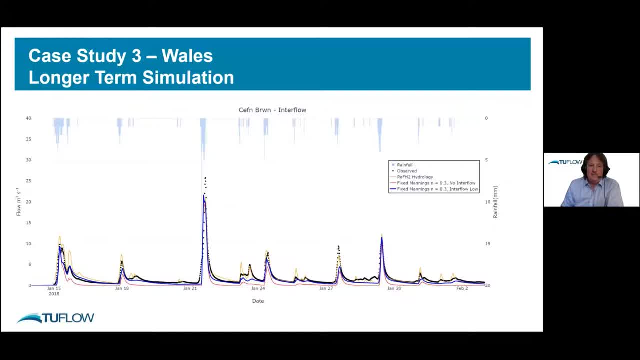 peaks. um. so i think in the previous case, we're starting to miss some of these um small sharp rainfall events that occurred between there. we're not getting some of that um uh response in in the catchment. um, as we move to to um faster interflow, we are starting to just to see those. 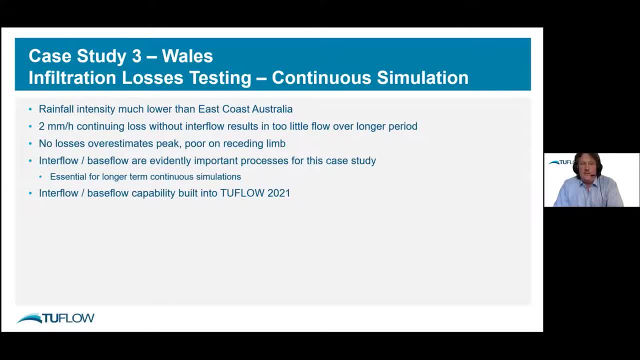 uh responses as well. rainfall intensities are certainly a lot lower than that we expect to see here in eastern australia, which, um, based on the spread of um of the people in this in this webinar, most people actually aren't from eastern australia- um quite quite a low rainfall intensity, um when? 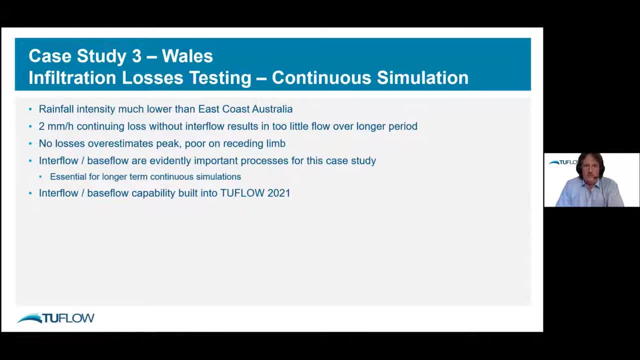 we applied that um continuing loss, um without any interflow. uh, it really did show that uh, there's too little water in in the system over over a longer period. if we do run a case with with a no rainfall soil or excess uh rainfall losses, we overestimate the peaks now but we get a poor um. 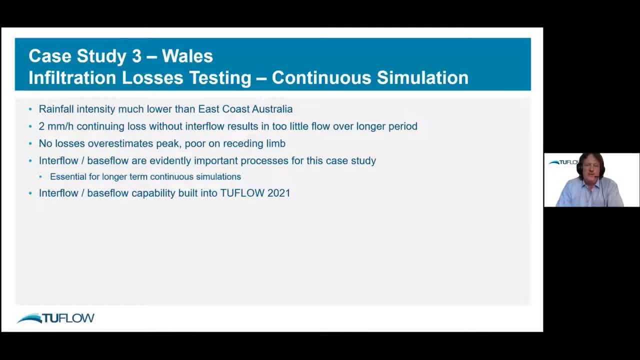 response on the on that receding limb, and so i think for this particular case, interflow base flow components actually pretty important for this um, for this uh, particular case study and probably are essential for that longer term simulation approach. so we have been building those into the 2020 version of two flow. 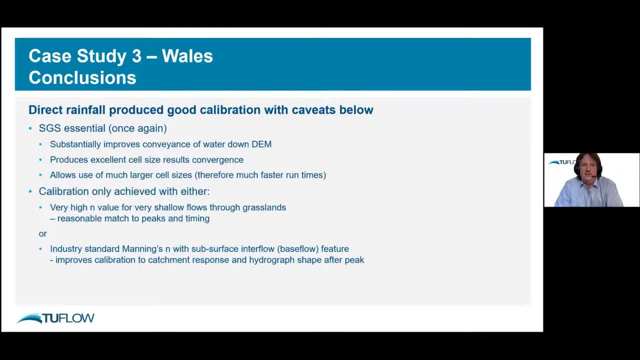 so i think we were able to get a, a good calibration, uh with that, with the caveats of of using sgs again, um, because it really does provide a better uh conveyance, um, for that direct rainfall, good cell size convergence and allows to run with that with course of cell size. but we 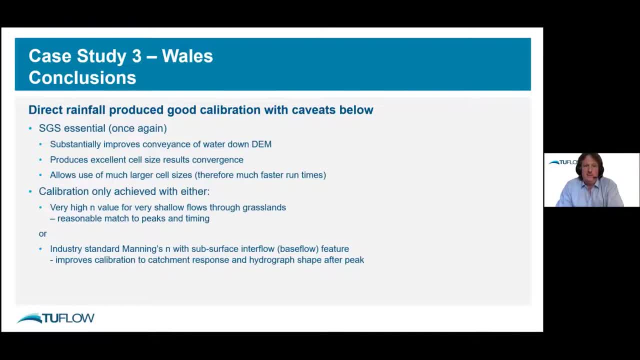 could only get that calibration with either a high manning's end value- um we could get a good match to the to the peaks and timings, um- or using a sort of an industry standing manning's end of six and and turning on some sort of subsurface, uh interflow, in order to get that um slower uh. 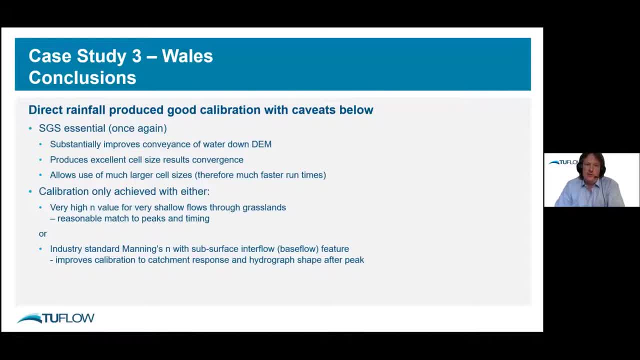 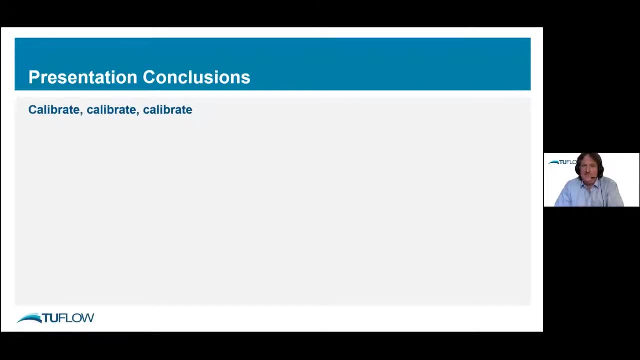 interflow and base flow responses, and that certainly improved the calibration and catchment response, um, after the peaks of the events. in conclusion, i guess, um, as always, um, calibrate, calibrate, calibrate wherever you, wherever you can, and also test, test tests. so, um, you know all of 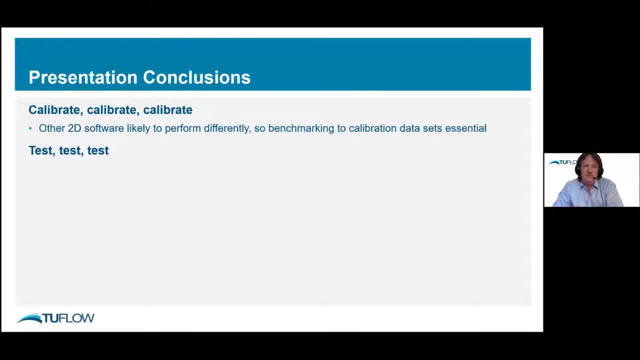 this uh testing was was done with essentially the two for hpc um suites software. so other software is likely to perform differently and have maybe slightly different performance. so that's that's a different um knobs to to turn in order to get um calibration. so so benchmarking and calibration. 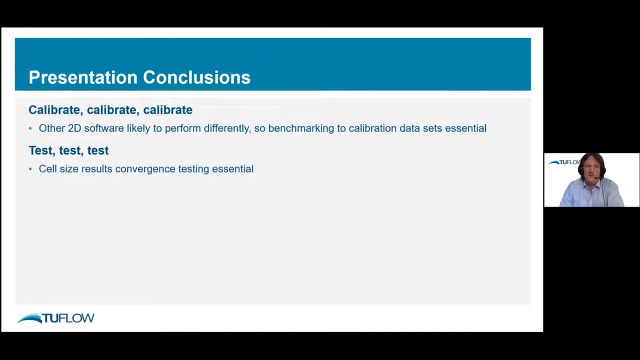 is is really essential. um, and also, you know test, test, test. you know look at testing cell size and and uh, yeah, uh, loss methods, and i didn't uh show any of it today because we didn't have time. you know rainfall interpolation methods where you use a um, you know a tinning or an inverse distance. 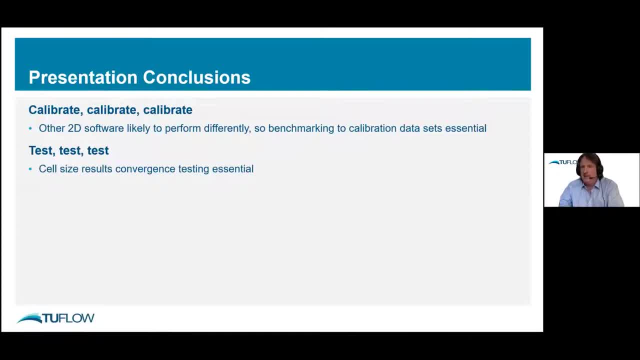 weighting in getting from your point gauge locations to a spatial rainfall across your um catchment. but i think those case studies probably show that that um you can use direct rainfall, um you know, with hpc, as an alternative to traditional hydrology, um, provided that um probably would say that you sgs is pretty key to that um and and depth varying mannings. 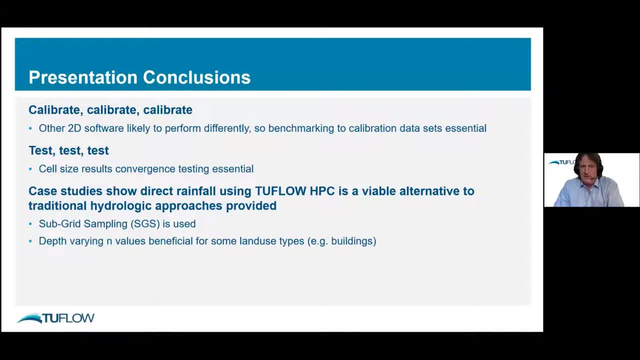 certainly has some benefits, uh, particularly for some of those land use types, um, like buildings, where you'd expect to see a very rapid response, um, at low depth, or where you're going to have to have a very rapid response when rain falling on those buildings, but a different response to to. 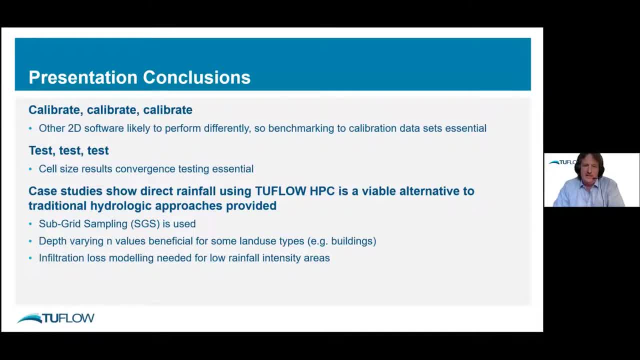 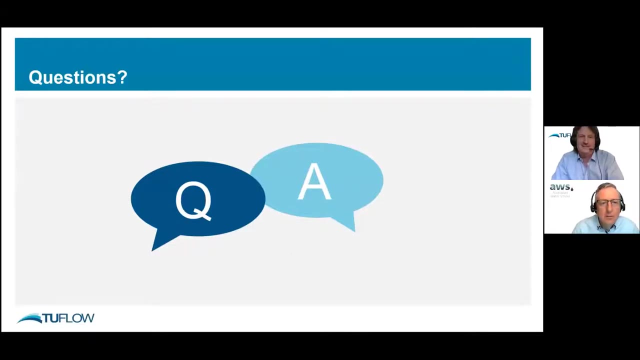 flow throwing through a building and infiltration losses is obviously important, particularly in areas of low rainfall intensity and subsurface or interflow um is probably needed for those low rainfall particularly. we've got those pervious catchments and and also uh longer, uh, longer term simulations. that's probably about all i wanted to say. uh yeah, the quick question. question and answer. 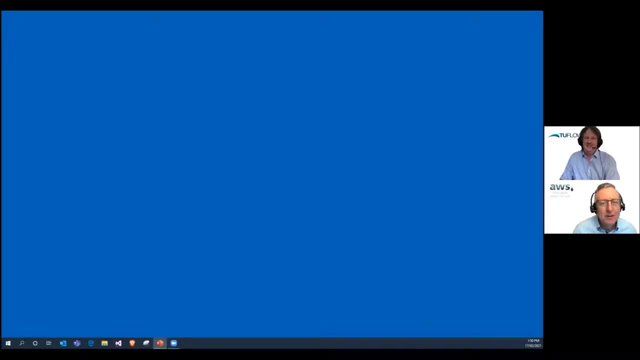 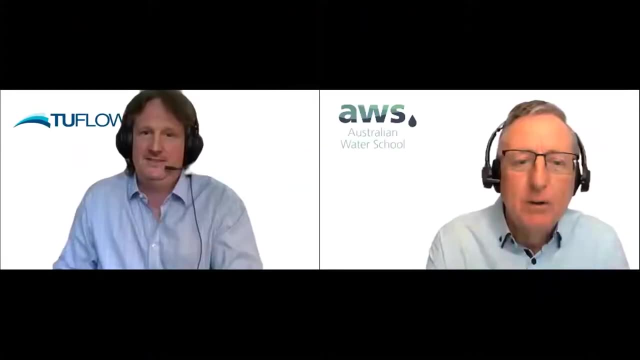 fantastic feast of information about direct rainfall and modeling. i don't know how long, how many times this has been done in the past, but that is covers a lot of ground. the case studies are fantastic and, uh really appreciate the time and efforts coming into this. i want to say bill and 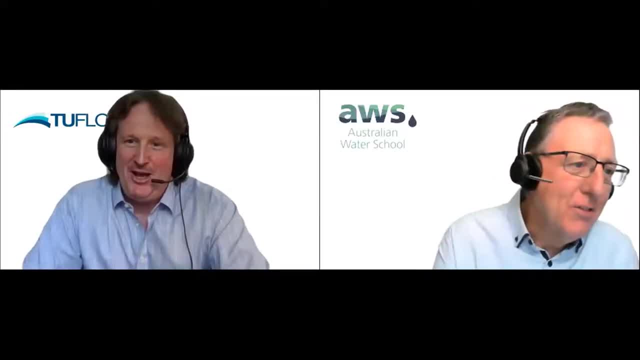 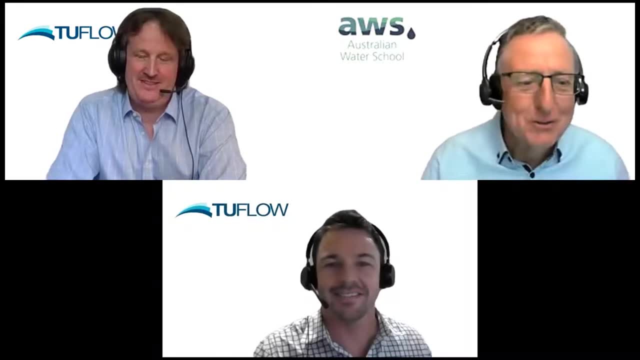 chris have been going flat chat behind the scenes. i don't think they got kind of please, fully unaware of all the questions that have been answered and that the questions are still coming in as far as they're getting answered. yeah, good, good try though, chris. good good, well done bill. 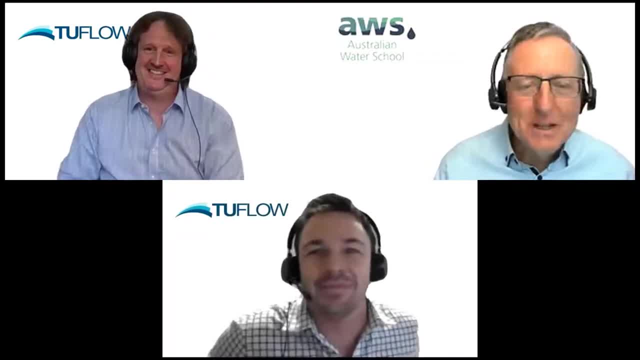 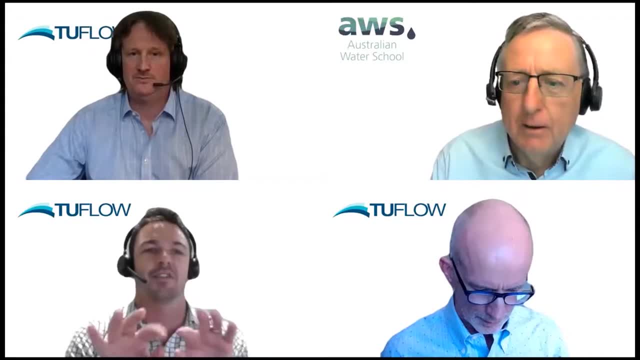 you did all you could do. fingers must be going going hot. um, let's get into this. there were two questions in there where people were asking specific questions land to the models- which i couldn't answer. so i just said: oh look, we'll circle back to this in the question time, do you? 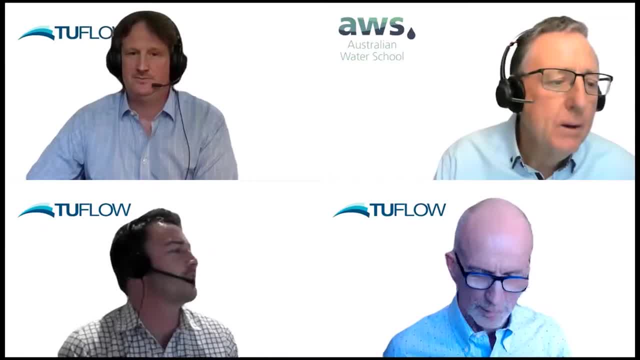 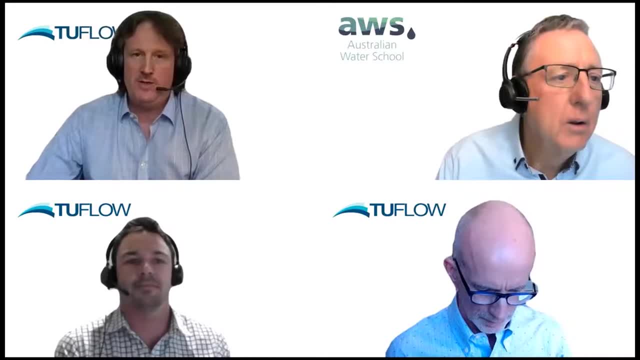 want to pick them up. yeah, yeah, yep, absolutely um. phil. someone asked: were buildings included in the dm for throsby? no, they weren't. they weren't um included as a building pad. yeah, it was actually done at a 10 meter cell resolution. this is this is going back to. you know it was. 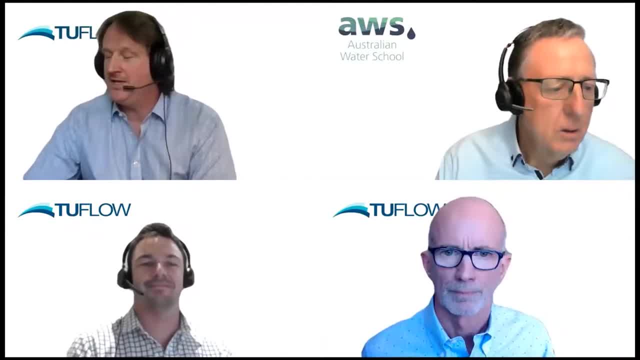 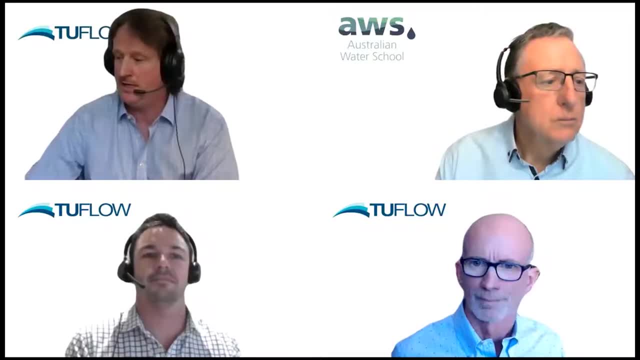 done almost 15 years ago ago now. um, so at that 10 meter resolution, it probably um is a little bit difficult to include those buildings and flow paths in between buildings, which is probably the one of the reasons that we adopted a, an urban block. if we were to do that again now, uh, we would. 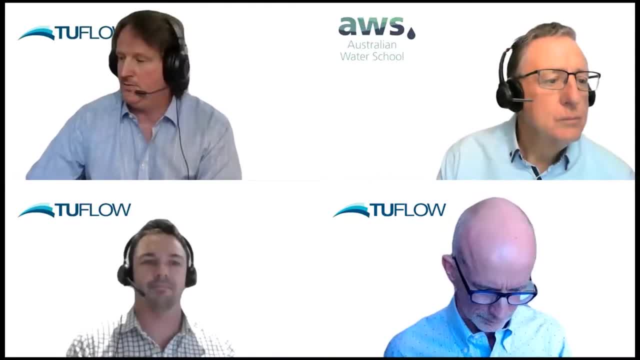 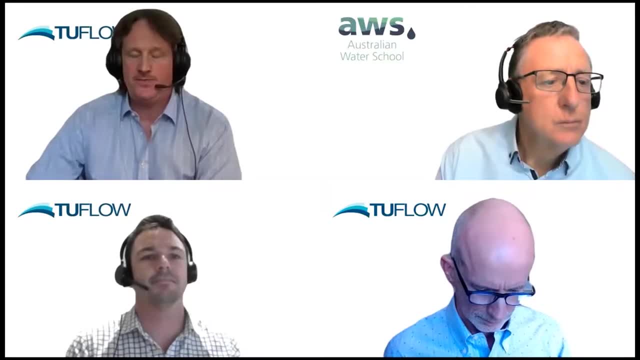 probably run with a much higher resolution uh version of that model and- and we actually are using that model- the same model for looking at um, whether or not we need to use 1d um in those urban channels- uh, so whether we can actually get away with with 2d um cells across. 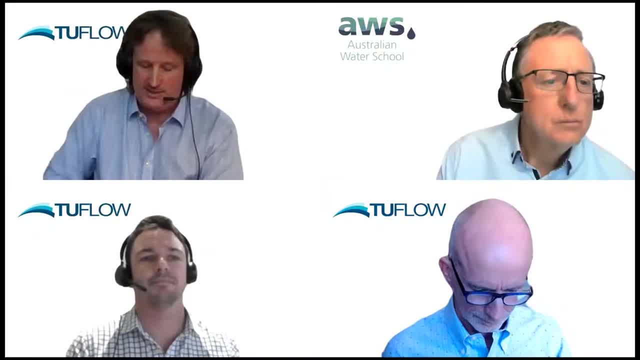 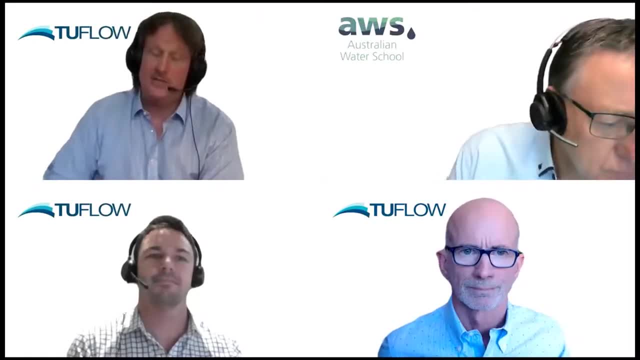 those, um those, those channels which are obviously not necessarily aligned to to the cell direction and things like that, um, where we're running it with a with a range of cell sizes that are much smaller, which would probably allow us to look at different building approaches. very good, um the. 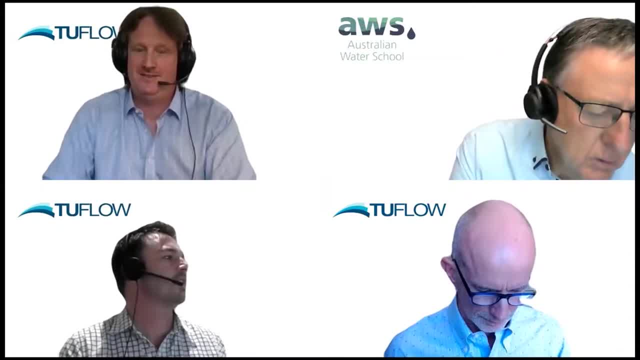 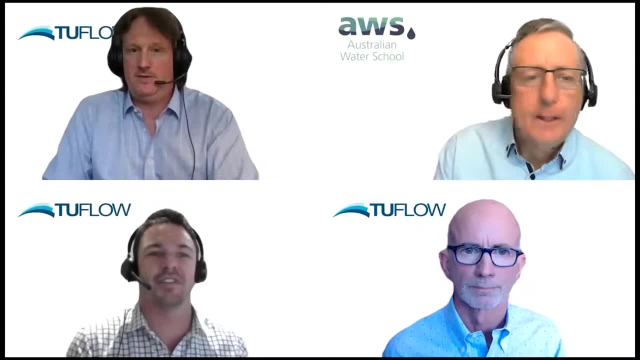 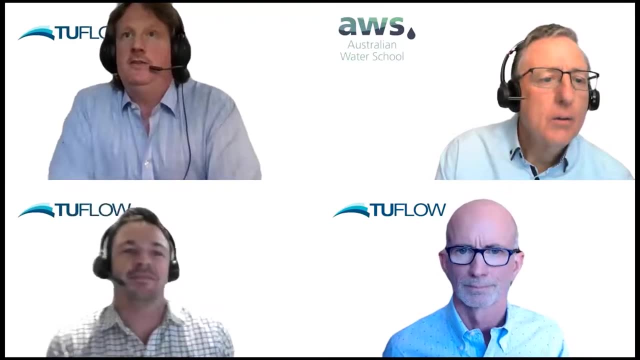 other one, which i um delayed to the question answer time was: what size sgs was adopted for this study? can you remember what the resolution of the dms were that fed into those models, because that would in turn define the sgs resolution? yeah, we were. you can um overwrite the? um the? 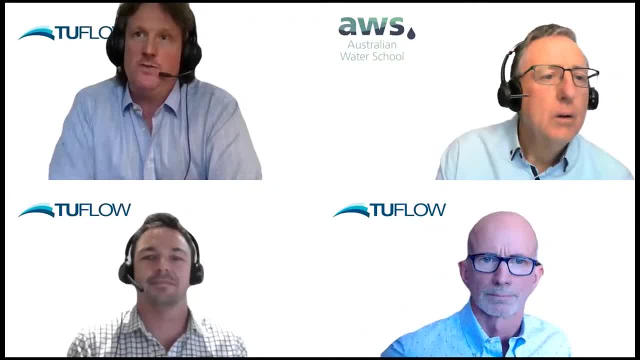 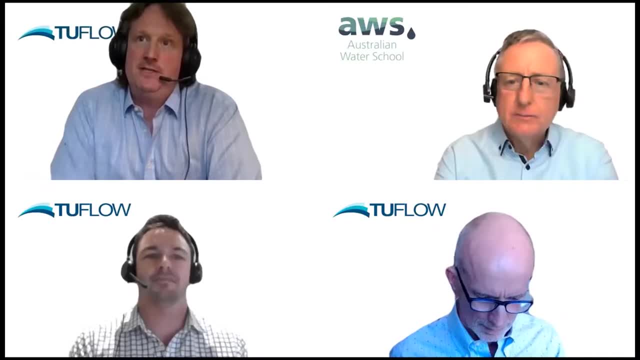 subgrid sampling distance. um, you know to to use a user set value, or if you don't, it's, it's essentially using the? um, the dem elevation. uh, there actually was a range of different cell sizes for different data sets. so i think that for most of the south johnson river that was at 10 meter. 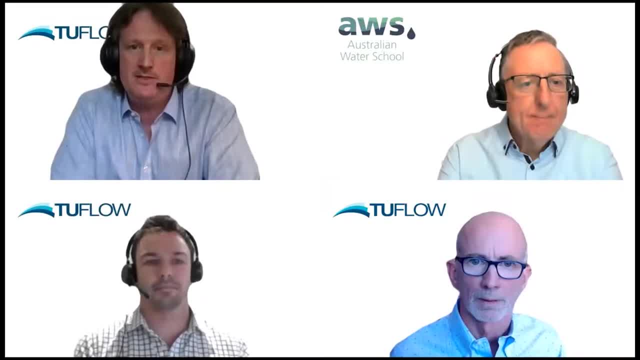 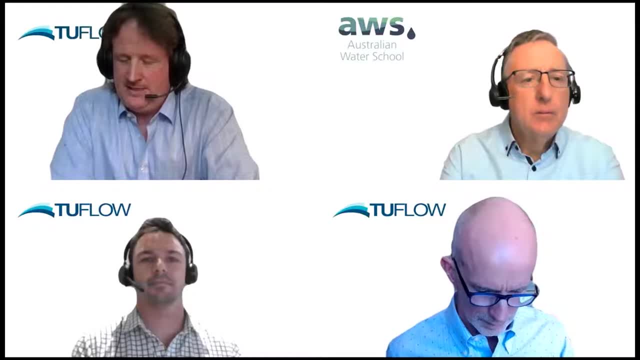 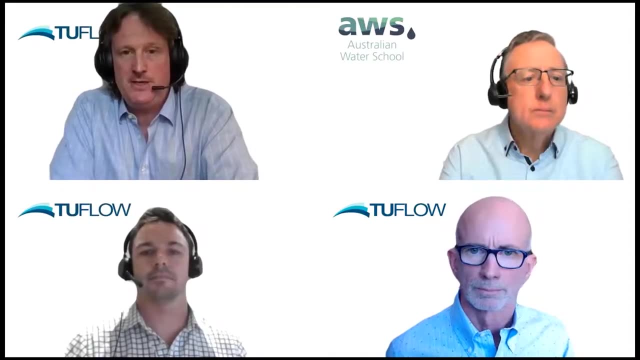 resolution. parts of it- actually the lower part, i think- was at five meter resolution. so we were using that um for that sampling distance, um, for the throsby, i believe, the dem elevation, um, there actually is a really nice tin uh of that, but i think it was exported at maybe a two meter elevation uh, so i think that's probably. 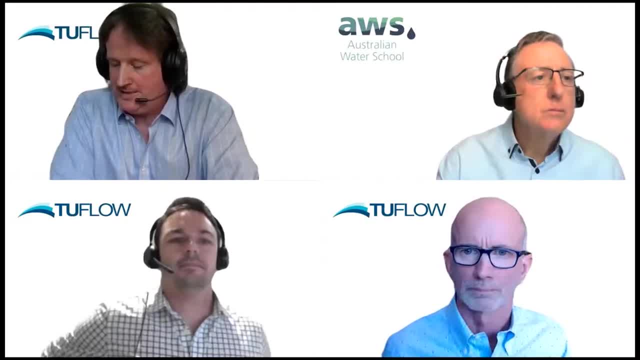 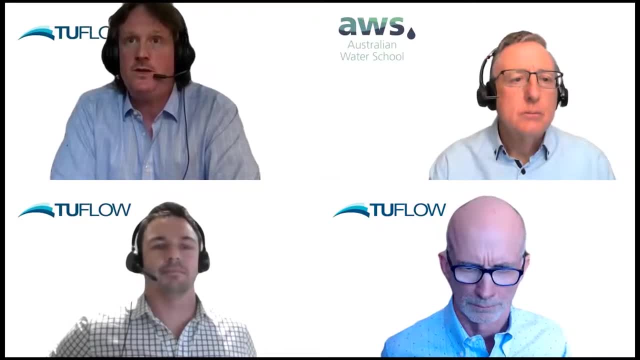 what was used as a sampling distance um and for the welsh uh test case, there was actually uh two different um cell sizes. there were parts of it that were covered with a 10, 10 meter um resolution, uh dem, but the majority of it actually was a two meter resolution. so that's what would have been. 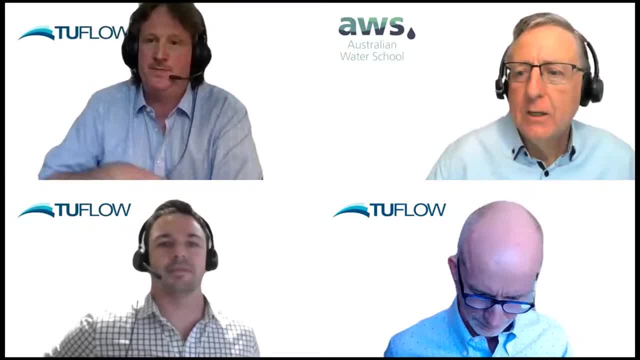 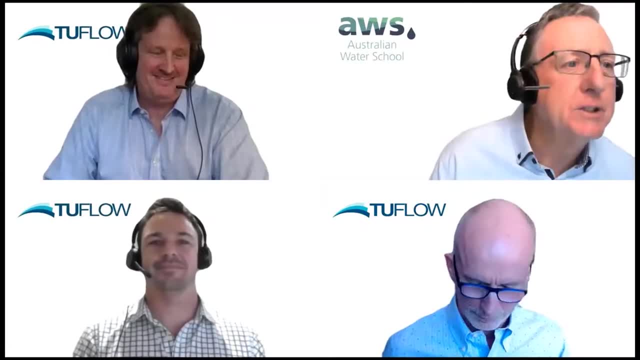 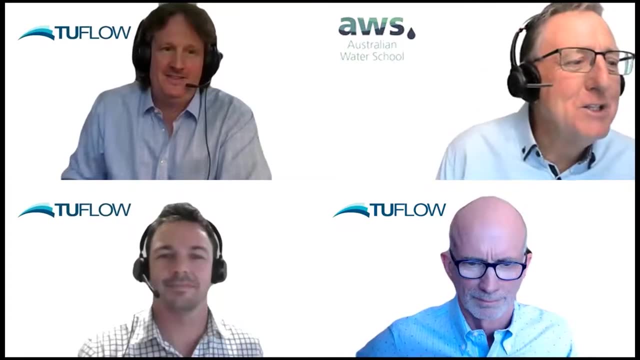 used as that sampling, uh, distance, yep, excellent, good, okay, well, um, let's get cracking. it's obvious that from the 70 plus probably 80 questions, 70 plus questions anyway, uh, that, uh, we've struck you forward here with a lot of people, so, all right, let's get cracking. do you have any tips in applying direct rainfall to ungauged? 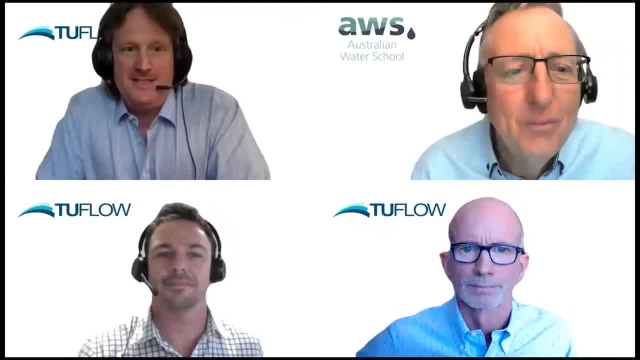 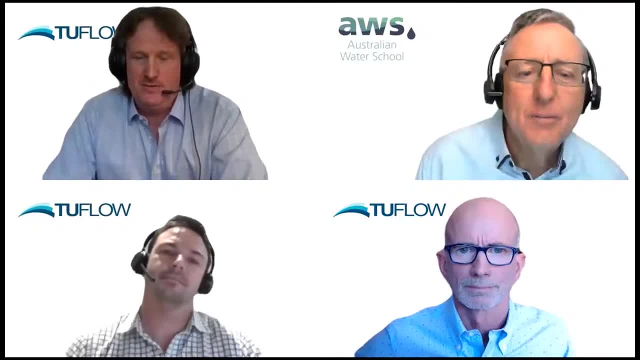 catchments. i mean, i guess, uh, the the point that rob made is is probably valid- that, uh, calibrating of all models is important. even if you had a hydrology model, that where you had um, that uh, that type of catchment, ungauged catchment, you'd probably be looking at sensitivity testing your. 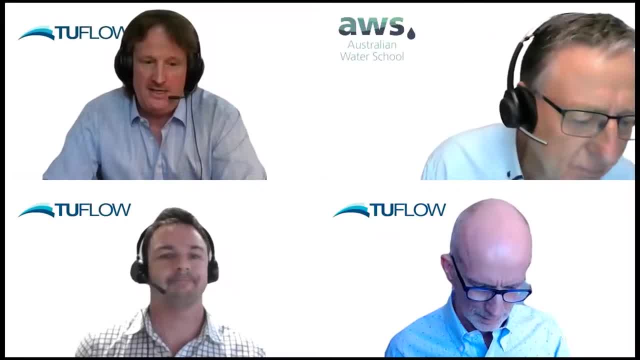 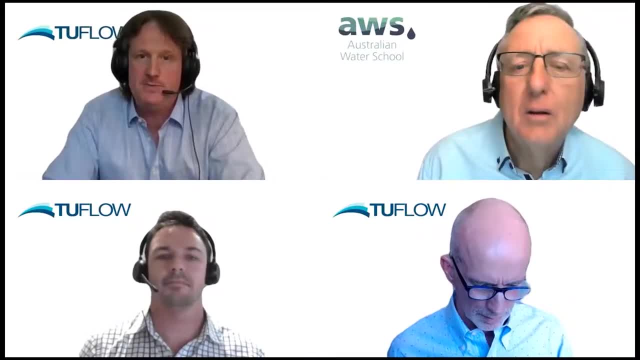 parameters and seeing how, how it- uh, how your model would work. so i think that's probably a good way to look at how your model performs with air. i think the same thing would go for, um, you know, a direct rainfall modeling. if you don't have that data to calibrate, i think it's probably pretty important. 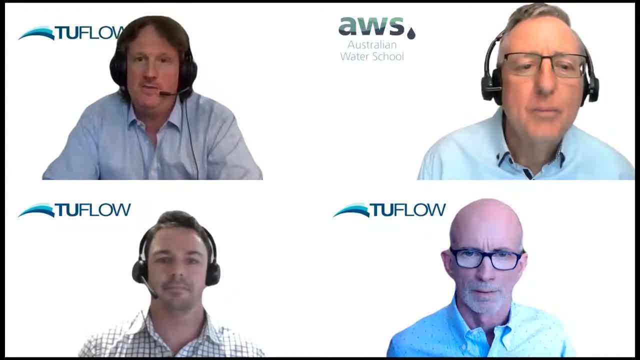 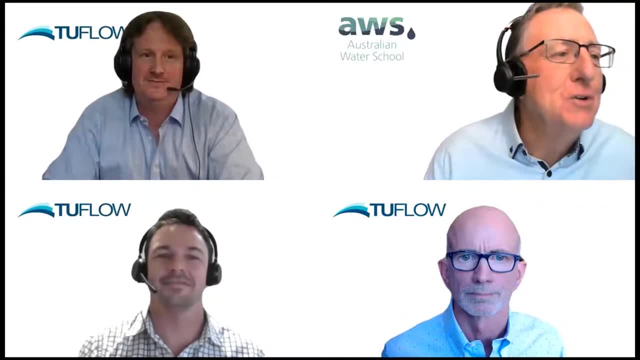 to get a feel for how, how sensitive your model is to the various parameters that you're, um you know, changing to in order to calibrate a model. steven. steven, you says, drawing from your test model merchant mentioned earlier, does it imply it is better to adopt rainfall on grid? 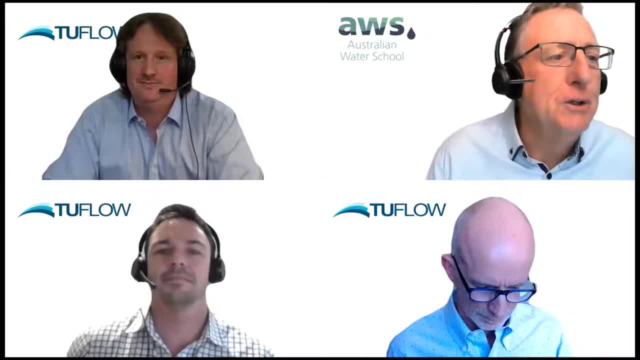 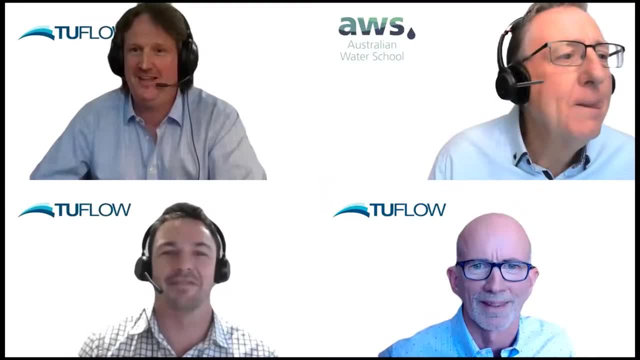 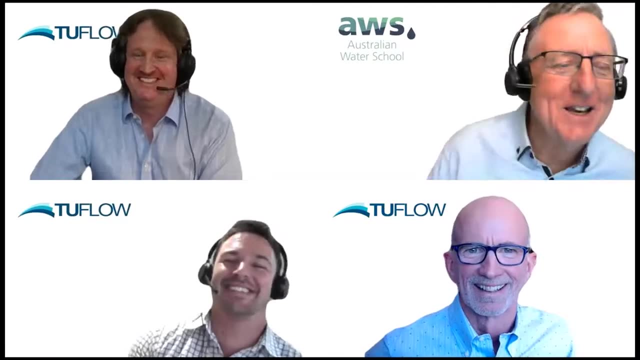 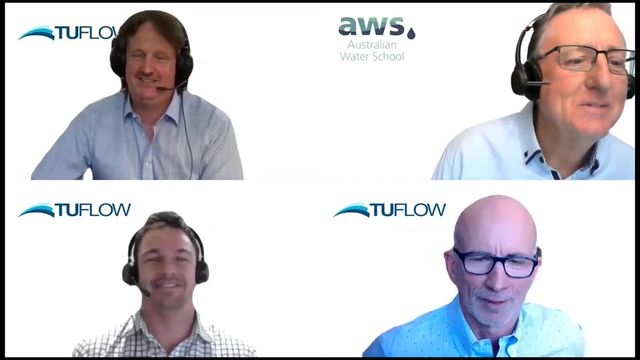 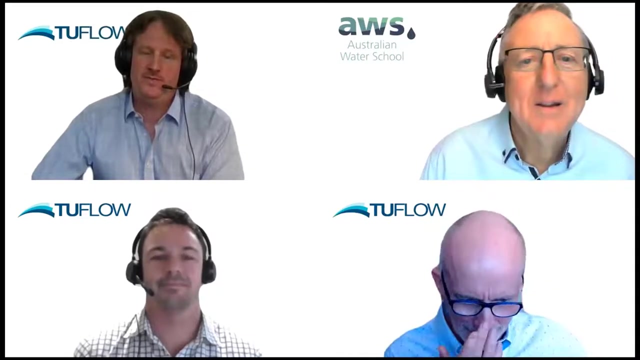 approach in an ungauged catchment than a traditional lumped catchment. hydrology approach: more of an ungauged catchment. the old-school way of doing that is by doing more of a forced down to like a five metre cell size. 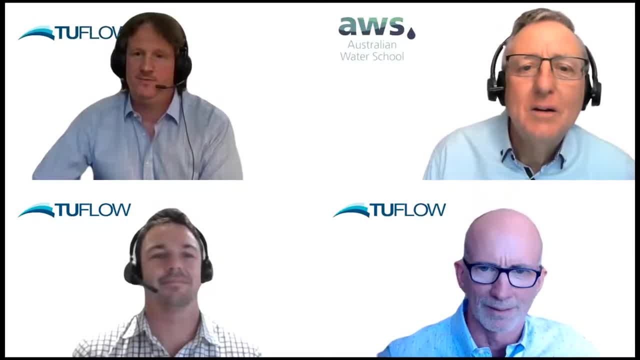 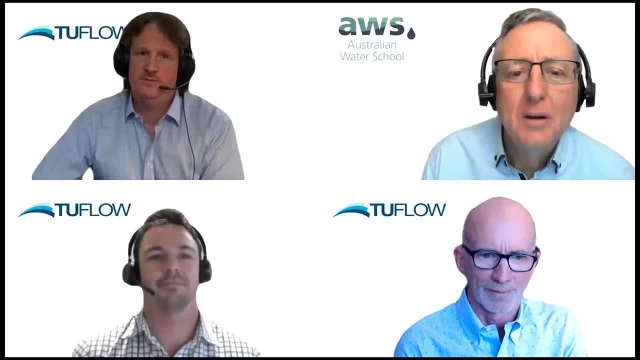 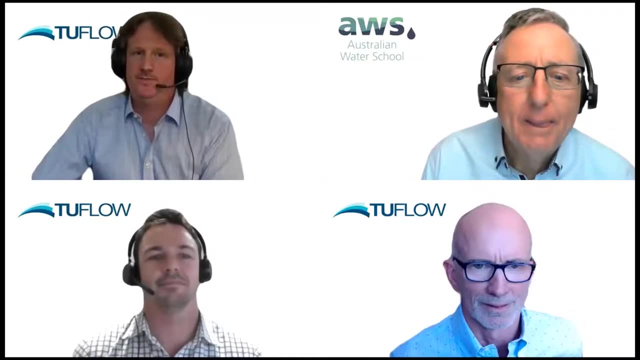 you can get consistent hydrographs of maybe a hundred metre cell size, which totally changes the run times by orders and orders of magnitude. So you can now feasibly consider doing this, I believe, to deal with all the hydrographs and all the meaningful events that AONR 2019 require. 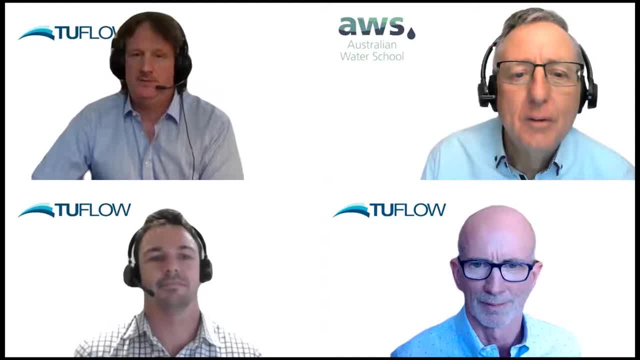 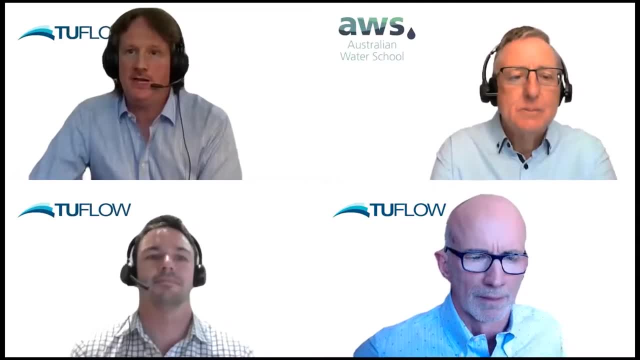 especially with cloud infrastructure. And yeah, there's lots of really opening up. And I guess the other thing, Bill, is with a quad tree. you can include coarser cells at the upper catchment and still get a good hydrologic response off those. 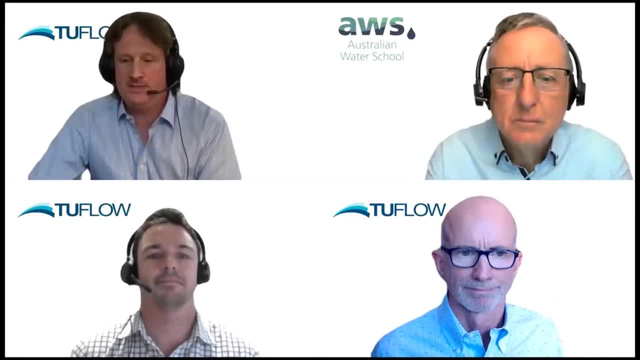 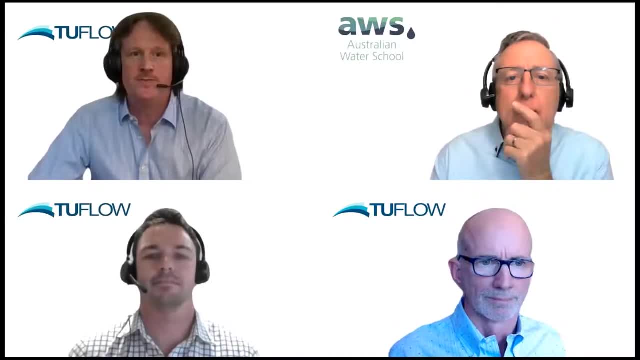 and have higher resolution cells in the areas, the lower areas, where you want the high resolution hazard mapping and things like that. So that's certainly possible as well, Absolutely, yeah, All right, this next one from Parshin. Should we choose what method to use, case by case? 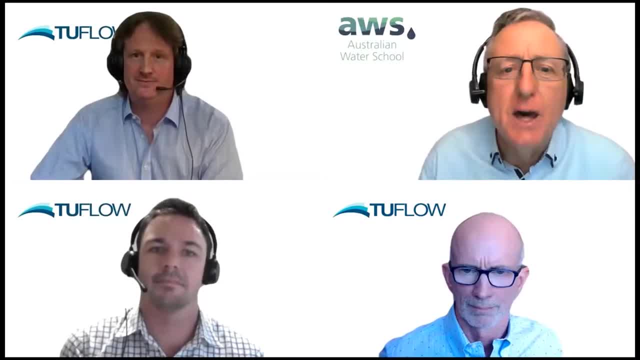 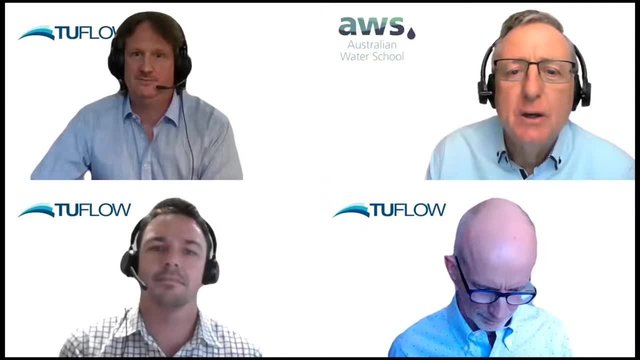 One of the pros of direct rainfall comes hand in hand with a con, and that is that omitting hydrology modelling, which then warrants extensively more simulations that cover various durations, which, in Australia, each of them comes with 10 temporal patterns. 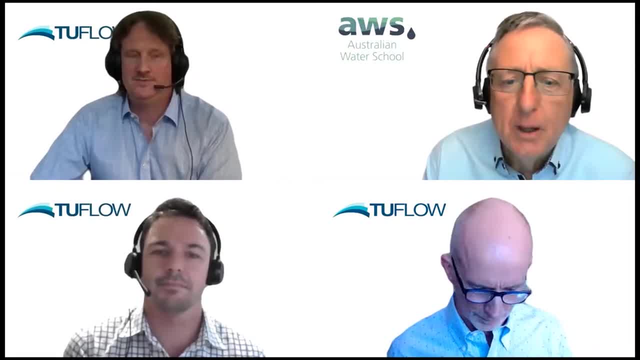 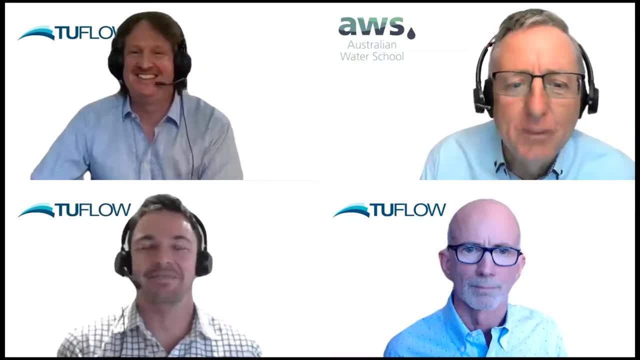 I won't read the whole thing, but should we choose what method to use case by case? Yes, over you, Chris. Yeah, Simple answer. yes, Okay, done with that, Michael. no, Ruby Vandree, have you compared it to other solvers? 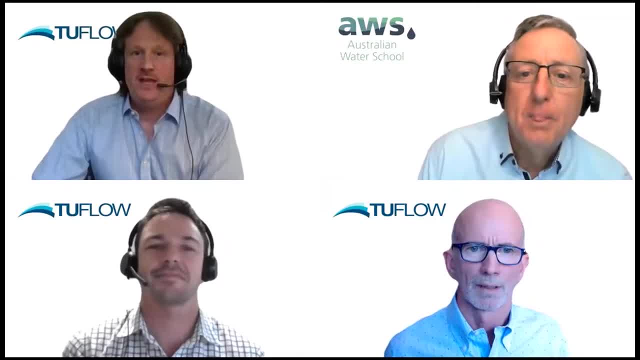 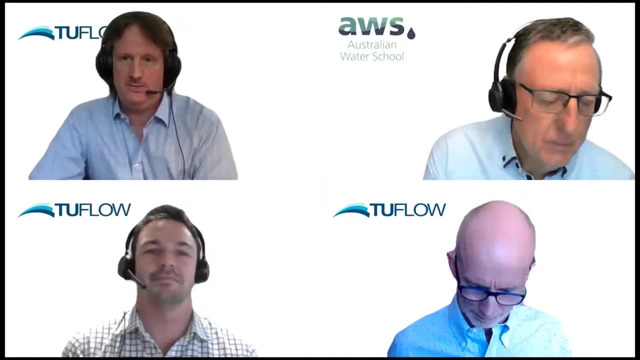 ie finite volume versus finite difference. I guess the original test case, which was the Throsby test case, was done on a finite difference and we did see a pretty consistent result across there. So an implicit finite difference compared to the Tufo HPC. 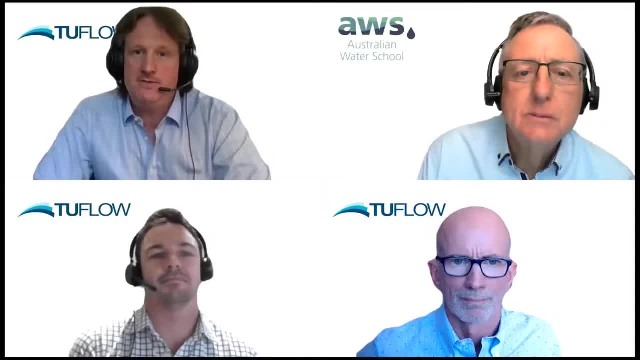 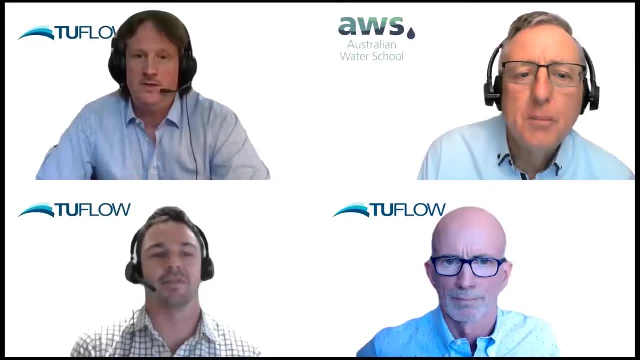 which is a finite volume solver, And we did see pretty consistent results across there with exactly the same inputs and cell sizes and things like that. We did see that. I might add to that as well, actually, The work that Phil just presented on the Johnson River catchment. 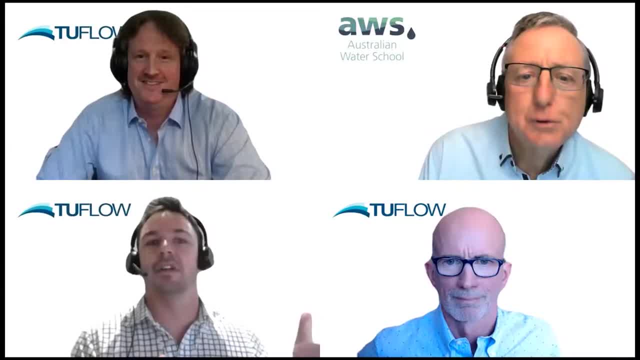 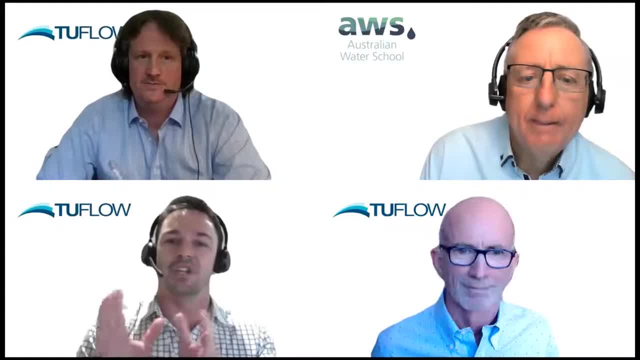 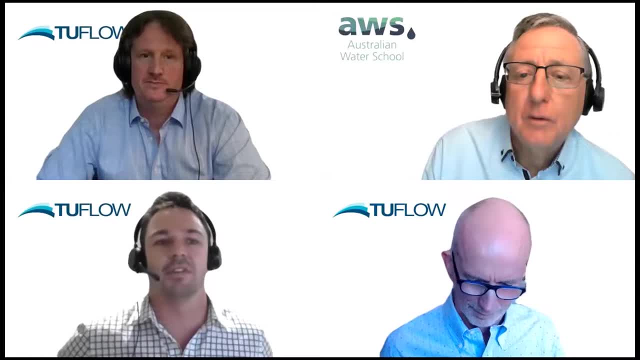 which Tufo Classic is finite difference. GPU or HPC is finite volume. I ended up just going across to the finite volume solution for the simple fact it was quicker because I could run on a GPU card. But at the end of the day, 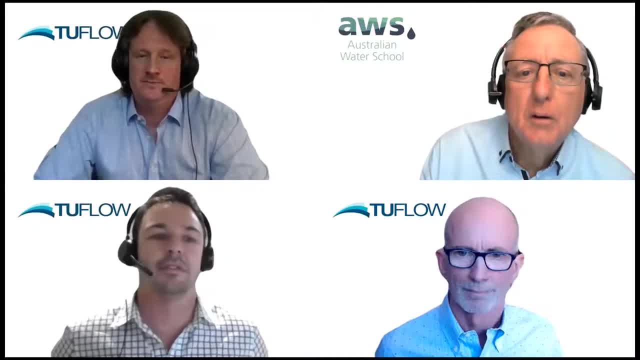 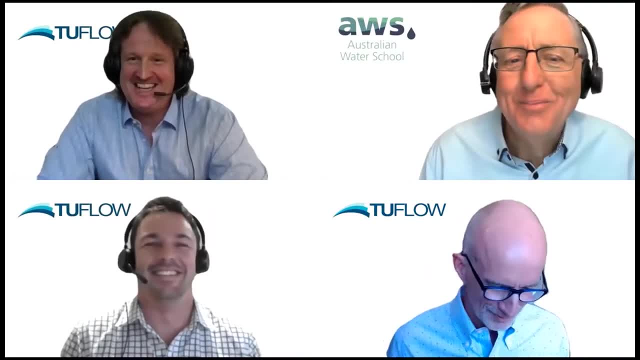 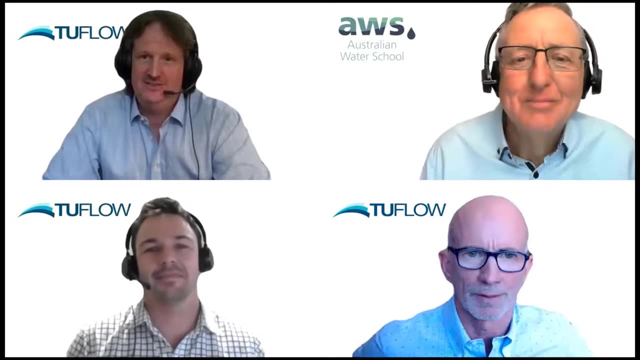 the results are actually pretty comparable. Blimble, Tuflo 21 be released. 21 be available. I'll answer that correctly. We're aiming for August And there will be a beta. I mean, all this functionality is actually already in there. 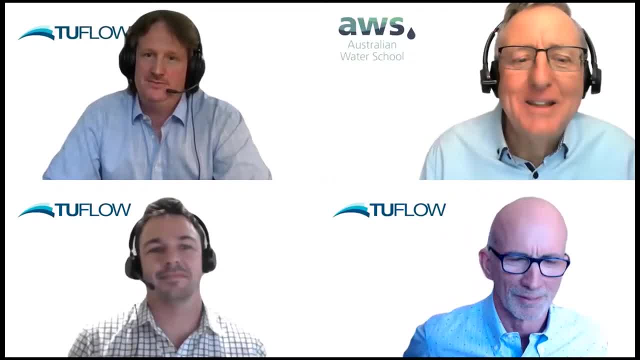 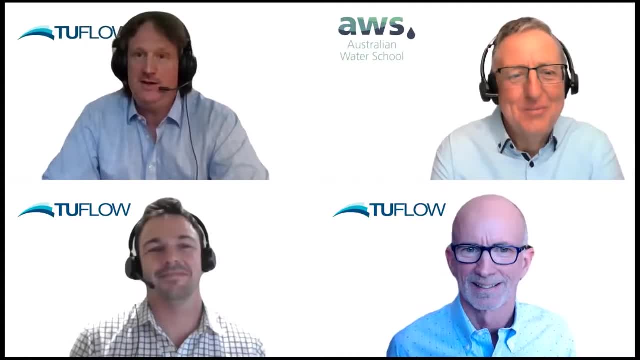 It's about when we press the stop button. Sean, do I have a viewer? Yeah, that's certainly what we're aiming towards. We've still got a fair bit of testing and things like that to do. Obviously, we want to make sure. 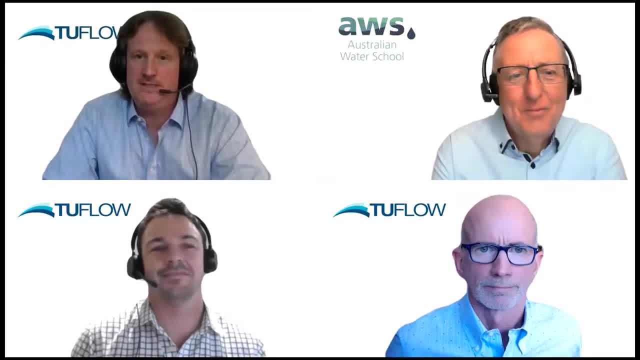 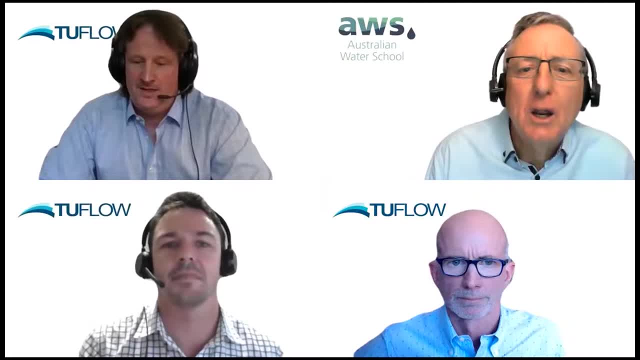 that it's doing all the right things before we release it. That's great. How are you using what depth to filter out shallow surface flow? I guess, once again, that's probably a case-by-case one. It probably depends a little bit. on the purpose of the modelling. If you're doing direct rainfall modelling of that South Johnson with very coarse cell sizes, big rural floodplains, you're probably going to have a different cut-off depth than you would for a high-resolution urban model. 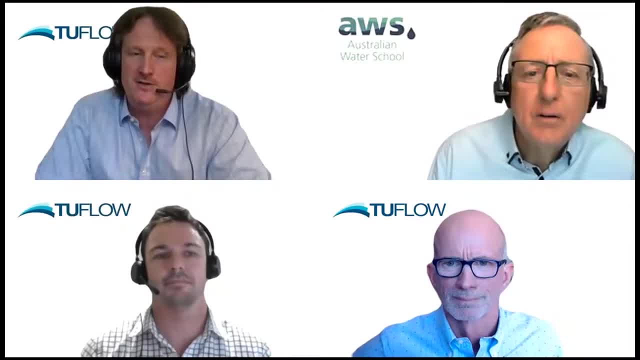 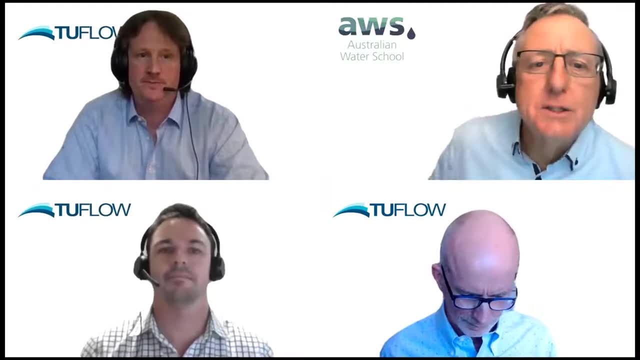 where you're looking at flows down streets and things like that. So yeah, that probably is a little bit of a case-by-case basis. Sure, Enos asks: what was the time step for the study? What was the study's time resolution? 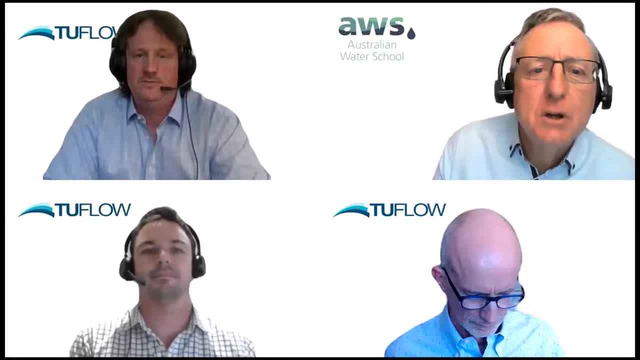 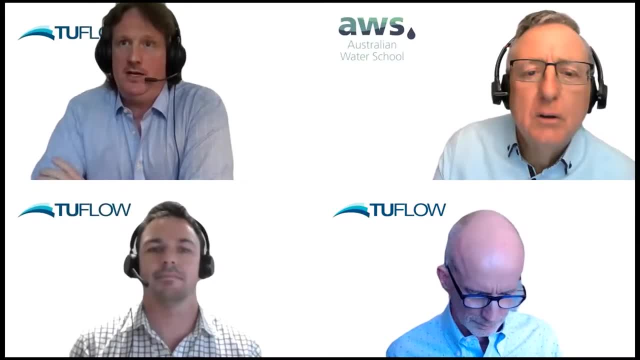 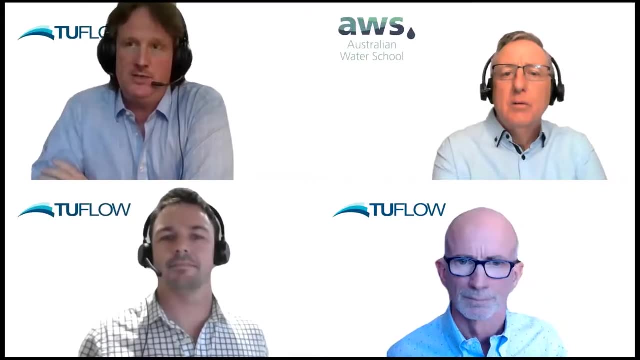 and which infiltration method was used. In terms of the time stepping, with the exception of the initial the Throsby original staff, which was using a fixed time step, the rest of them were all using 2-4 HPC, which is adaptive time stepping. 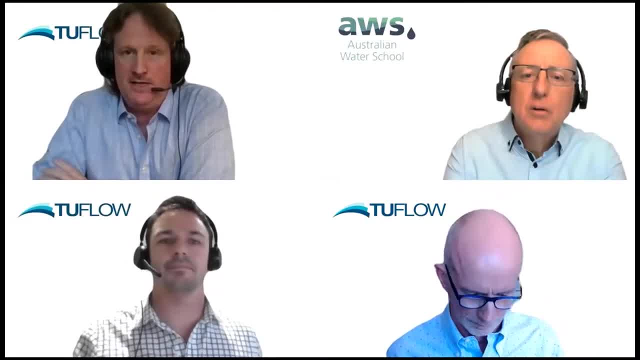 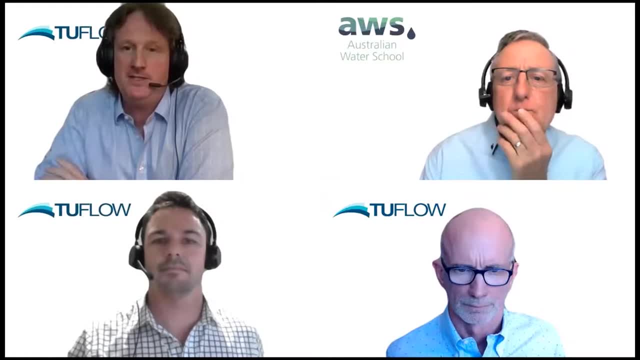 So it's looking at depths of water and velocities and also a diffusivity term to work out what each time step should be Okay. So it varied throughout the simulation, So obviously in periods where there was less water around, 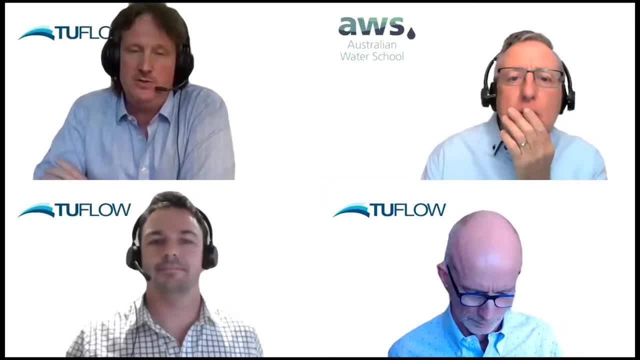 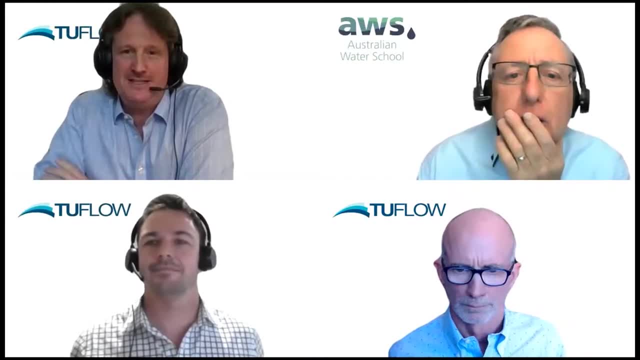 it would pick a time step that's larger, but after a heavy burst of rainfall it will slow that down. Sorry, Enos, I forgot the second part of that question. Yeah, I just pushed it across to answer it and I don't know where it went. 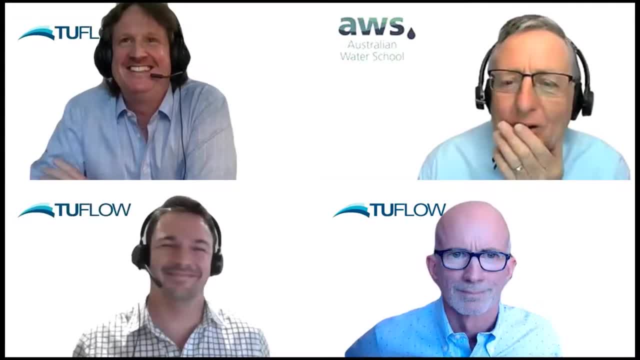 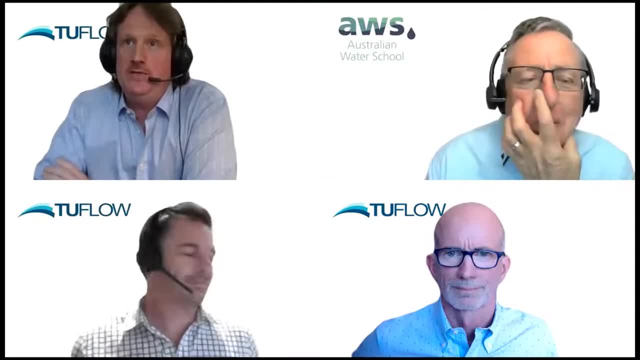 Sorry about that Memory like a sieve. No, that's all right. Oh, no, no, I can't find it in the Oh which infiltration loss methods were used. That's it For the South Johnson. we did look at green-amped Horton. 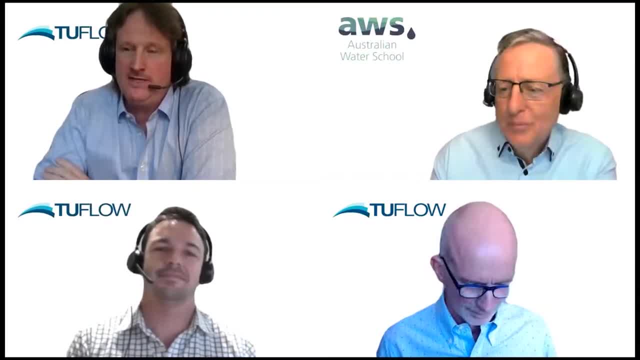 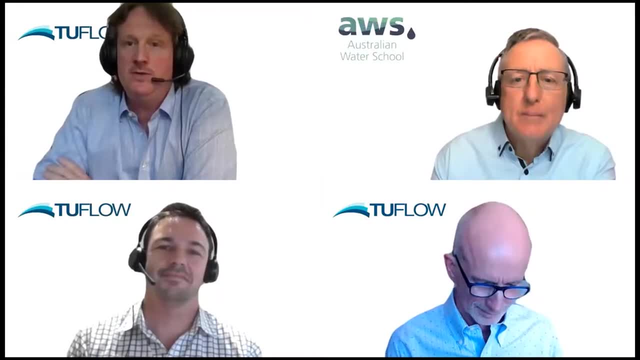 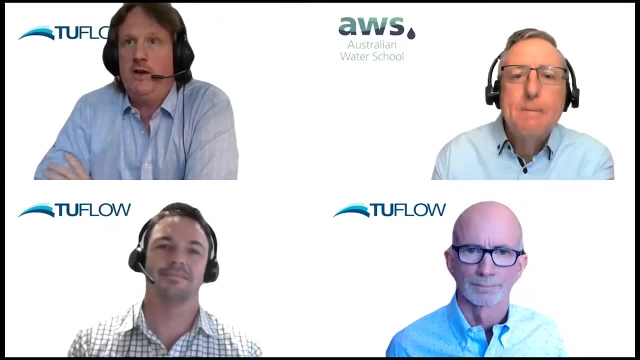 and continuing loss and also rainfall excess. But for the other ones- I think for that Welch test case we were using just a simple continuing loss method and the same for the Throsby, the urban catchment. We're actually using the same loss parameters. was originally used in the original hydrology model, which I think was 2 millimetres per hour as well as a continuing loss. But that did actually vary across the different land use types. So you know, for example, roads would have a high fraction, impervious on those. 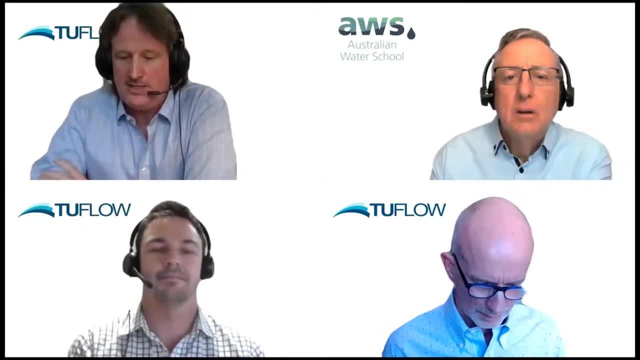 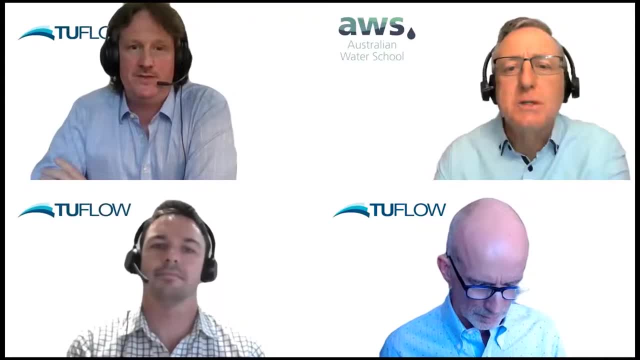 So default, 2 millimetre per hour loss, but a fraction impervious being set based on the land use type. Kundan asks: Hi Philip, what was the grid size and model runtime for the Newcastle model? 10 metre model cell size. 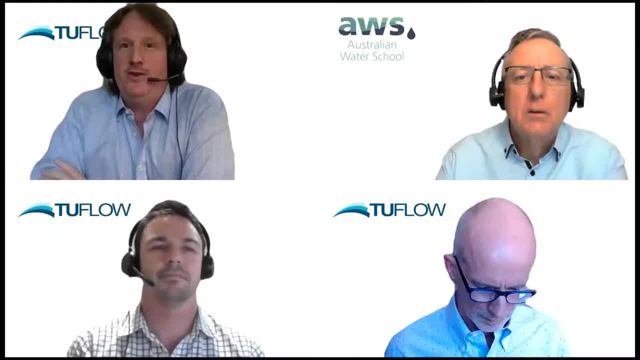 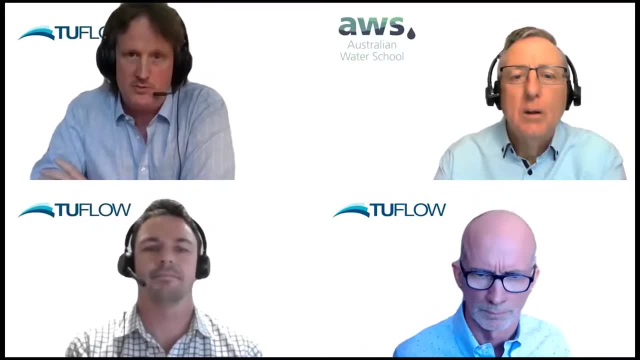 And it was, I think, about 30 minutes. We did do a lot of cell size testing of that but I think for that 10 metre model it's about 30 minutes to run that model with a coupled 1D as well across that catchment area. 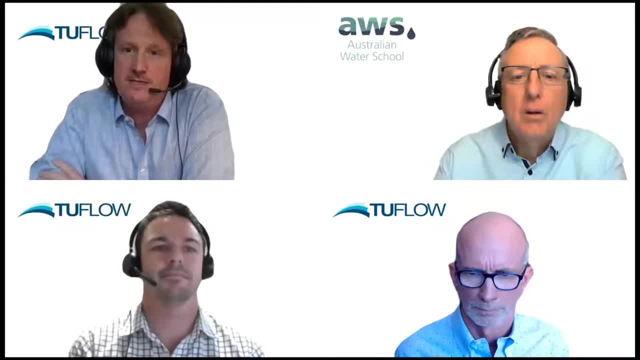 I can't recall off the top of my head how many 100,000 cells were in there, but it's a reasonable size catchment at 10 metres. Yeah, Ashwin says. I may have confused myself. Could you please elaborate? 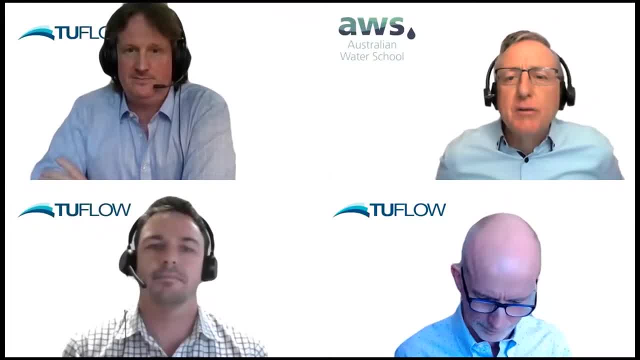 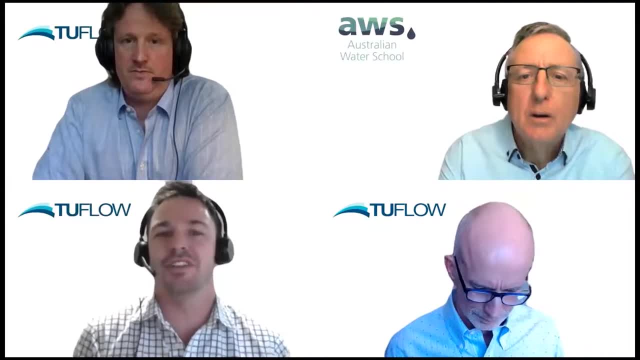 One is using a 2D grid, synonymous with using direct rainfall. That's not a necessity, Right? You can use direct rainfall, direct rainfall with a 2D grid, solver or, if you'd prefer, to use a hydrology model. 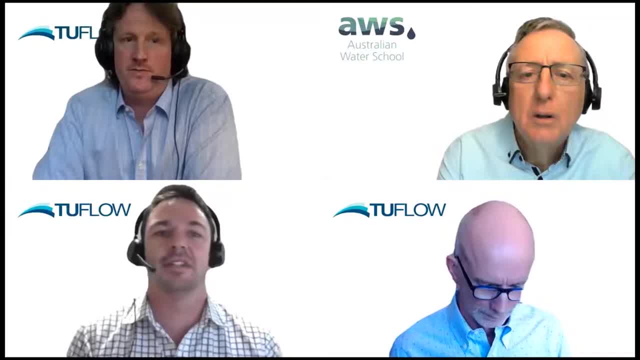 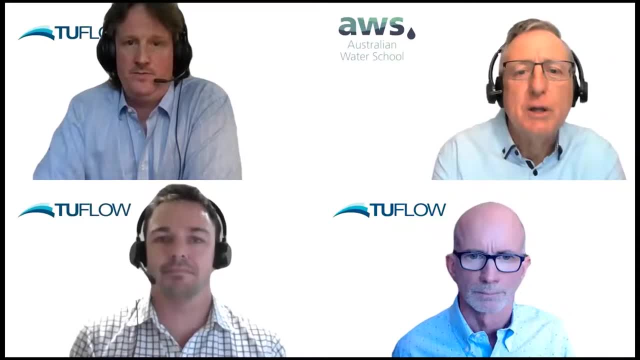 you could pull the flows from that hydrology model to put into the 2D grid solver. So probably answer number two: is it possible to use direct rainfall without using 2D grid? Absolutely, The answer is yes to that. So there's another module in 2Flow. 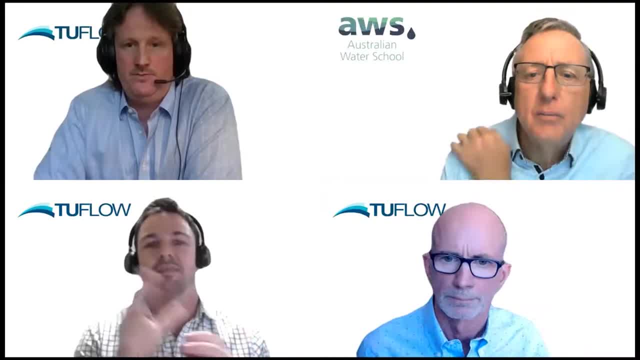 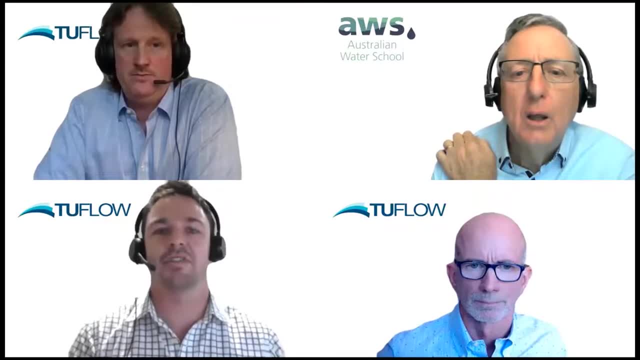 which allows for you to vary your cell sizes spatially. So it's analogous to a flexible mesh, I guess- And yeah, absolutely, You can use direct rainfall In a mesh. And thirdly, how can you accurately represent catchment flow? 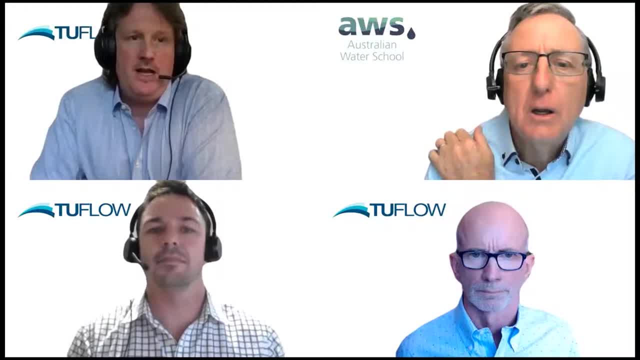 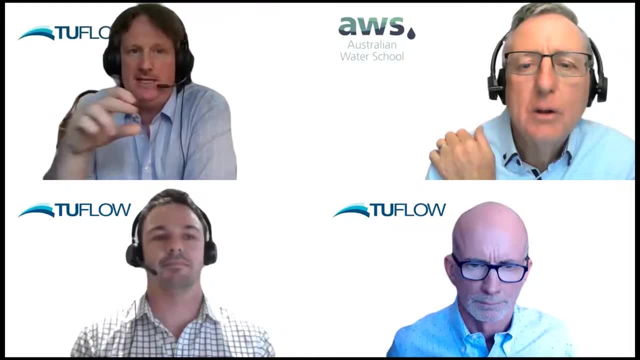 without using a 2D grid that captures cell by cell flow. I mean, I guess that's going back to a hydrology type model where you've got either a lumped or a semi-distributed hydrology model where you break it down into catchments. 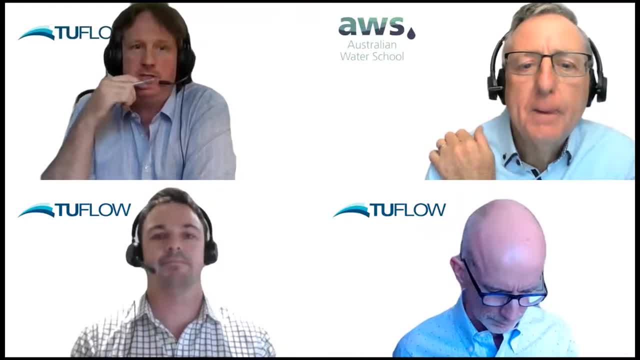 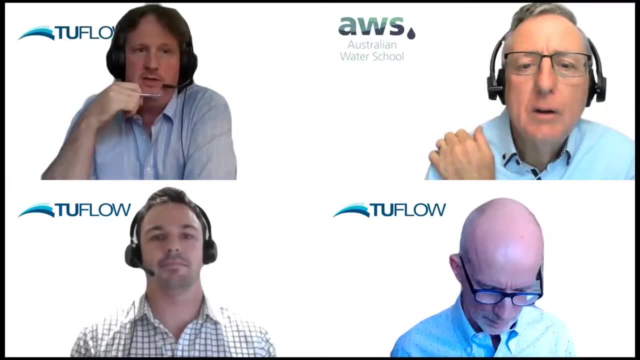 and get your flows out of that hydrologic model to do that And then the resolution that you're able to do that depends on the resolution that you break your hydrologic model down into That. the original the test case had about 200 sub-catchments in there. 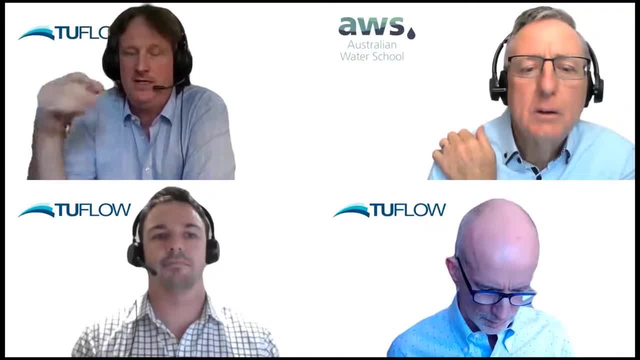 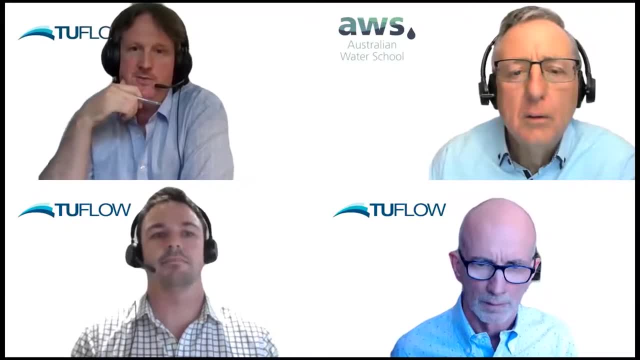 So we're getting quite a good breakdown of flows throughout that, Whereas I think for the South Johnson River, even though it was a much larger catchment area, that model was probably broken down into about 30 or so sub-catchments. He goes on to say: 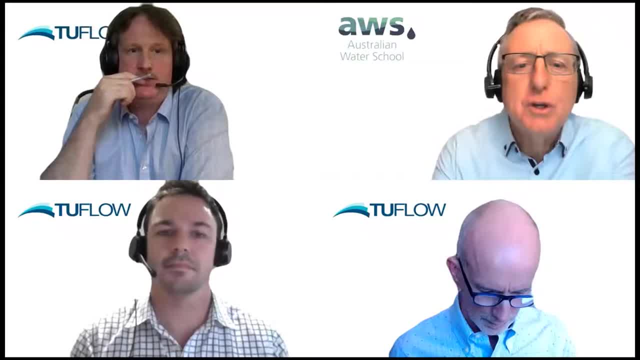 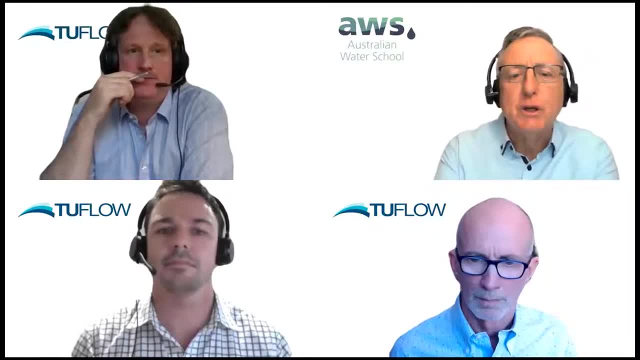 while Ashwin is answering this question. while peak flows from hydrologic models may be similar, it surely can't pick up the changes in flow as accurately as a 2D grid when considering smaller time steps. Sometimes yes, sometimes no When it comes to hydrologic modeling. 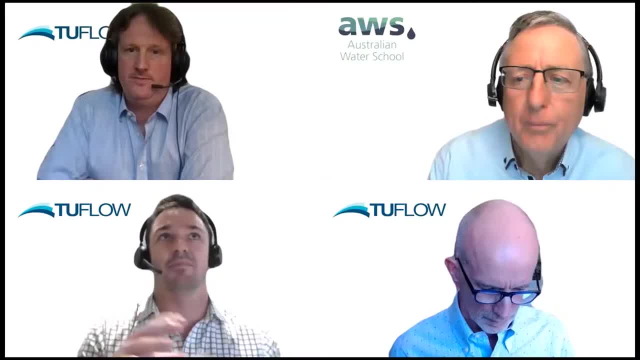 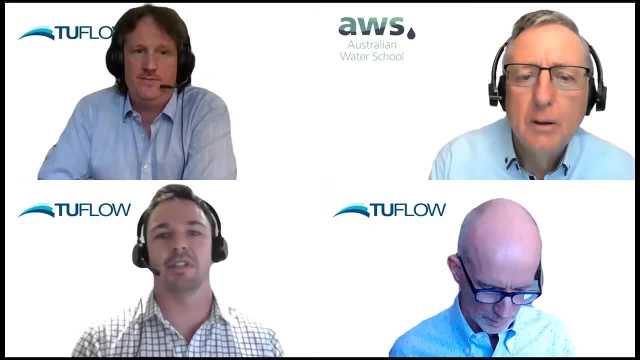 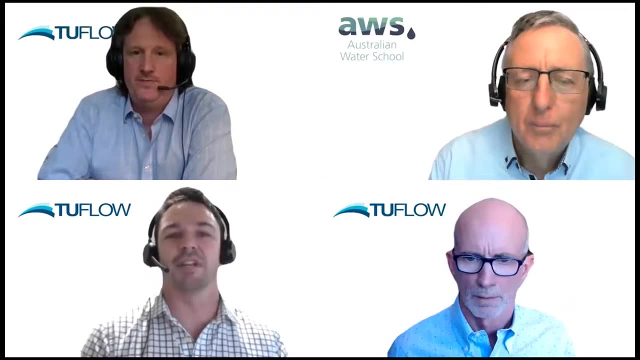 you're lumping your uncertainty more broadly within your sub-catchment parameterization, So sometimes it works out really well. Other times it's a bit more challenging. It doesn't work, but under those situations often it's indicative of your sub-catchments. 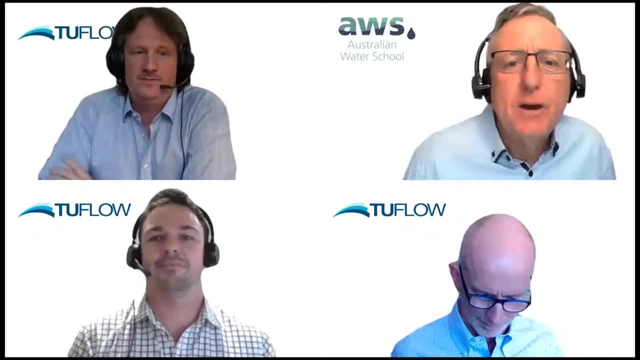 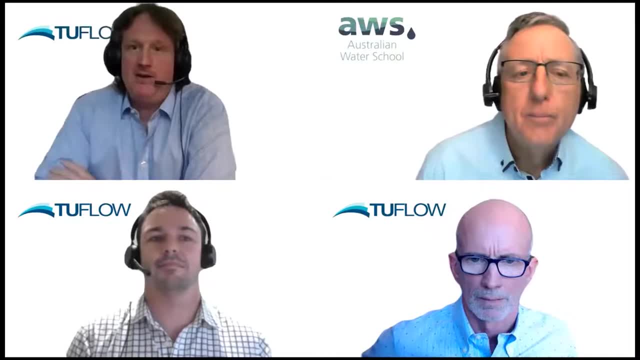 not being delineated at a fine-off resolution. Basil has asked: how does the rainfall on a dry model grid treat it? Once you've started, once you get rainfall on a dry grid, that grid cell will then become wet to account for that rainfall. 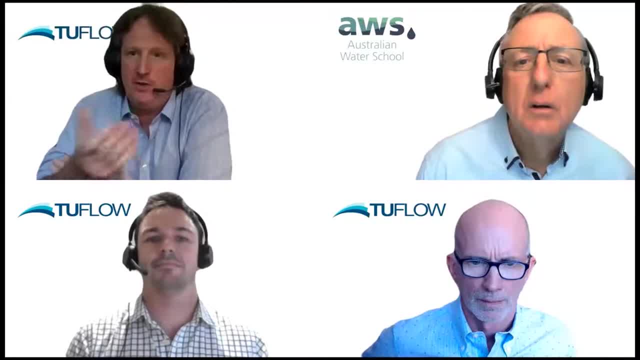 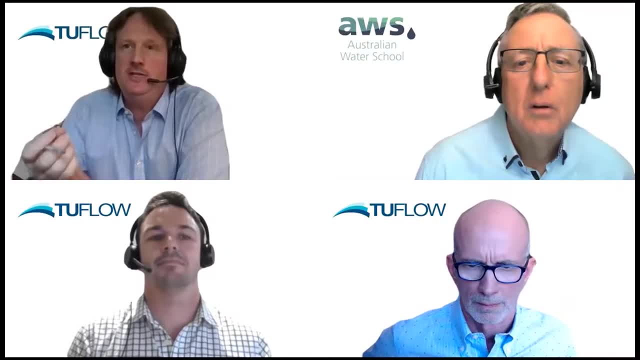 because it can't stay dry unless there's yeah. So as soon as you start applying rainfall, all of those cells become wet, And I think one of the cons to the direct rainfall method was that you do need to set, essentially, a mapping depth. 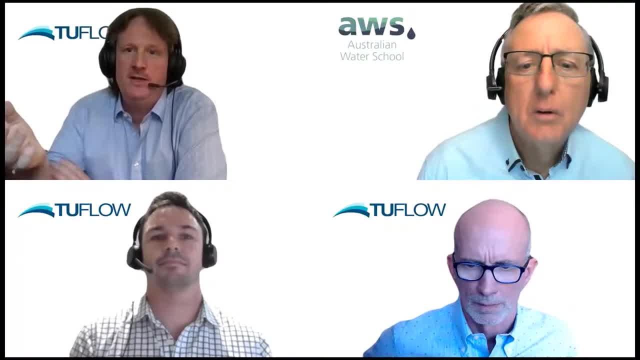 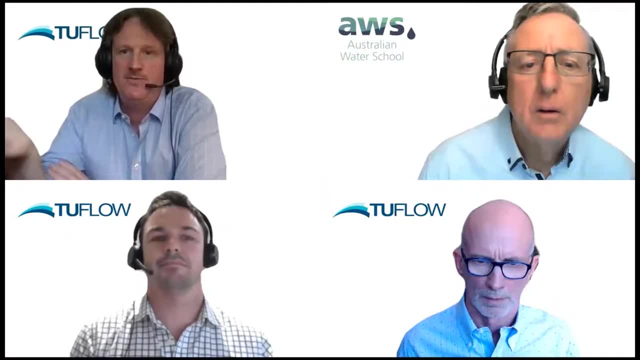 what's considered wet for your mapping. You might have 0.2 of a millimeter of rainfall sitting in a cell, but you might not want to show that as actually wet in your mapping. So essentially, yeah, applying rainfall to a dry cell will make it wet. 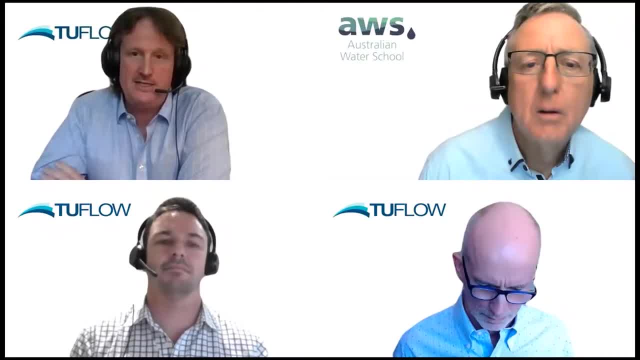 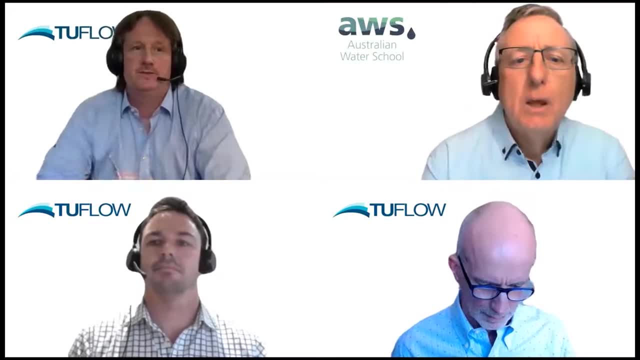 The user sort of has some options there as to how they present that in terms of what's considered wet and dry for mapping, which is probably different to what's considered wet and dry hydraulically. Jeff asks: can someone please reiterate why depth varying manning didn't prove particularly useful? 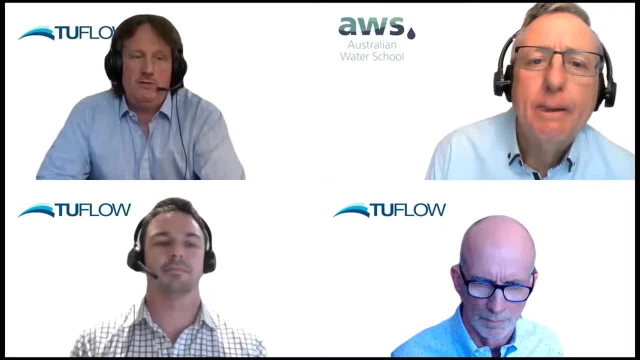 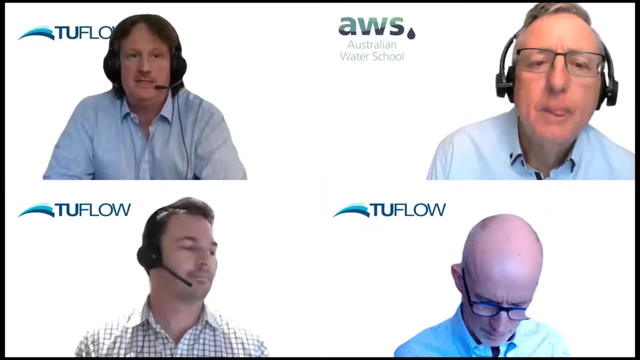 I mean, I think it depended on the case. I think that when we were running that with the depth, the first test case, which was a Throsby case, it certainly did prove to be quite useful in terms of matching the shape of that. 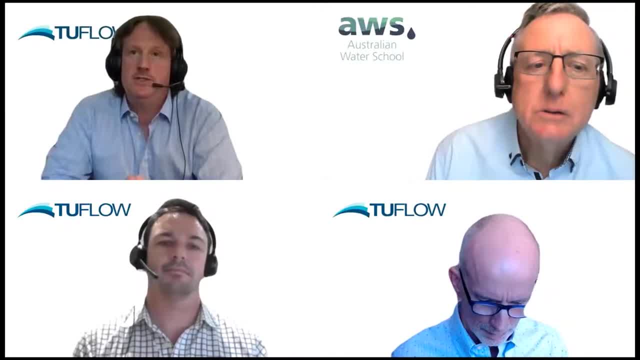 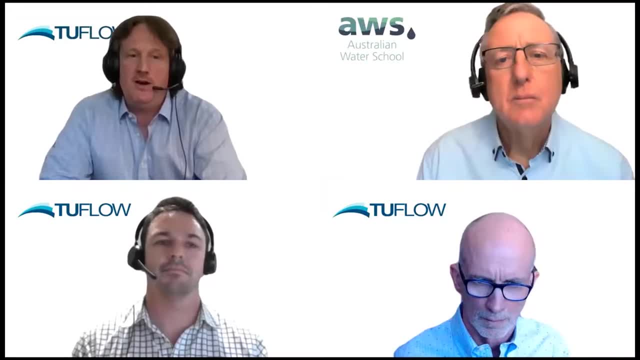 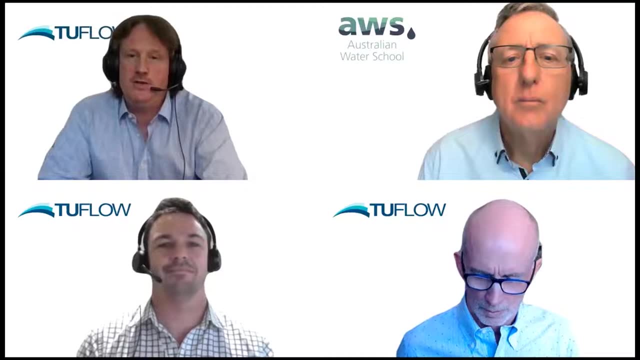 For the second- sorry, the third- test case, which was the Welsh model, the depth varying mannings probably didn't prove that useful, because I don't think it's a surface runoff problem entirely, in that I think that there's a lot of interflow going on. 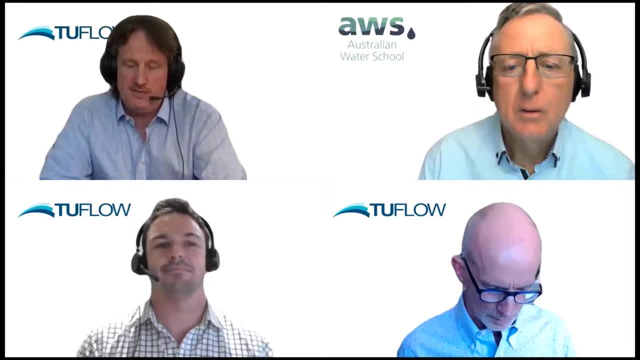 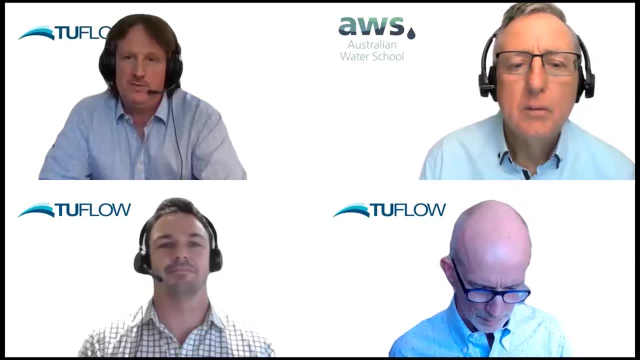 in that model, probably due to the low rainfalls and high soil porosity. So I think that just using mannings to calibrate, we ended up with a high mannings value. whether we used a depth varying mannings or not, we still had to have quite a high mannings value. 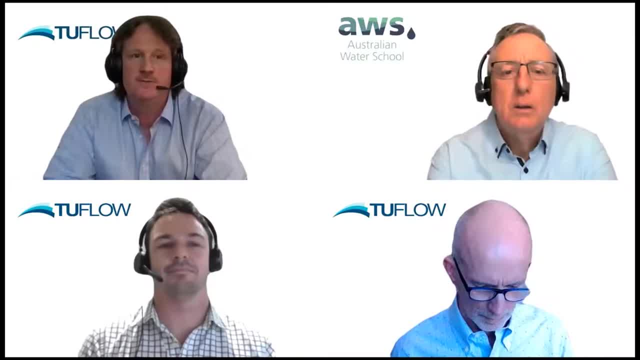 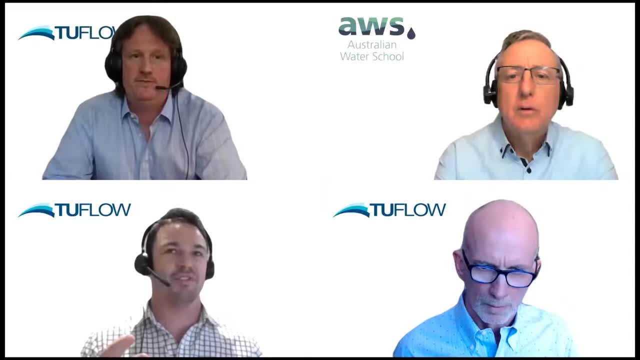 to calibrate that if we weren't accounting for interflow. Can I just add to that There's been a few questions along that same line of thinking. When it comes to modelling, it's always important to remember that what we're trying to do 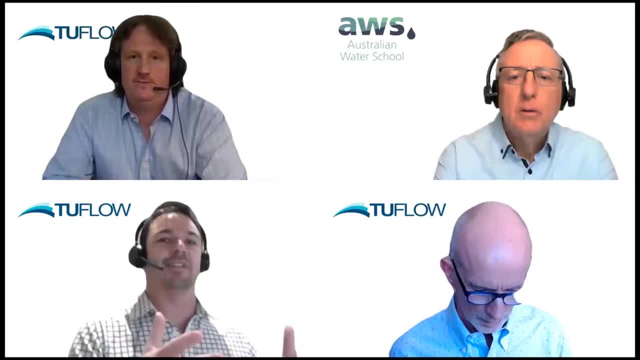 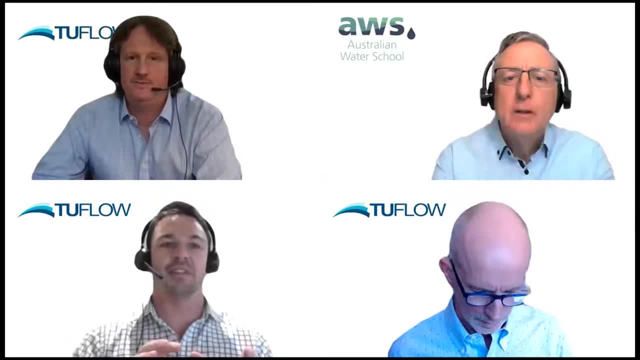 is replicate what's happening in reality in a computer. Now, if the dominant forcing of the flood behaviour is that interflow behaviour, then you need to represent it in the model for it to produce an accurate result, Or alternatively, if that's not a dominant parameter, 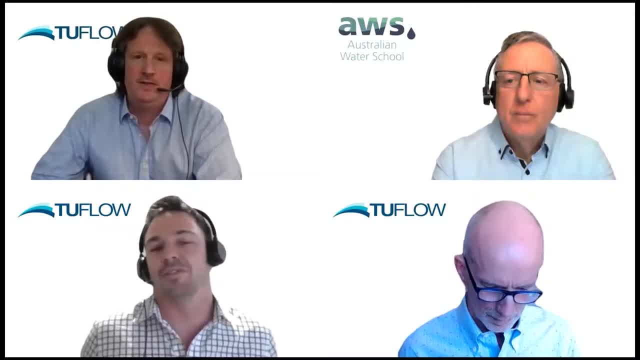 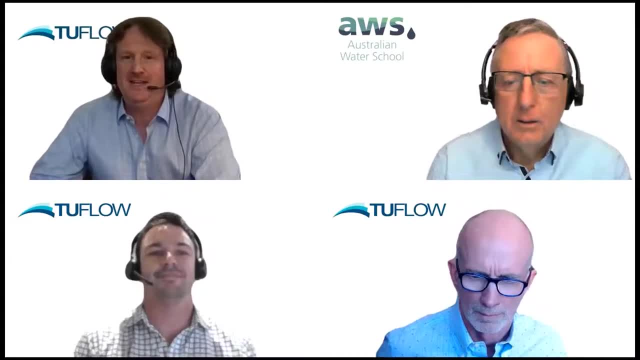 then it doesn't come into play And every single catchment is unique in that way. And probably what we're more used to in Eastern Australia is high rainfall intensities and probably clayey soils, where that subsurface flow for flood behaviour is probably not so important. 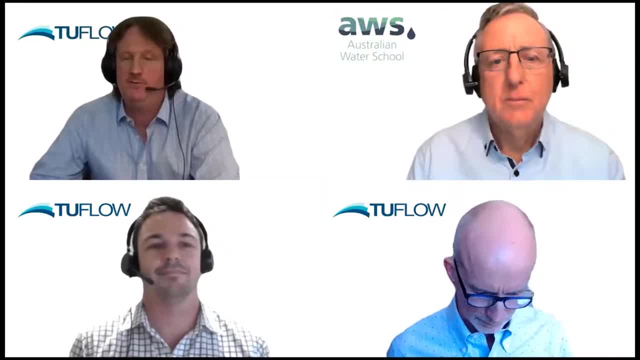 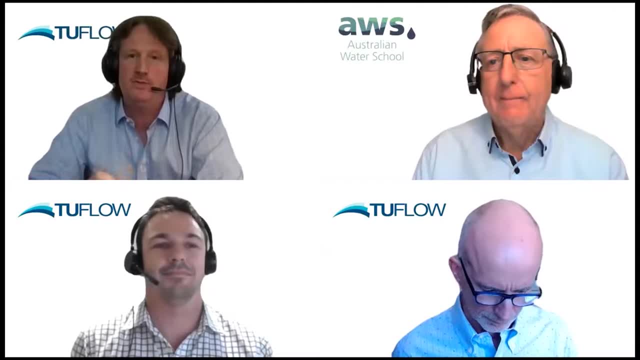 If you're looking at longer term simulations, that certainly will become important. But if you've got 100 millimetres of rainfall in an hour, that slower mechanism is probably not as important for that peak flows. I think we're going to have to make this. 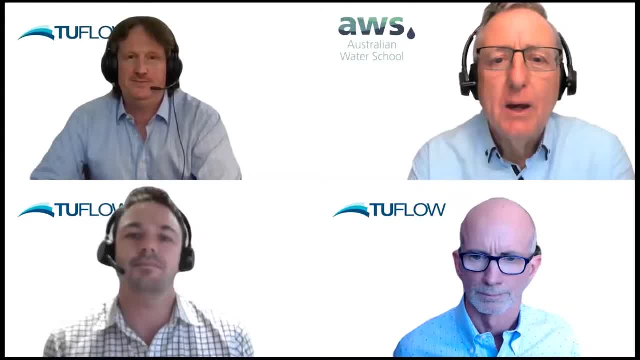 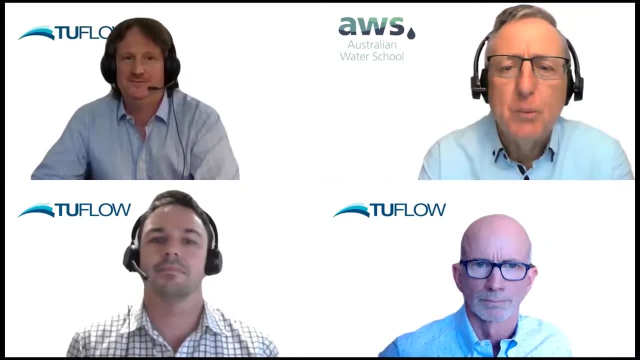 our last question. everyone, It's been a terrific time. This is from an anonymous attendee. How does the two-flow model 2D model resolve the transfer of vertical momentum when using the direct rainfall on steep terrains? Would the error resulting from these be insignificant? 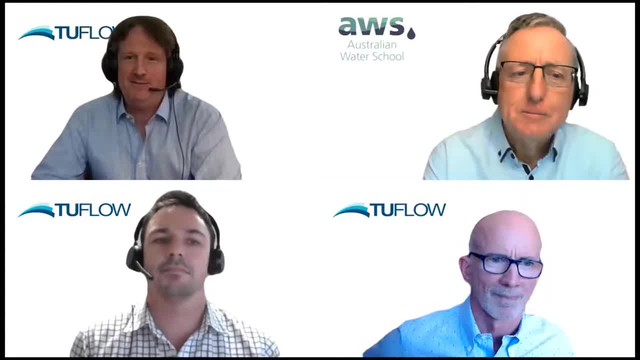 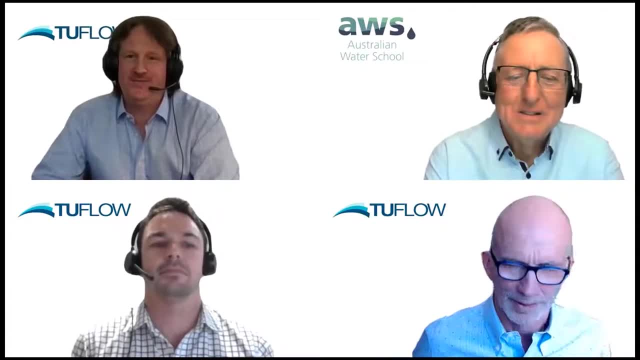 Any tips and cautions on dealing with them. This sounds like a very good question. It sounds like a very good build question. Yeah, it's a good question, Typically, unless you've got a cliff face or something like that- the steep terrains that we're dealing with. with most catchments, don't really have this problem. It's not like the problem you have with a spillway from a dam, where the vertical acceleration is really important And none of the 2D or even the 3D layered schemes are really suitable for that. 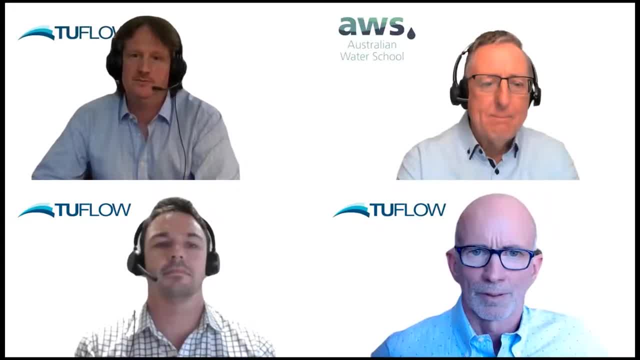 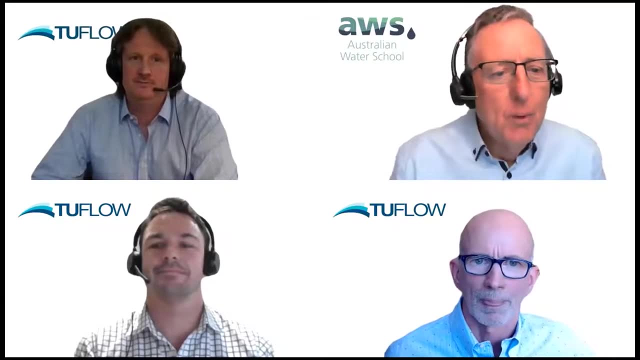 You have to move into CFD, well, So the errors from not having that vertical momentum, in my view, would be totally insignificant for nearly all our catchments, except for maybe cliff faces and waterfalls and things like that. Well, I think we're going to have to leave it there. 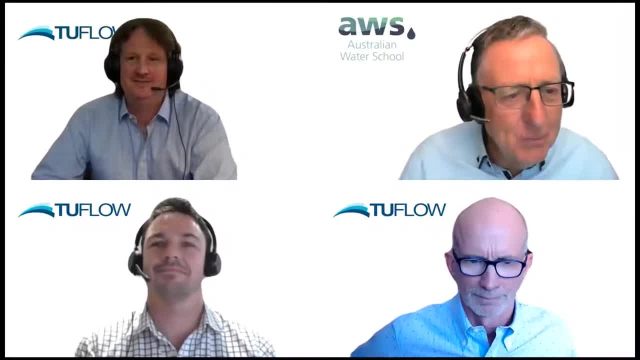 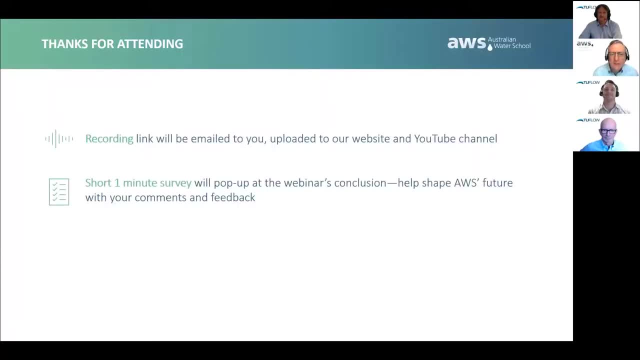 Phil, Chris, Bill. it's been an absolute pleasure listening and watching and seeing the interest, And there's still hundreds and hundreds of people online with us as we speak, And that's a good indication of just how important this is. It's just great to see people of note in the industry. 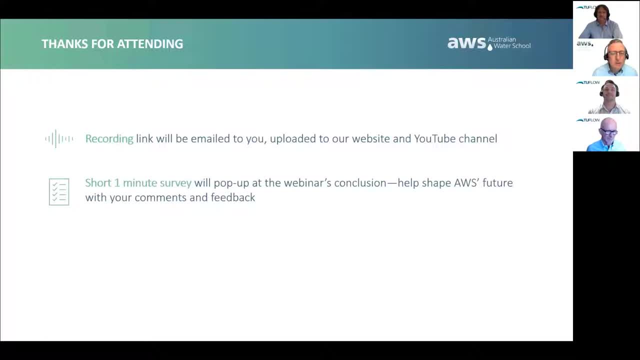 coming on board And these webinars and wonderful to have you all together with us today. again, I want to say thank you to the Australian Water School team as well: Joel Waltman, Jessica Burgess- It's so great having them work these webinars. 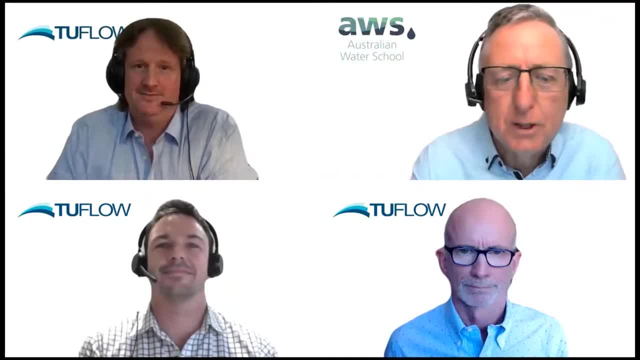 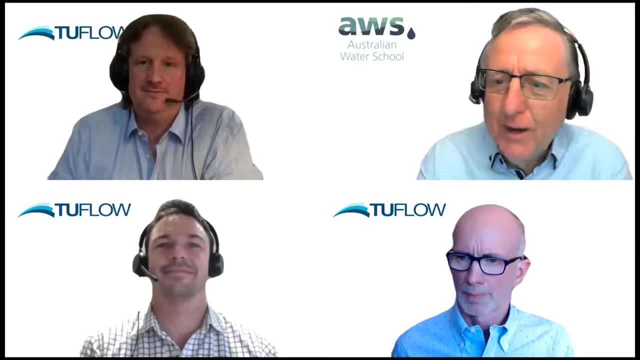 for the water industry. It's highly useful. So thank you to Joel and Jess and the team there at Water Research Australia who support the Australian Water School. I think that's it for today. Any final closing comments? Philip, Chris Bill. 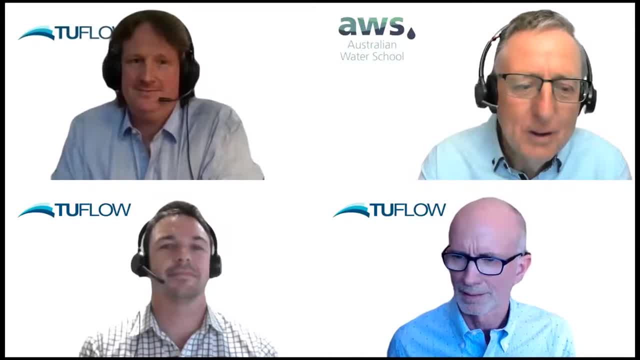 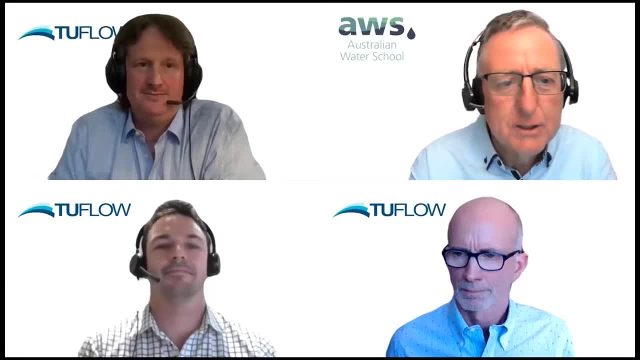 Trevor, I think the remaining unanswered questions we'll try to answer. I think that's a normal process. That will be. It'll be fantastic And we will make that part of send out to attendees if they'd like to see that. You know, the only thing I'd like to say: yeah. 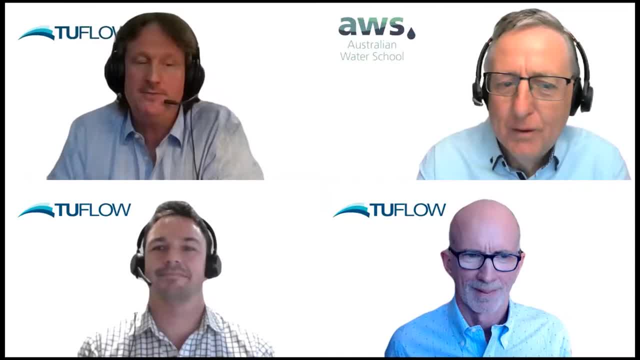 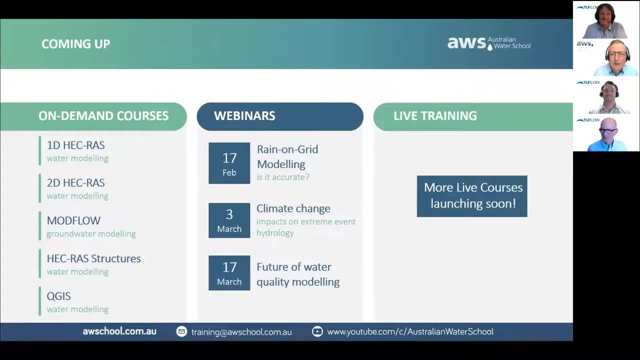 thanks everyone for joining in Wonderful. It's been great to have such a good turnout. And thank you, Phil, It's been great, It's been really good. It's been a very fun. Phil has done this. He's three kids under five and there's a couple. 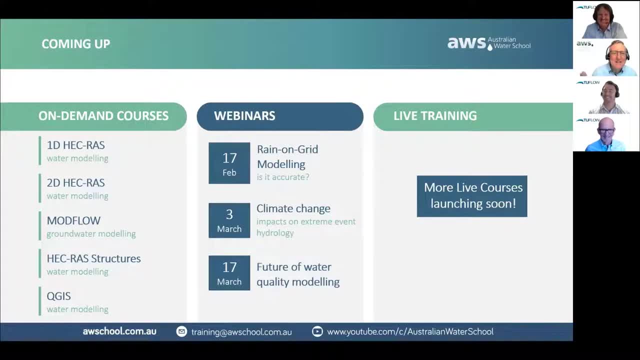 on his knee most days. How does he? You don't sleep, Philip. with that many people in your household, We're all being absolutely amazed. Done well, Phil. Done really well. I want to remind you also- you're seeing the screen there. 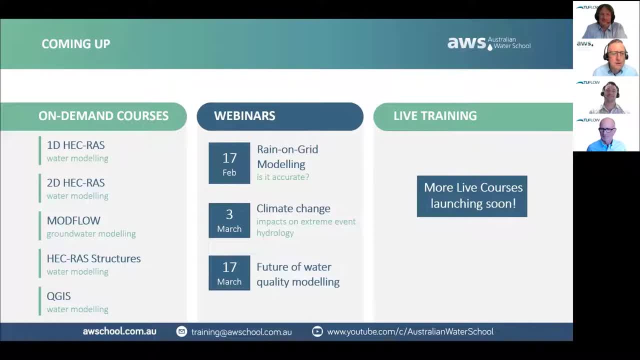 on-demand courses, webinars and live training. Just go onto the website, the Australian Water School website, and you can pick all that up there. It's a fantastic array of water industry webinars, training and courses. So once again, thanks a lot, Phil. 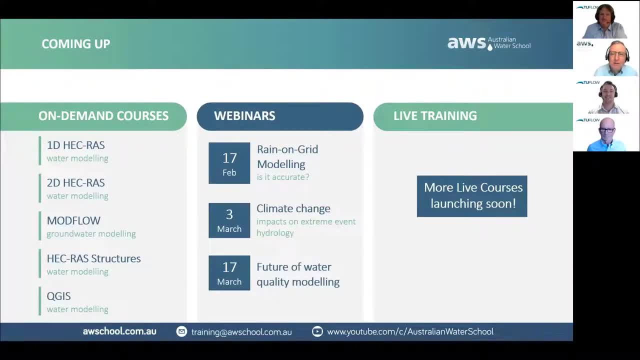 Thanks Chris, Thanks Bill, Thanks everyone for joining us and making this such a terrific time. I'll stop because I can see the messages coming in from lots of people. Yeah, it's a fantastic presentation. Thanks everybody.